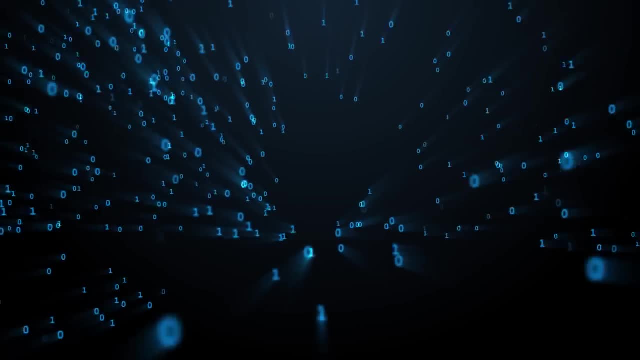 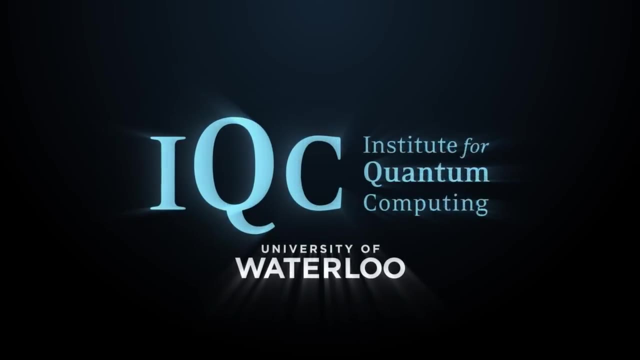 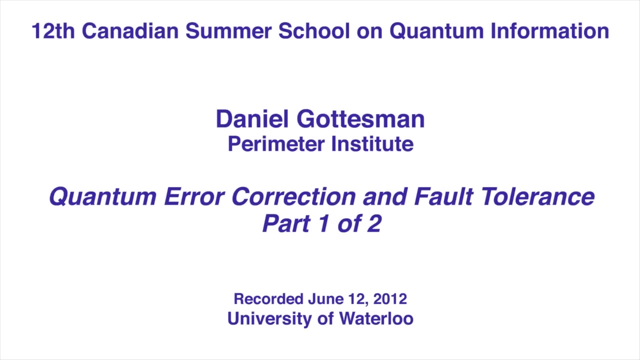 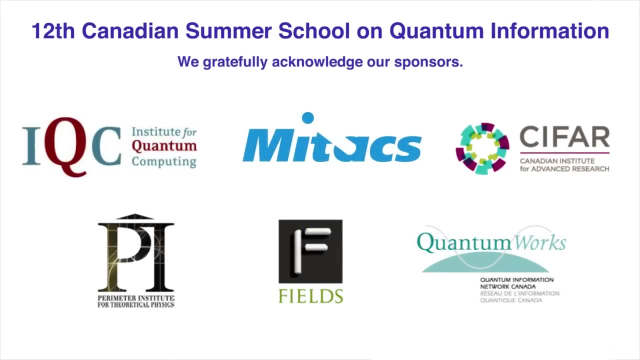 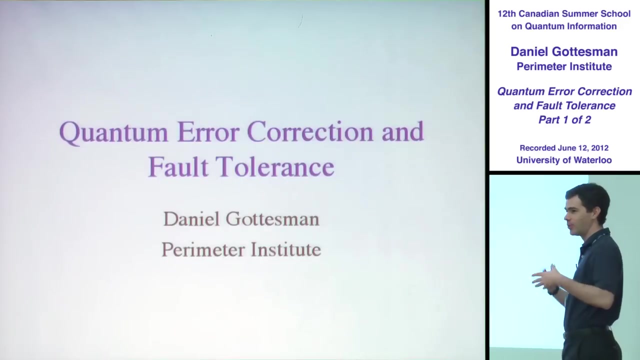 I guess you've heard some already about implementations, So maybe that gave you a little bit of appreciation for the fact that building a quantum computer is not very easy and that you can't really expect that every individual gate or every individual qubit is going to be doing exactly what you want it to do. 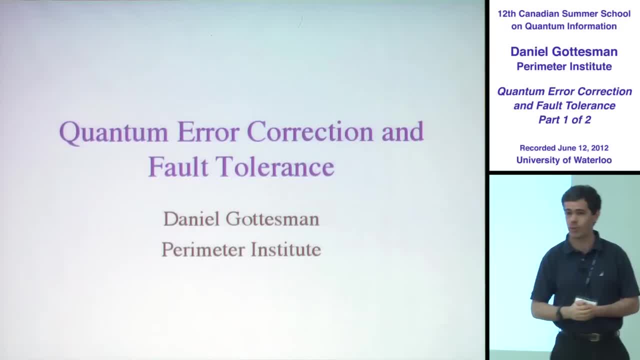 And so that's where quantum error correction and fault-tolerant quantum computation step in. The idea there is: we'd like to build a quantum computer in the presence of noise, and we still want to get the right answer at the end, of course. otherwise there wouldn't be. 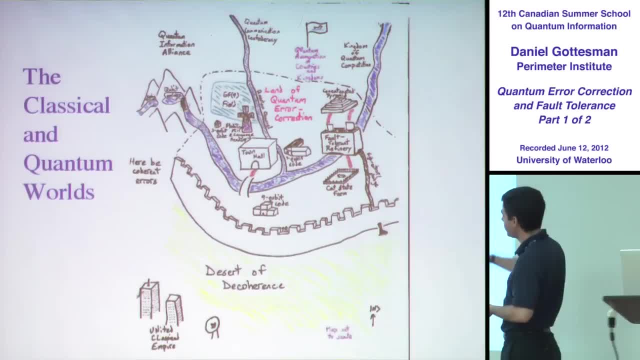 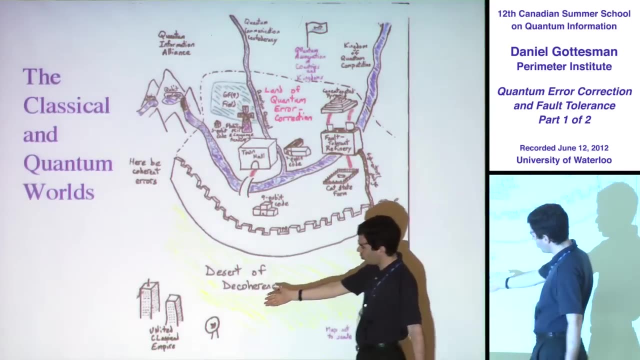 much point, Okay, so first. well, so this hour and the next one after lunch are going to give you kind of an overview of quantum error correction, And here's maybe the big picture. So down here in the lower left corner of this picture is a map. I guess is a really better. 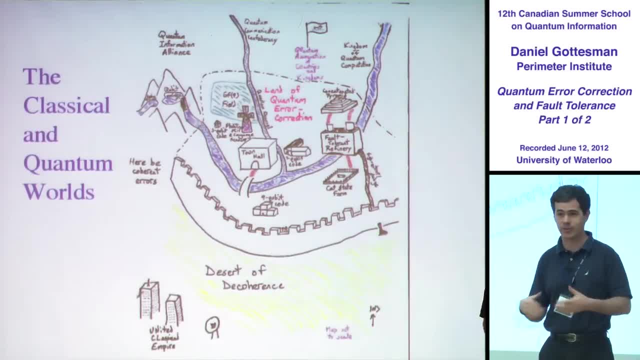 word for it is where we live in everyday life. It's the classical world, with skyscrapers and satellites, There's a lot of light dishes and things like that, And then the quantum world is taking up the bulk of the map, and that has been the sort. 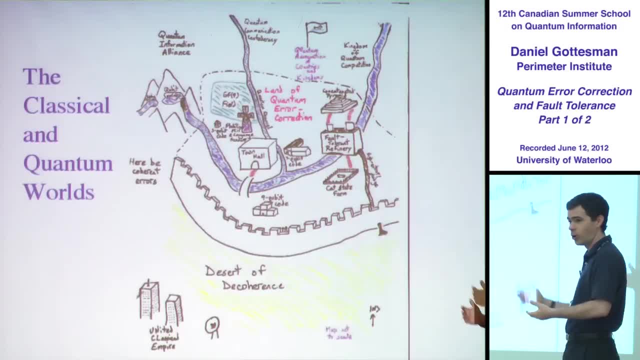 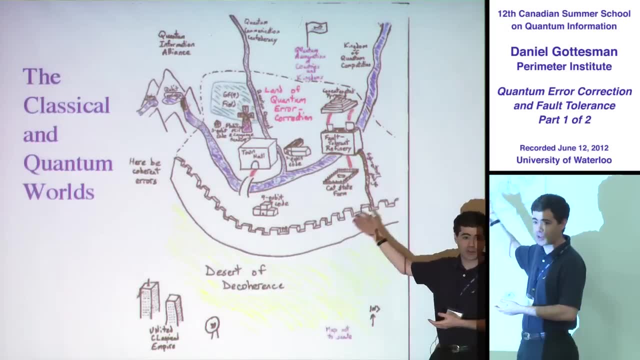 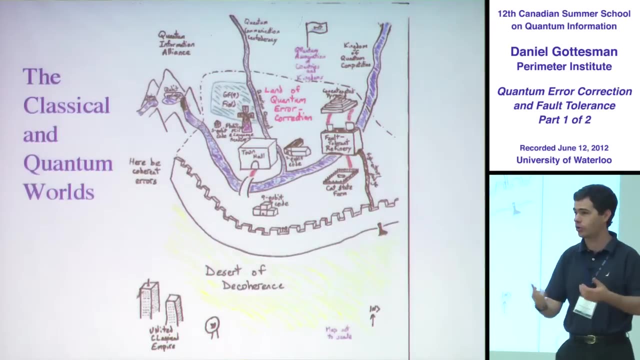 of amazing stuff. you've been hearing about quantum algorithms, later quantum cryptography, quantum communication, things like that. But the quantum world and the classical world are separated by this vast desert of decoherence, And any quantum thing that tries to interact with the rest of the world gets very rapidly. 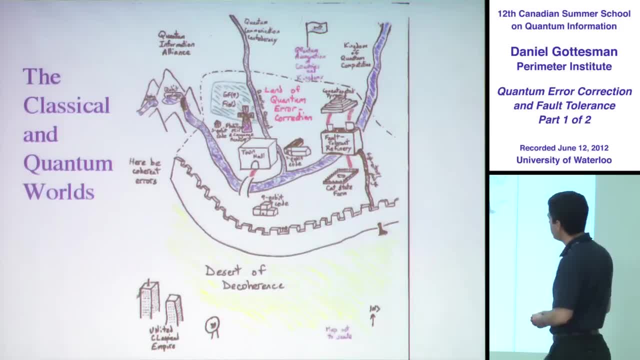 decohered and becomes- It's just classical again. And so the sands of this desert are very corrosive to quantum things, And so the purpose of quantum error correction is to build a protective wall around the land of quantum computation in order to protect all the quantum wonders that you have been. 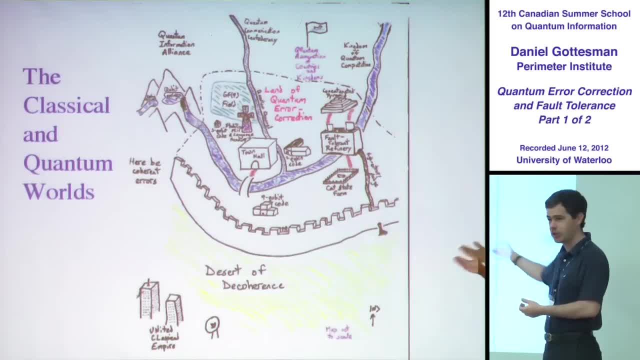 and will continue to hear about this week from the depredations of the sands. And so there's a variety of sites to see in the land of quantum error correction and I'll give you kind of an overview of some of them over the next two hours. 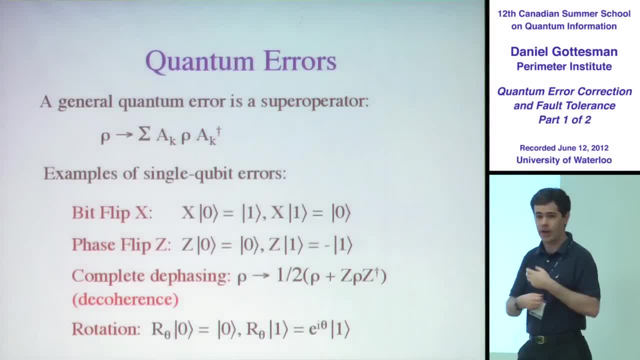 So, to get started, let's think a little bit more carefully about what an error is for a quantum computer and what kinds of errors we're going to try to correct. So the most general thing that can happen to a single qubit is a completely positive. 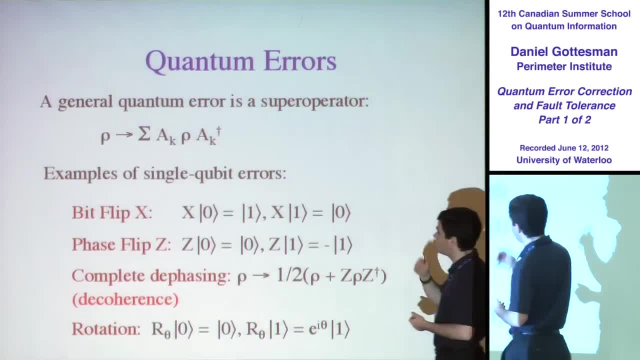 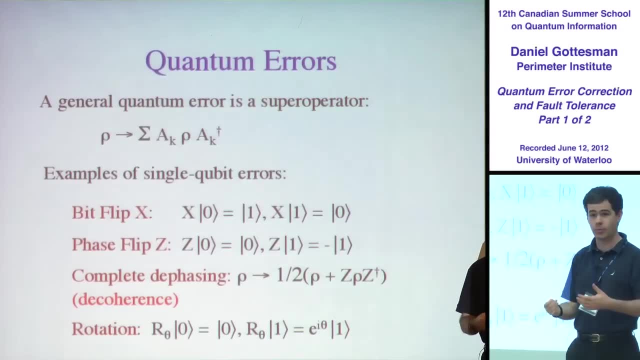 map, a super operator which will have the effect of mapping the density matrix rho to some sum over a A k rho, a k dagger. If you prefer to think in terms of Hilbert space vectors, kets, then you can think of. 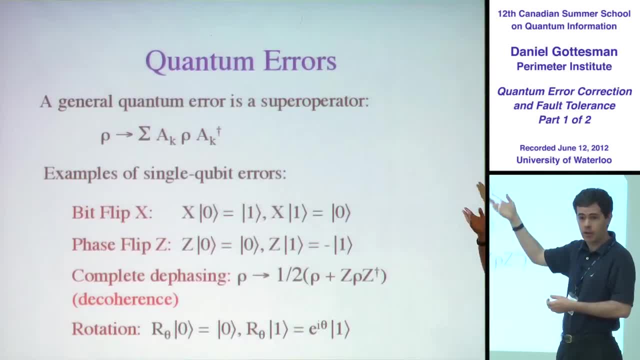 this as just having some matrix a k that occurs with some probability And on a single qubit. well, the matrix is just going to be a two-by-two matrix. I should say that these individual matrices a k don't have to be unitary. 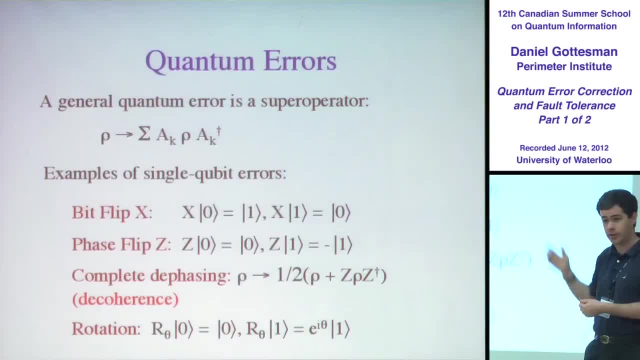 There's a condition on super operator: that sum of a k dagger a k is equal to the identity. So they have to all kind of together sum up to one and that makes probability conserved. But individually they don't have to be unitary. 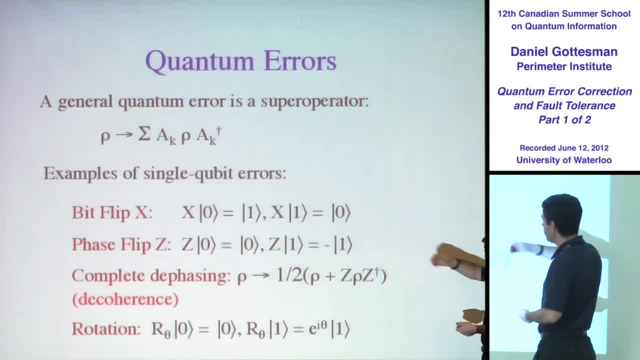 But you know, sometimes there will be a unitary error. It's actually a bit flip. So a bit flip is kind of what you think about. classically, when you think about an error, It takes zero to one and one to zero. 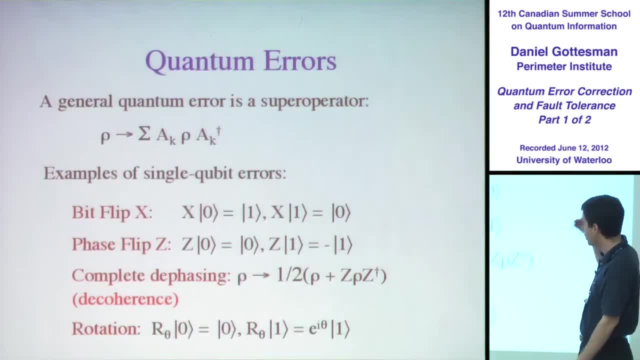 But of course this is a quantum error. so if you have a superposition alpha zero plus beta one, the bit flip still has to do something to it, and what it does is it takes alpha zero plus beta one to alpha one. 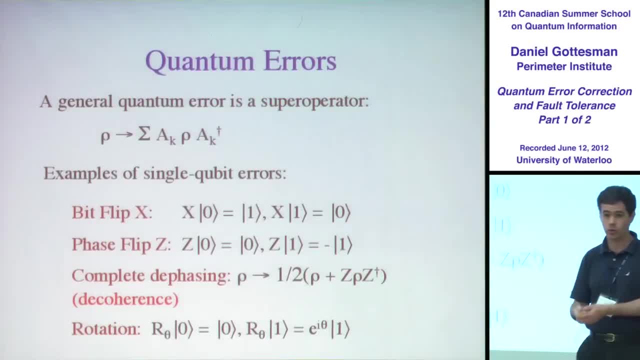 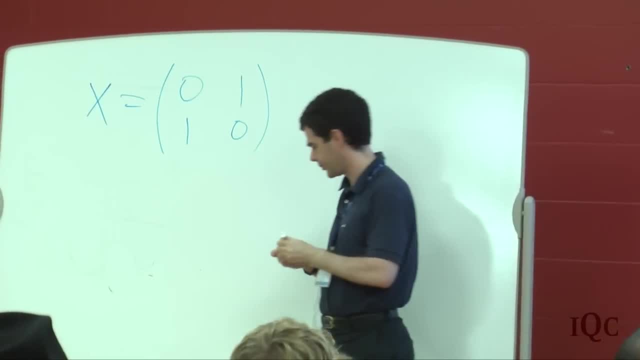 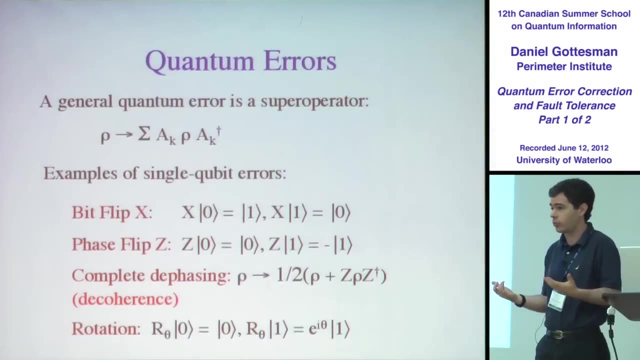 That's the effect of a bit flip. You can write that as a two-by-two matrix like this. Okay, but there's other kinds of errors that can afflict a quantum computer as well. So, for instance, phases are very important, right. 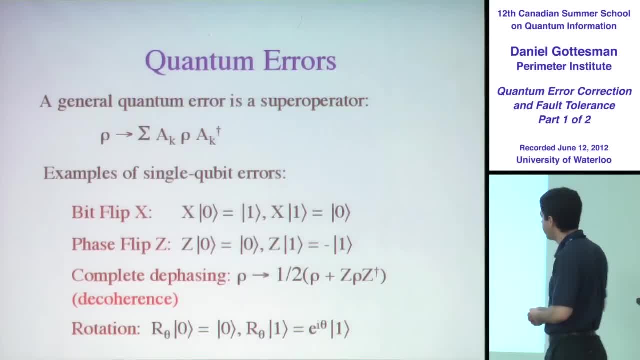 That's kind of what distinguishes quantum states from classical states, And so we have to worry about phase errors. So phase error would be written as a z matrix. here It's the same, as It's the poly sigma z, which takes zero to zero and one goes to minus one. 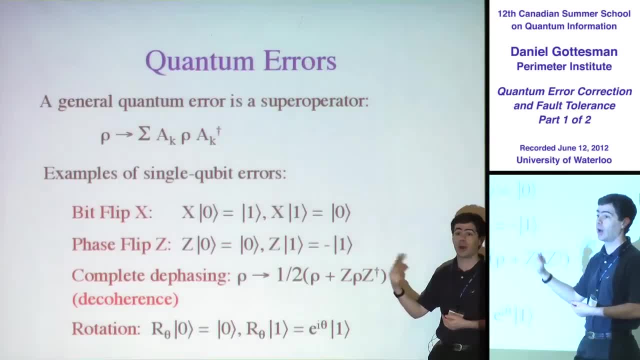 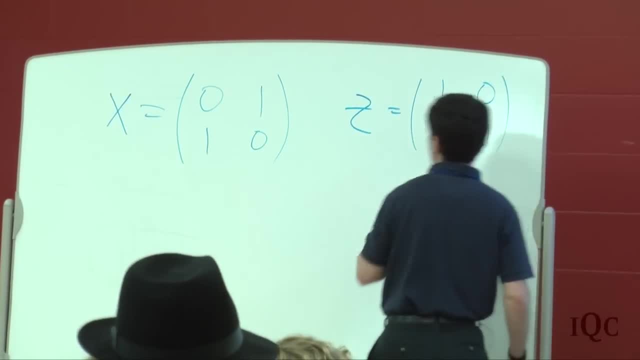 And, of course, if we have a superposition- alpha zero plus beta one- we get alpha zero minus beta one after the z error, And so then, as a matrix, z is this. Then, of course, there's a third poly matrix that we'll be dealing with later, which is: 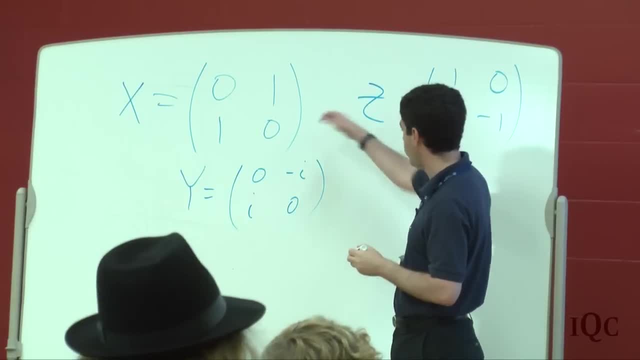 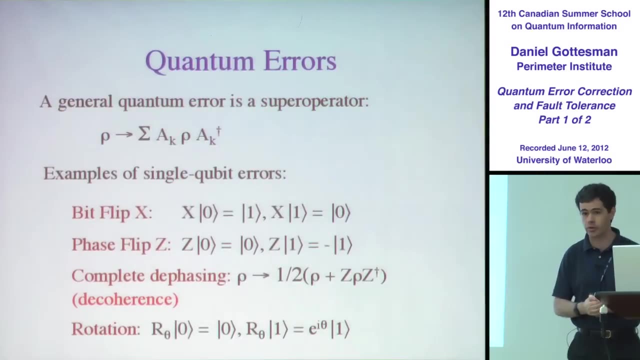 y, sigma y, and that's both a bit flip and a phase flip simultaneously. Okay, but of course unitary errors, as I said, are not. That's the only things that can occur. So, for instance, we could have a mixture of two different unitary errors. 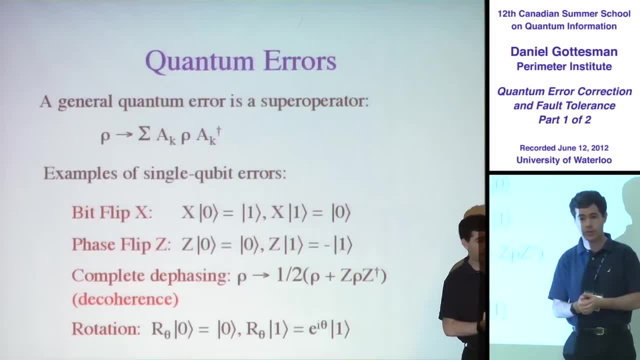 So, for instance, with probability one-half nothing could happen to the state, And with a probability one-half we could have a z error that flips the phase, And the effect of this kind of error is that the phase information is completely lost on the qubit. 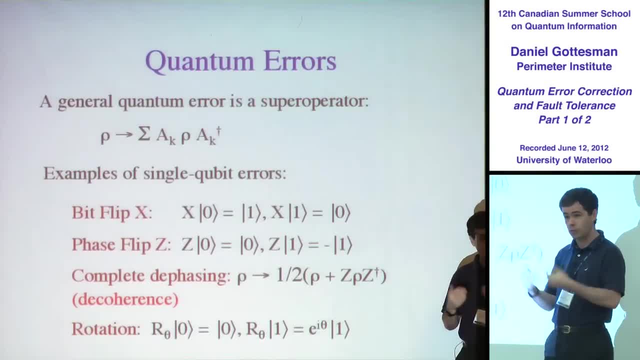 So that would be something certainly bad. We don't want that to happen because we want to preserve superpositions in our quantum computer, to take advantage of the quantumness. And then, as another example of what could go wrong, you could have a phase rotation that's different from plus one or minus one. 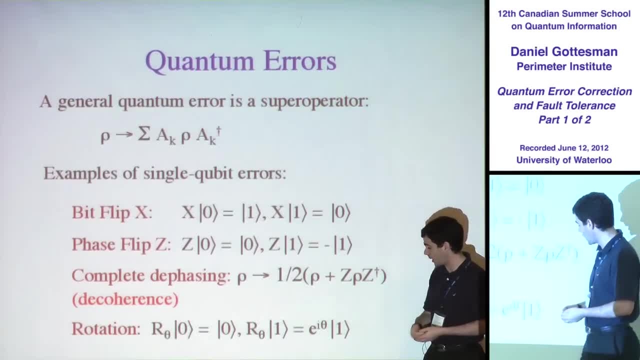 It could be really any phase. So we could have a rotation by an angle theta where zero goes to zero and one goes to e, to the i theta one, And of course these are just a few possibilities There's really, you know, any two-by-two matrix could appear here, up to scaling. 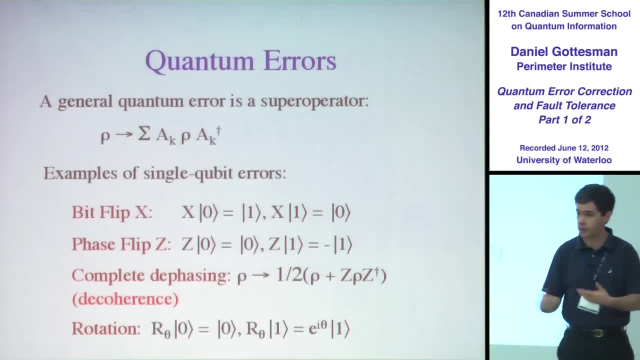 And you could also think of, you know two qubit errors, three qubit errors, et cetera, And somehow we're going to want our quantum computer to deal with this wide variety of possible errors. our quantum error correction code. 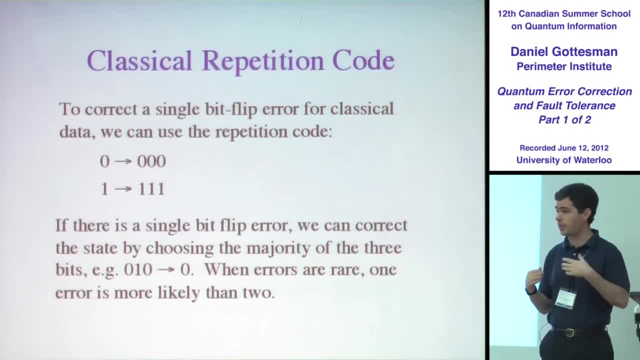 So okay, so how do we deal with this? Well, let's start by thinking of classical error correction, for inspiration. So, classical error correction. well, the first thing you think of is you think of the repetition code. Suppose we have to deal with those classical bit flip errors. 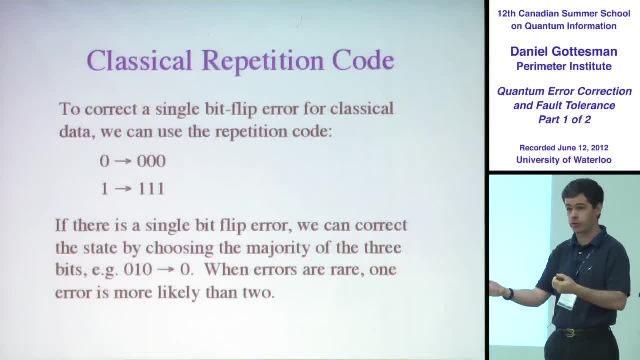 Well, what we can do is we can encode a zero as three zeros and a one as three ones. Okay, And then if one, If one bit has been flipped, we'll end up with, say, zero, one zero, And we'll be able to recognize that it was the middle bit that was flipped there. 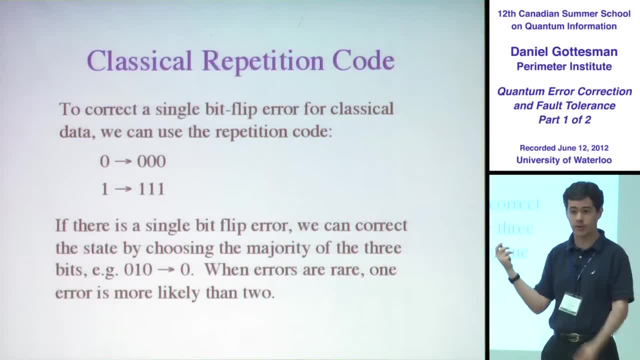 and that it originally started as zero, zero, zero, So we should decode it as a zero. Now, if each bit is getting flipped independently, then it's possible that actually two bits were flipped And that instead of starting with zero, zero, zero, we started with one one one. 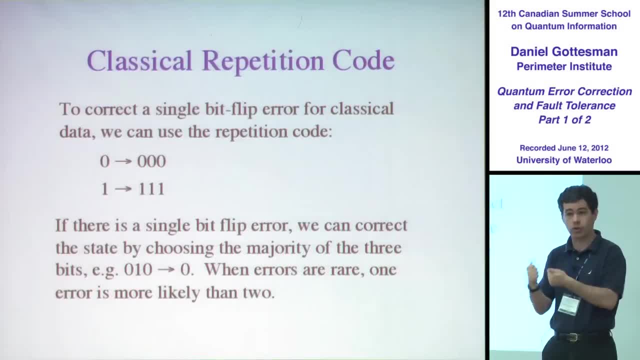 And it was the first and third bits that got flipped, And in that case our decoding will take it to the wrong thing. Okay, So this is not perfect, But if the probability of error per bit is small, then the probability of having two errors- 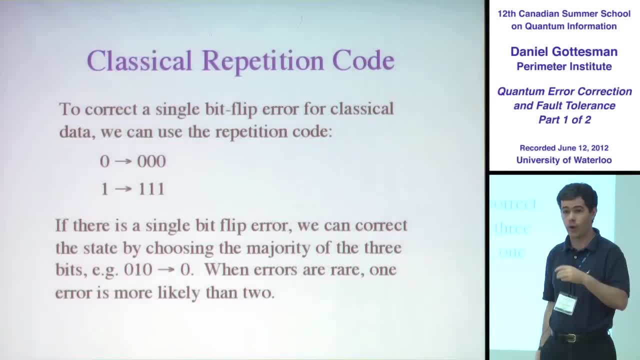 say the probability of error per bit is p, then the probability of having one error on one of the three bits is about three times p, whereas the probability of having two errors on two of the bits is about three times p. squared Okay, And if p is small, it's much more likely that we had one error than two errors. 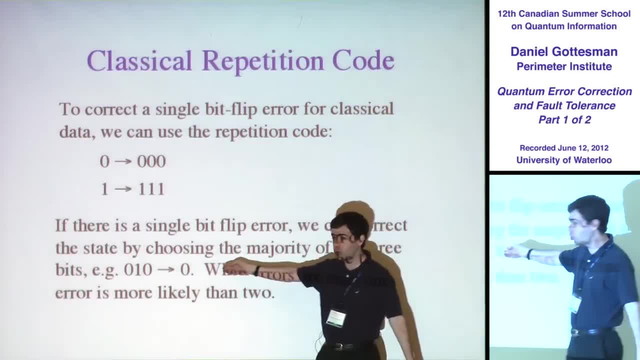 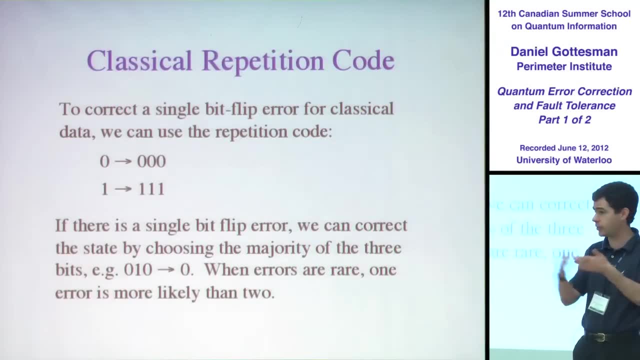 And that means That means that the probability of getting an error when we decode it is order p squared. That's what happens when there's two errors, Whereas if we hadn't encoded it at all and just sent it through this channel and had the error on it by itself. 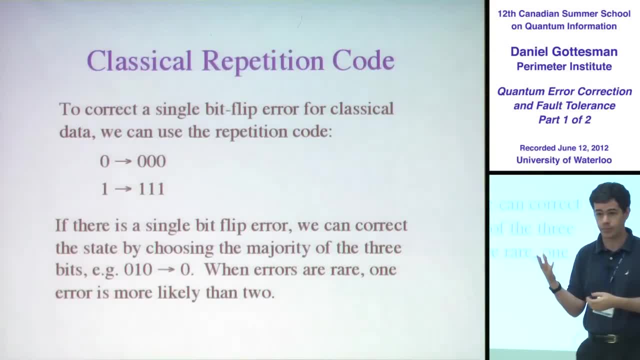 then there would have been a probability p of error. So we've made an improvement. Okay, And kind of abstracting this idea for most of the rest of the talk, I'll consider a situation that's similar, but with quantum errors, And we'll assume that there's. 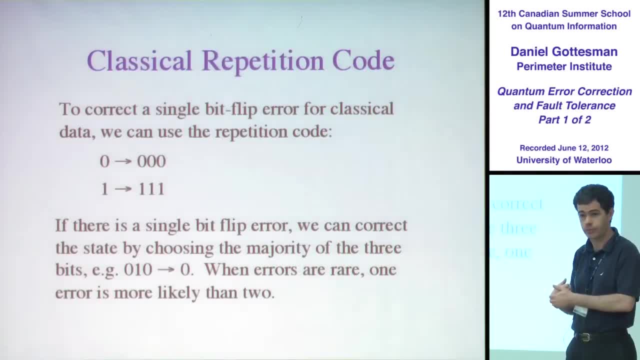 There's only one error in the code. Okay, And the logic behind this is: well, maybe the errors are occurring independently and one error is more common than two. Okay, So now this is a classical error-correcting code, and there's a big theory of classical error-correcting codes. 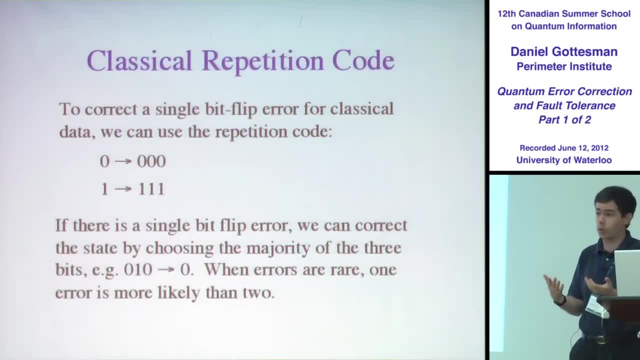 that have much more complicated codes. But we want quantum error-correcting codes. We want somebody to encode quantum states and protect against quantum errors. So what should we do? Well, thinking about this repetition code, we might try to do the same thing. 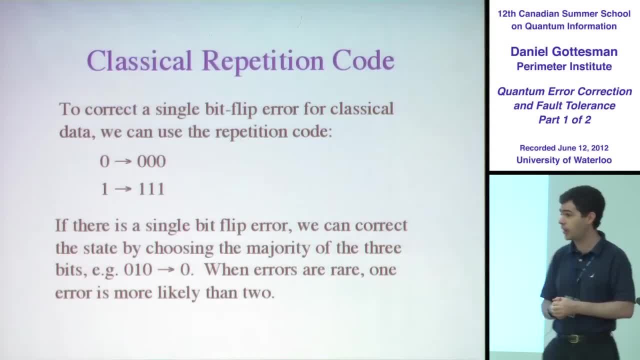 Let's make a quantum repetition code. We'll take a state psi and encode it as three copies of psi, Psi tensor, psi, tensor, psi. So what do you think of that? You can't copy right The no-cloning theorem. 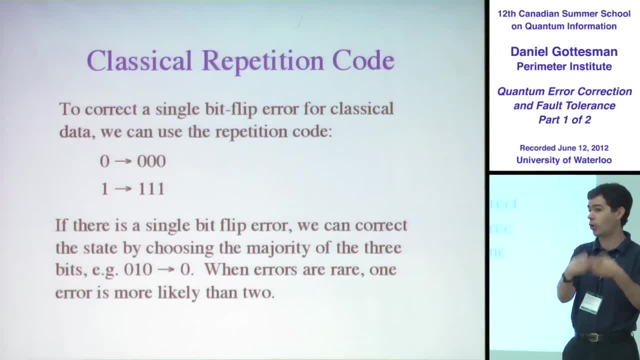 says there's no quantum operation that will take an arbitrary state psi and make two copies psi, tensor psi, let alone three copies. So that seems like a problem. The no-cloning theorem seems like a blockade in the way of doing quantum error-correction. 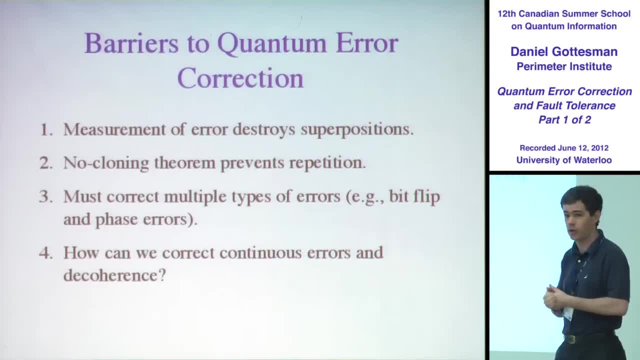 And as you think about it, you come up with more problems that quantum error-correction will somehow have to overcome, if it can exist. So, thinking back to the repetition code, how did we correct errors? Well, we looked at it and we said: 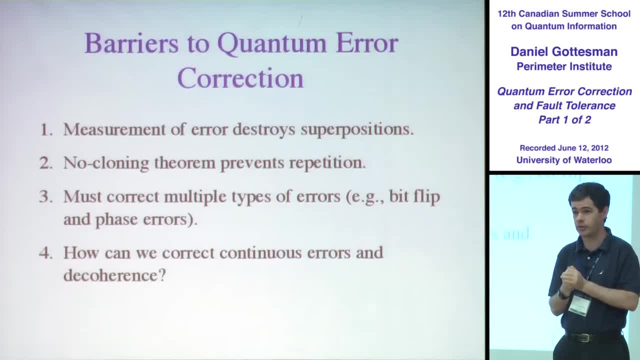 oh, the middle bit, say, is different from the other two bits. Therefore it must be the middle bit that was flipped. But when you're talking about quantum states there's a problem with that. I said you look at it. 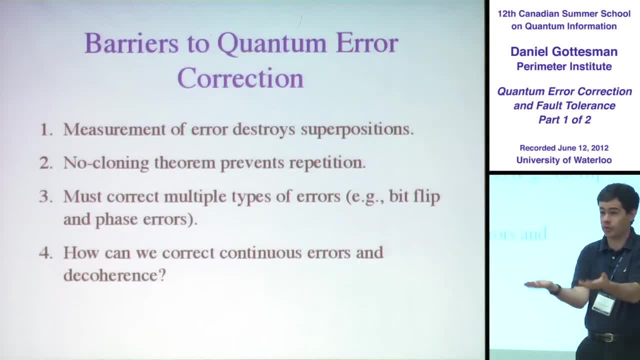 but you don't want to look at a quantum state, because that will destroy superpositions, which is exactly what we're trying to protect. Okay, So that seems like a problem. How do we measure the errors without measuring the state? Well, that's a contradiction. 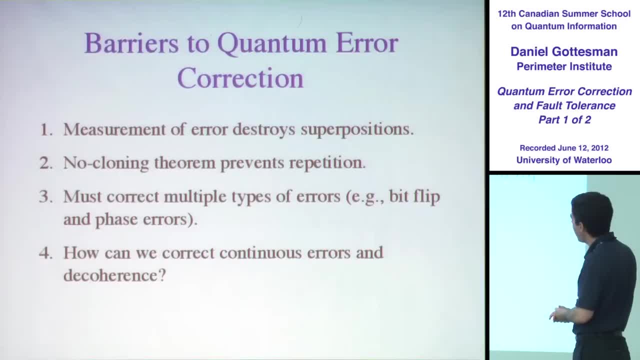 So something's going to have to give there. And then the no-cloning theorem. even if you solve those two problems well, it's still clear that quantum error-correction is going to be much more complicated. I mean, as well as correcting bit-flip errors. 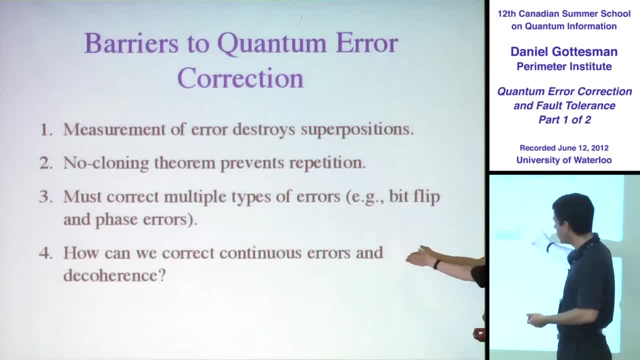 we have to correct these phase-flip errors, And then there's the continuous rotations and decoherence that involves combinations of mixtures of different kinds of errors, And somehow a quantum error-correcting code is going to have to correct all of these. 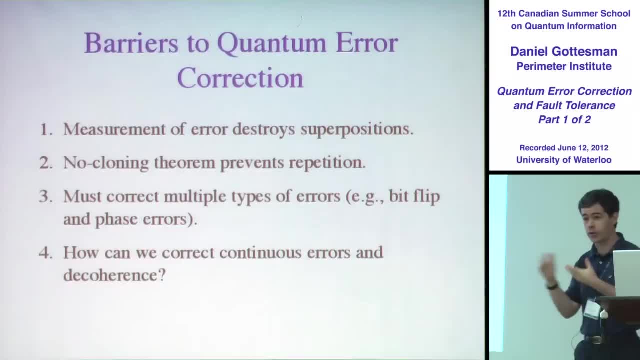 So this seems like a tall order, And at this point you might conclude: well, quantum error-correction probably doesn't work, But obviously I'm here, I have another hour and 45 minutes to talk, So there must be something there. 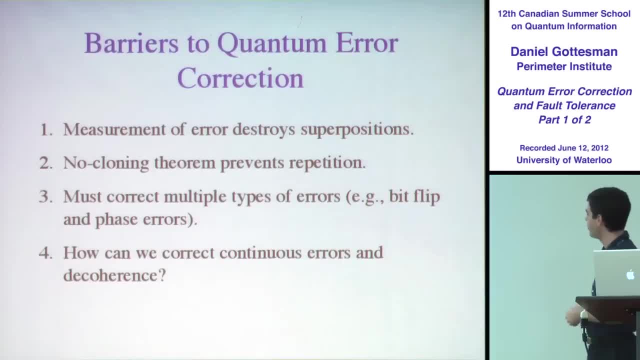 Let's start slow though. Let's just forget about trying to solve all of these errors And let's just focus on a simple situation where we have a quantum state and we want to protect it against bit-flip errors and see if we can come up with a code that will do that. 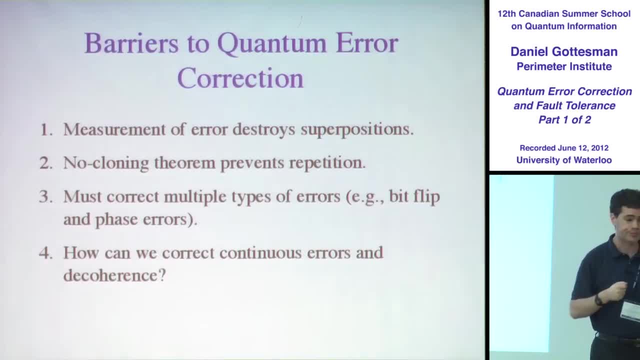 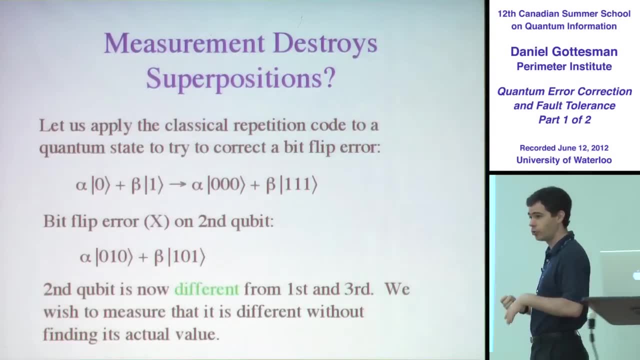 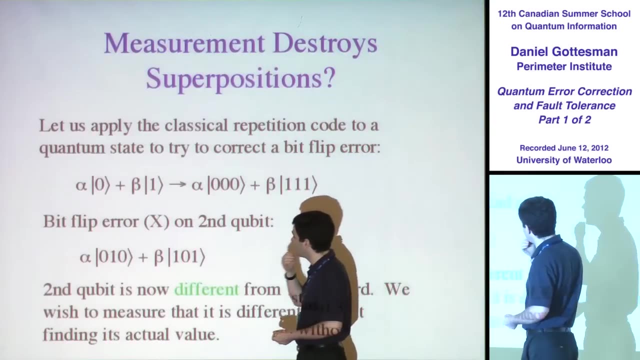 and in the process solve the first two problems. So the repetition code, classical repetition code, corrects bit-flip errors, So maybe we can make a quantum version of that. So in particular, if we encode 0 as three 0s. 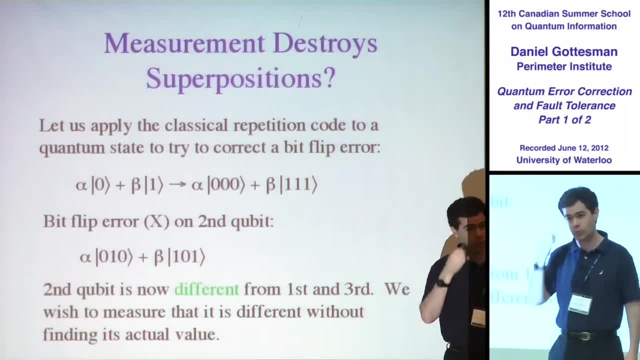 and 1 as three 1s. then by the linearity of quantum mechanics we should encode alpha 0 plus beta 1 as alpha 0, 0, 0 plus beta 1, 1, 1.. That's a perfectly valid encoding. 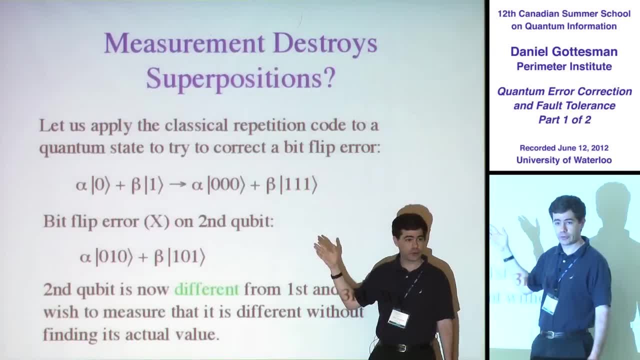 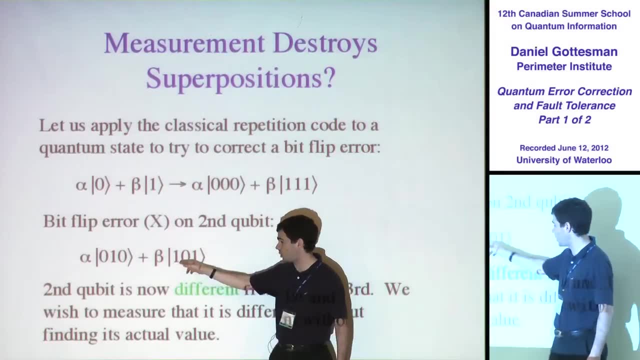 And then what happens if we have a bit-flip error on one of these qubits, say the second one. Well, instead of having alpha 0, 0, 0 plus beta 1, 1, 1,, we have alpha 0, 1, 0 plus beta 1, 1, 1.. 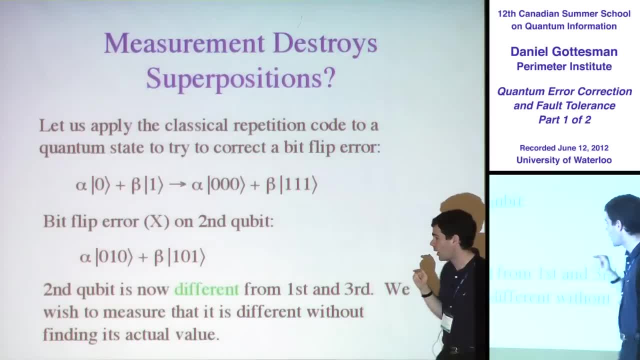 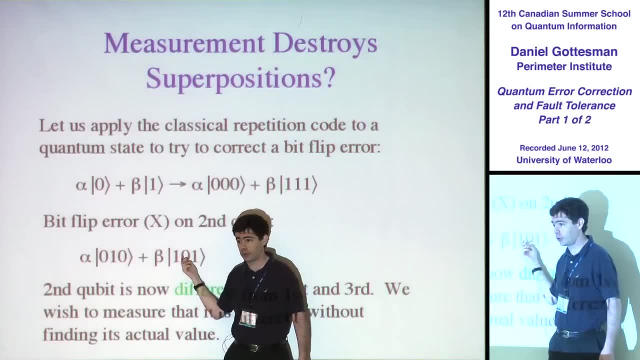 And the thing is that in both of these two kets the middle qubit is different from the first two qubits. Now, it's certainly true that we don't want to look at these three qubits to say, oh, the second qubit is 1 and the other two are 0. 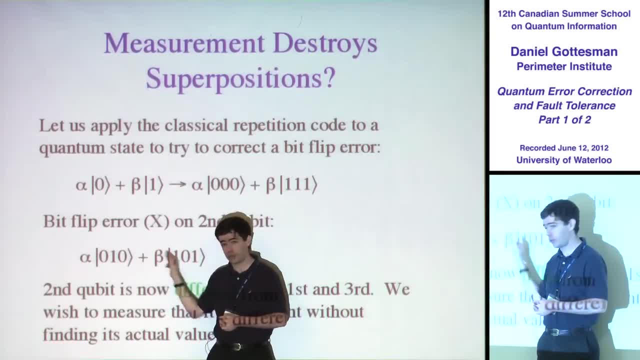 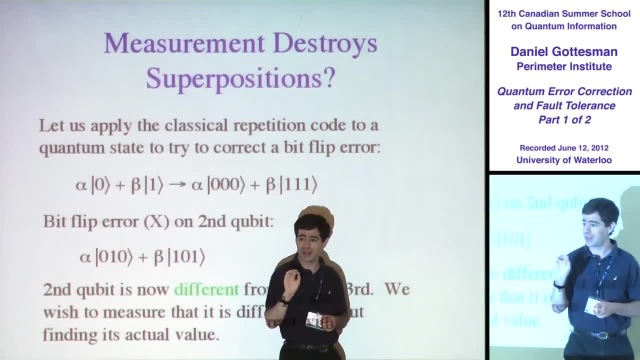 Therefore the error must be on the second qubit, because that would destroy the superposition. But if we can measure the fact that this qubit is different from the other two without measuring what it is, then that's a property. that's true for all of these states. 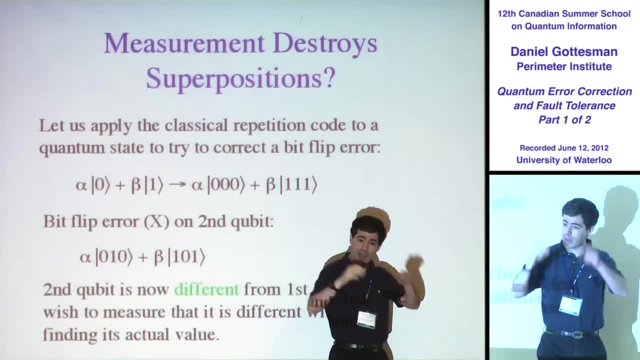 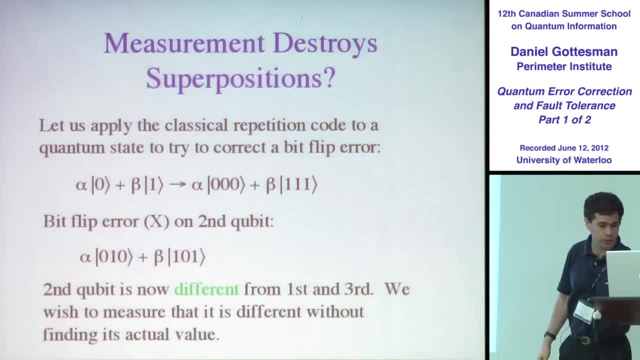 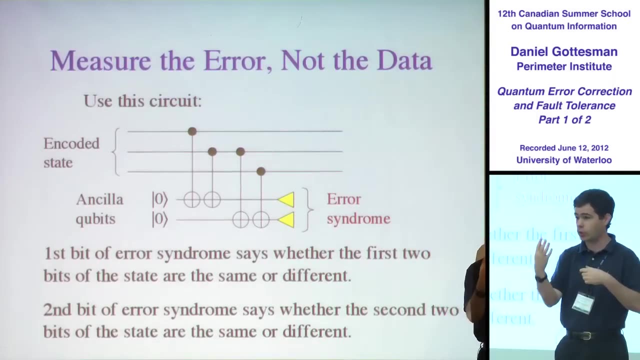 no matter what alpha and beta are, And so that's a property that we can measure without disturbing the superposition that we care about. Okay, so how would one do that? Well, let's think about it. So what we want to say is that the middle qubit 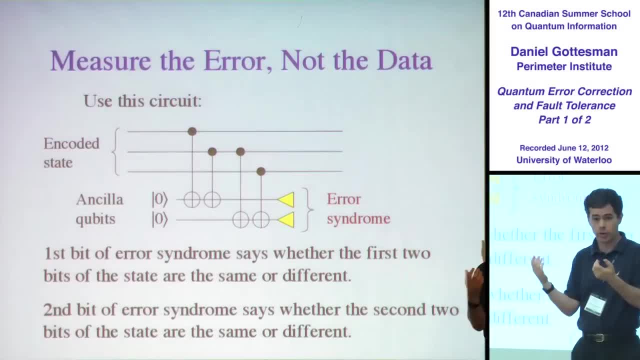 or one of the three qubits is different from the other two, In the correct state they should all be the same, And so we can break that down to saying the first two qubits are the same and the second two qubits are the same. 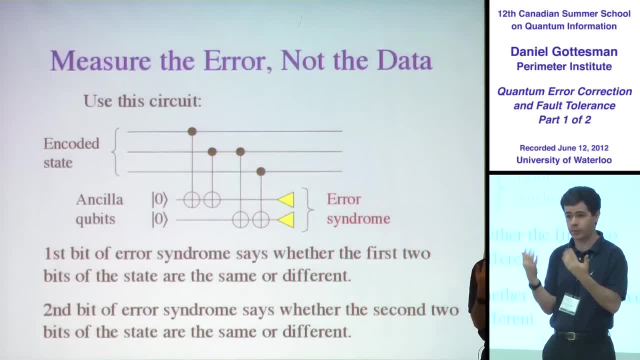 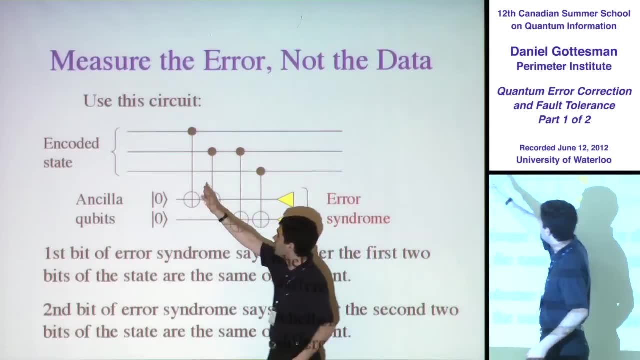 Okay, and if one of the three has been changed, then one of those two things must be wrong. So we can handle that with a little circuit like this. So we put this encoded state in and then we add two ancilla qubits. 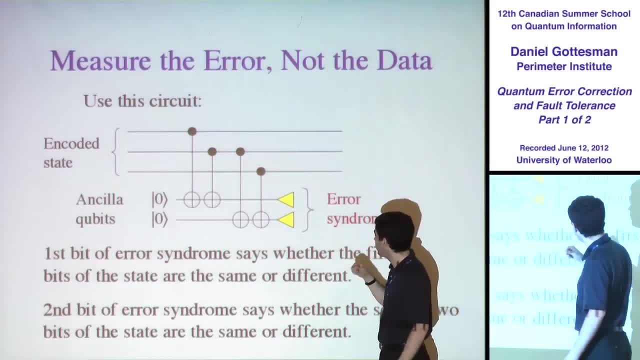 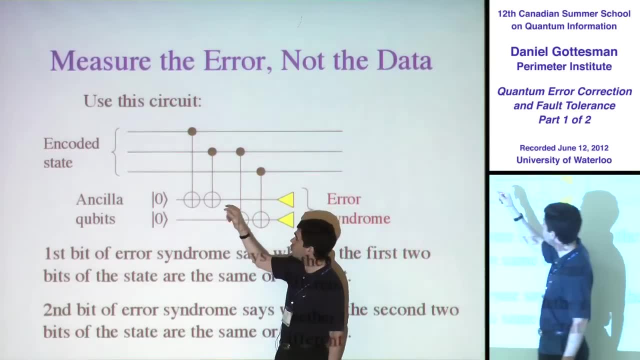 extra qubits that start in the state 0. And we're going to use these to measure what's called the error syndrome, which tells us what's going on with this error, And suppose we take the first two qubits and do control nots. 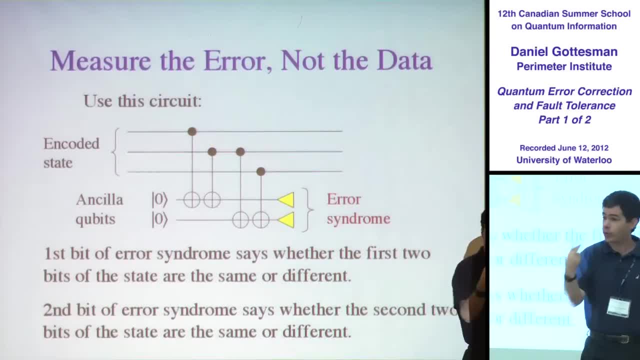 From both of them to the first ancilla qubit. Now, if both of them are 0,, then nothing happens to the ancilla. If both of them are 1,, the ancilla gets flipped twice and it ends up back at 0. 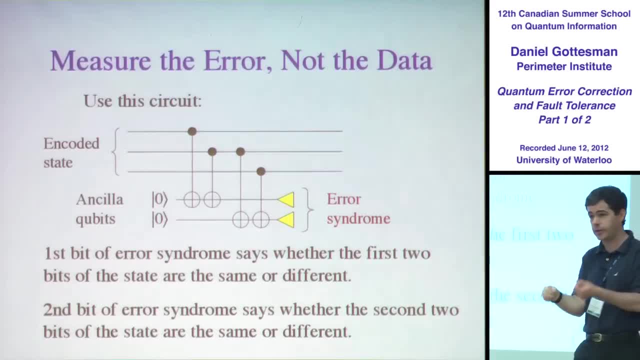 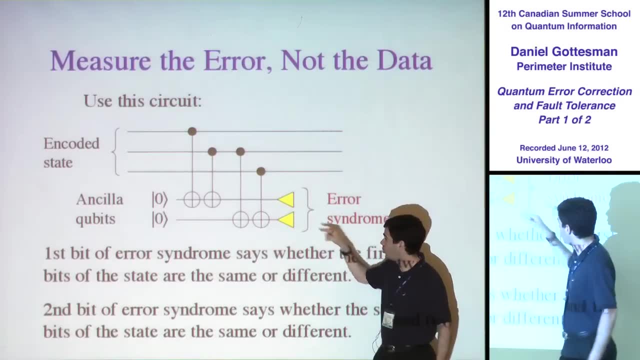 But if one of the first two qubits is 0 and one of them is 1, then this ancilla qubit gets flipped exactly once And when we measure it it ends up as a 1.. Okay, so this bit of the error syndrome. 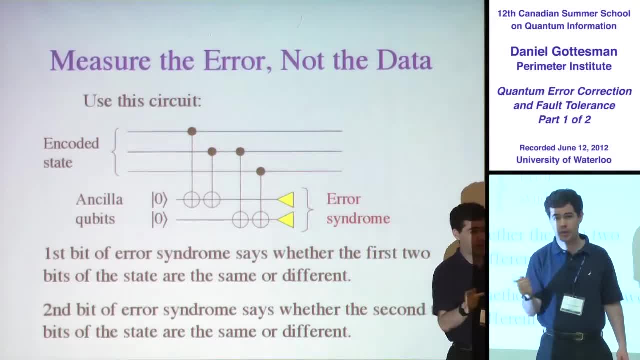 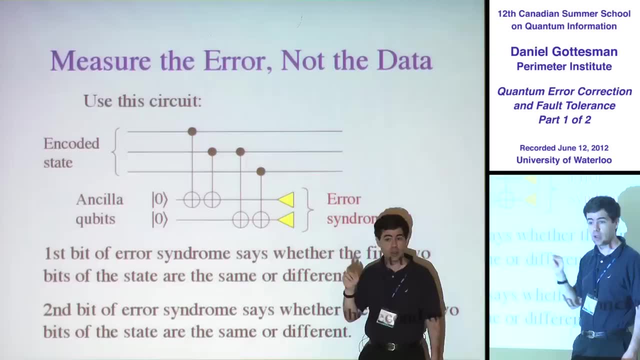 this measurement that we make tells us whether the first two qubits are the same or different And similarly we can do control nots from the second and third qubit to the second ancilla qubit to measure whether the second and third qubits. 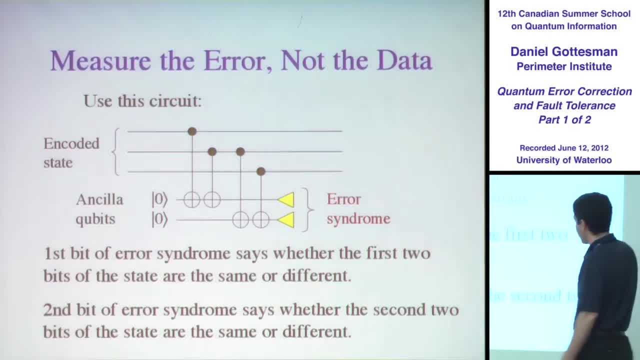 are the same or different. Okay, And so now let's imagine that case we had on the other slide where the second qubit is different from the first and third qubits. Well, what happens then? Well, the first two qubits are different. 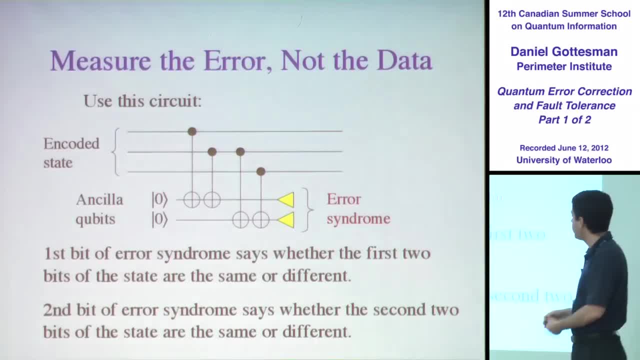 and the second and third qubits are different, And so both of these measurements will show up 1, 1.. Okay, so the error syndrome corresponding to bit flip on the second qubit is 1, 1.. Suppose we had a different error. 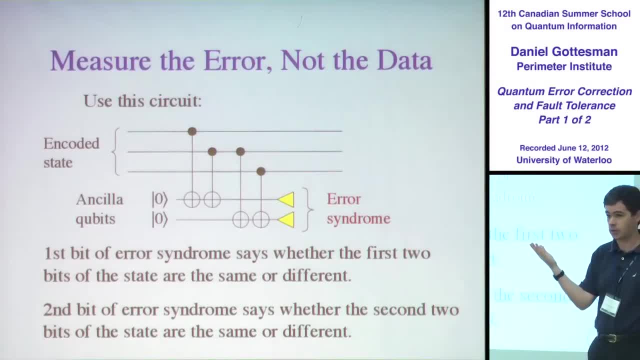 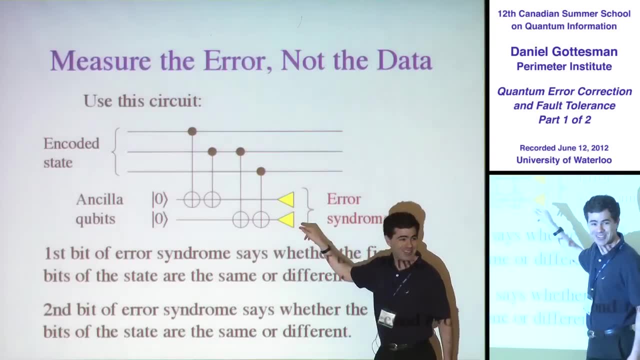 Suppose we had an error on the first qubit. What would we see then? I can't really hear, but I'm assuming somebody's saying the right thing, which is 1, 0.. Right, because the first two qubits are different: 1, 0.. 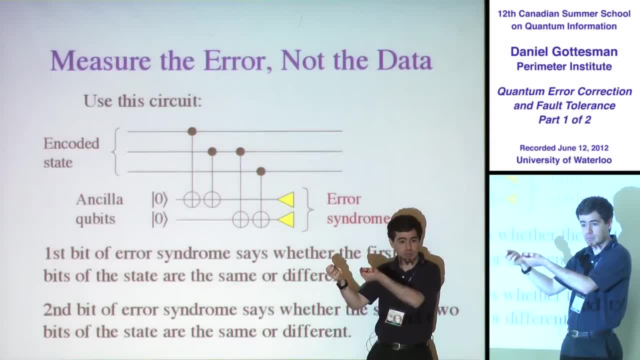 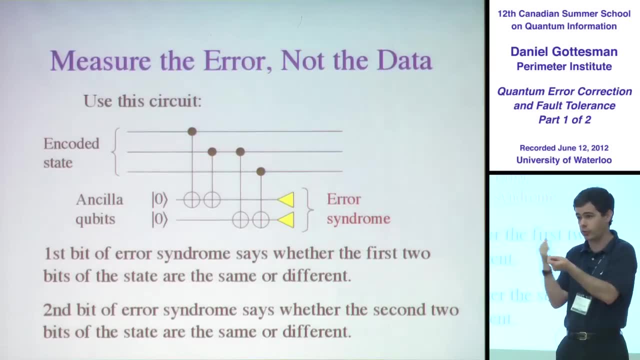 And the second and third qubits are 0, 0, the same, Or it could be 0, 1, 1.. And we don't know that. That's the point. We don't know whether it was 1, 0, 0 or 0, 1, 1.. 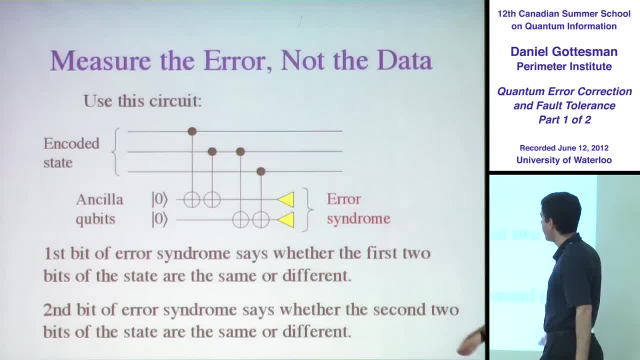 I guess there's really two points. So one of the points is that for each of the three possible errors, or the possibility of no error, we have a different error syndrome. So measuring the error syndrome will tell us what the error was and which qubit it was on. 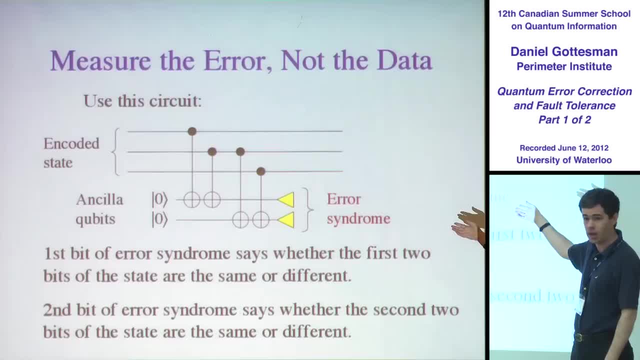 And the other thing is that measuring, that finding that information out, doesn't tell us anything about whether the encoded state was a logical 0, originally encoded as 0, 0, 0, or a logical 1, originally encoded as 1, 1, 1.. 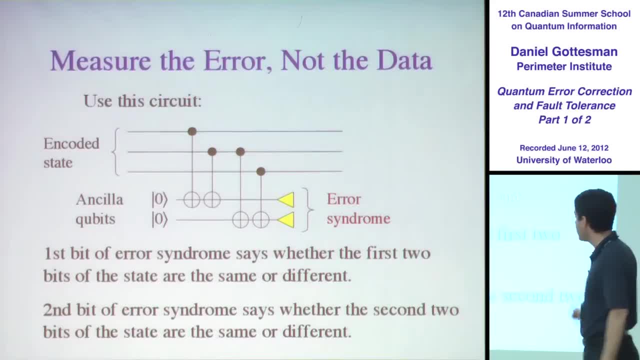 Or, for that matter, a superposition of those two. So making this measurement does not destroy the superposition of the logical states. That's good. That was the first problem we were worried about. We can measure the error without measuring the information. 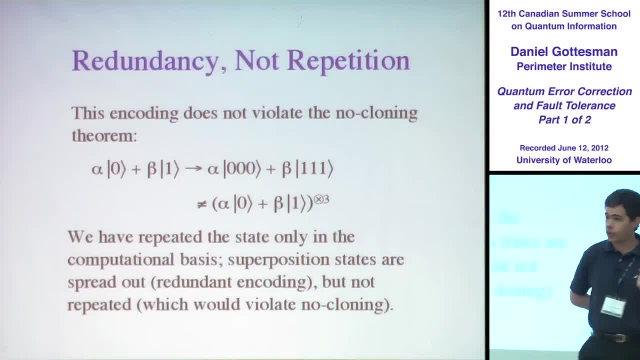 So then, what about the second problem, the no-cloning theorem? Well, you'll notice that this encoding that I gave is not a violation of the no-cloning theorem, Because, while it does encode 0 as 3- 0s and 1 as 3- 1s- 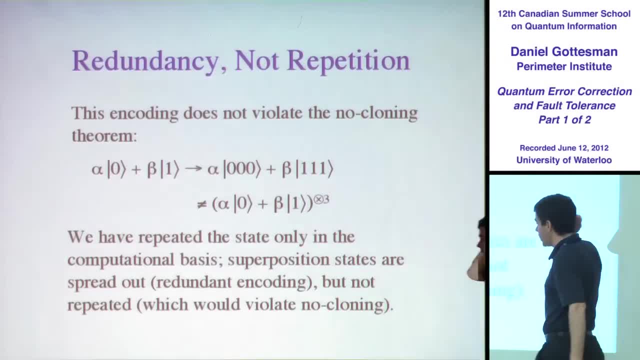 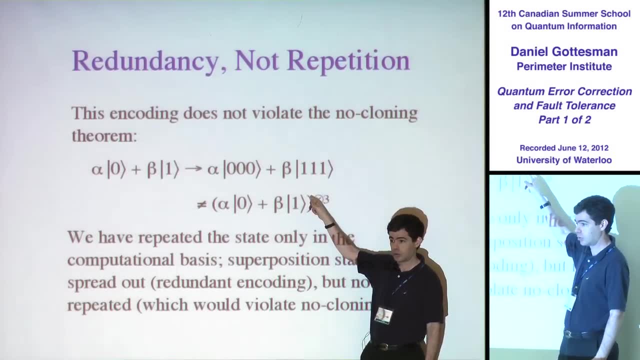 a superposition. alpha 0 plus beta 1, doesn't get encoded as 3 copies of alpha 0 plus beta 1.. Instead, it gets encoded as an entangled state. Okay, So that's okay. We're allowed to copy. 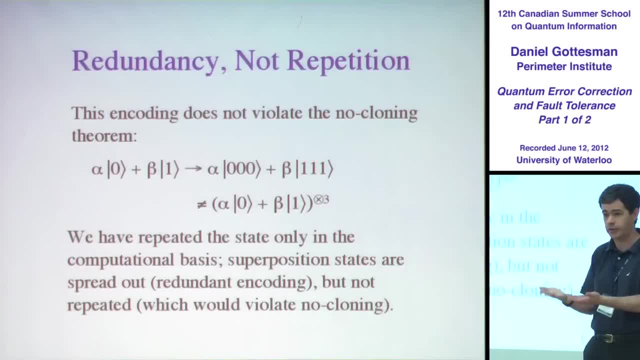 in a single basis, a particular basis, in this case the 0, 1 basis. We're not allowed to copy generic states. Okay, So with this 3-qubit code to correct bit flip errors, we solve these first two problems. 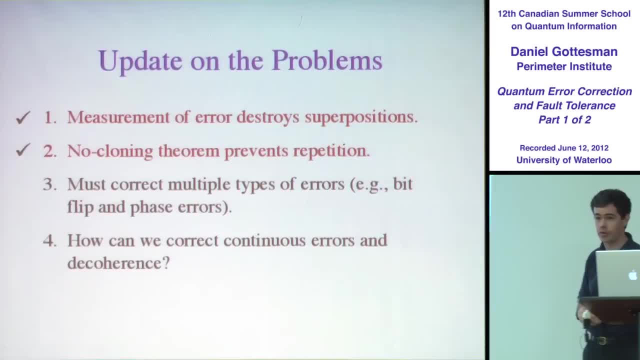 Okay, So going on, let's see how we can deal with these other types of errors. So let's focus for the moment not on correcting all different kinds of errors, but just on one different kind of error: phase errors. So correcting phase errors. 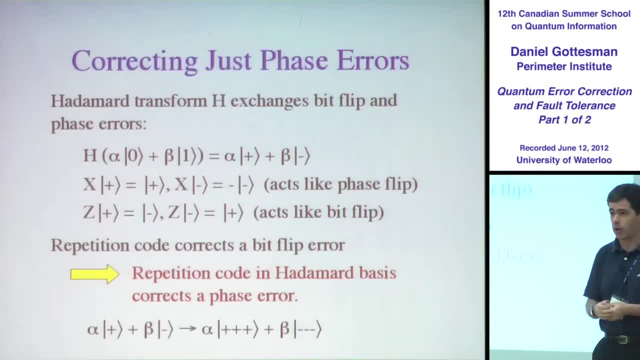 it turns out, is going to be very, very similar to correcting bit flip errors. To correct a bit flip error, we needed 3 qubits and we wanted them all to be the same in the 0, 1 basis And if there's a bit flip, 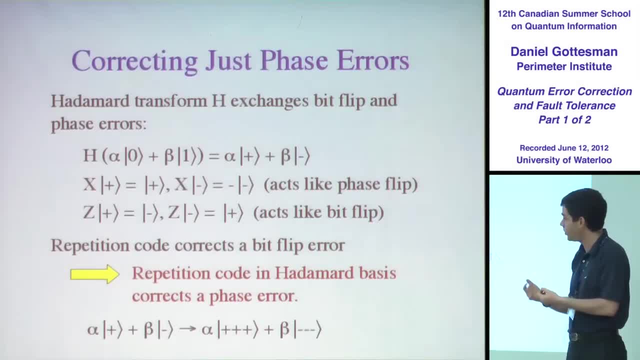 then they're no longer the same. in that basis Now the phase flip acts just the same way as the bit flip, but in a different basis, the plus-minus basis. Okay, Plus is 0, plus 1.. I didn't write it up. 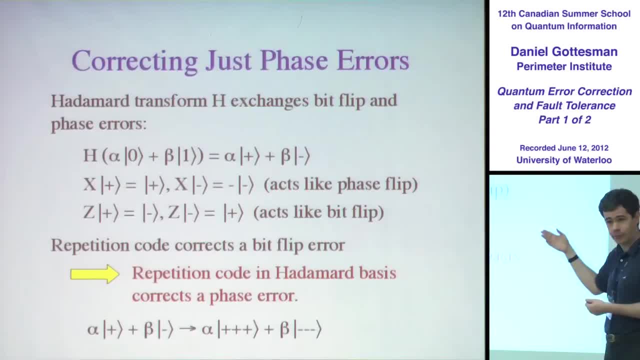 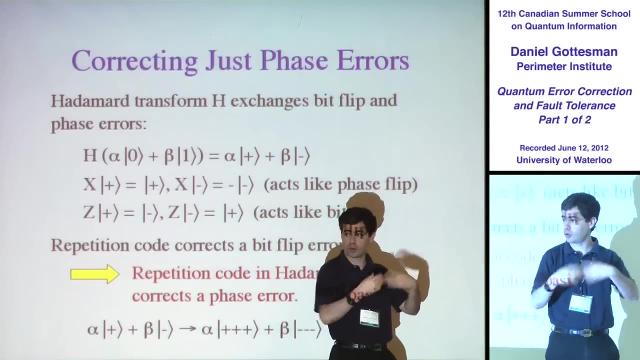 And minus is 0, minus 1.. And the Hadamard transform converts between the 0, 1 basis and the plus-minus basis. Okay, And in the plus-minus basis, as I said, the z operator which in the 0, 1 basis. 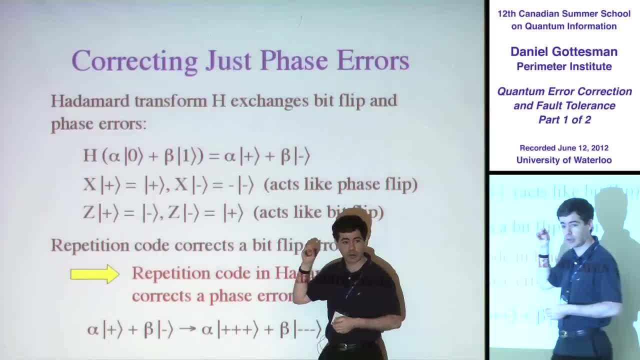 is a phase flip. operator z operator acts like a bit flip Because 0, plus 1 becomes 0, minus 1. And 0, minus 1 becomes 0, plus 1.. So it switches the plus and minus states. 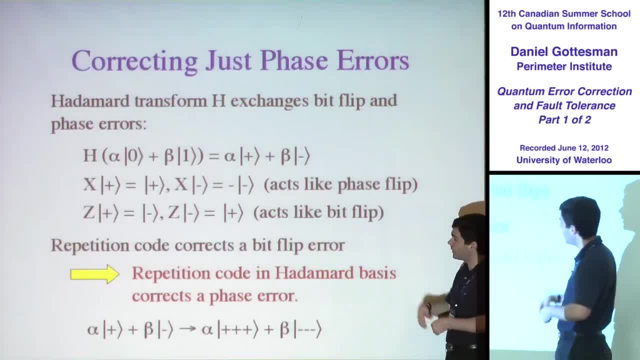 just like the bit flip did in the 0, 1 basis, And x, as it happens, now acts like a phase flip, Because 0, plus 1 becomes 1, plus 0,, which is plus again And 0, minus 1. 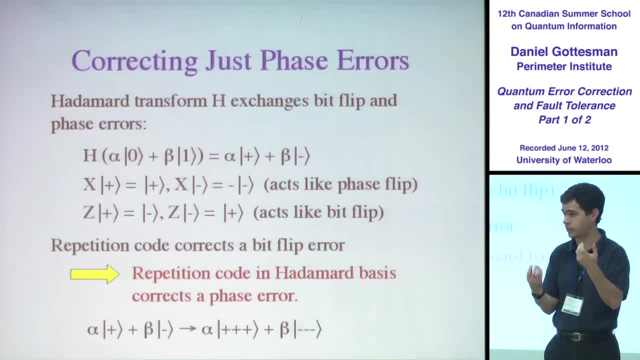 becomes 1, minus 0,, which is minus, minus. Okay, So Hadamard has kind of the effect of switching the x and z operators. So therefore, thinking about this, we can say: oh, to make a code that corrects one phase error. 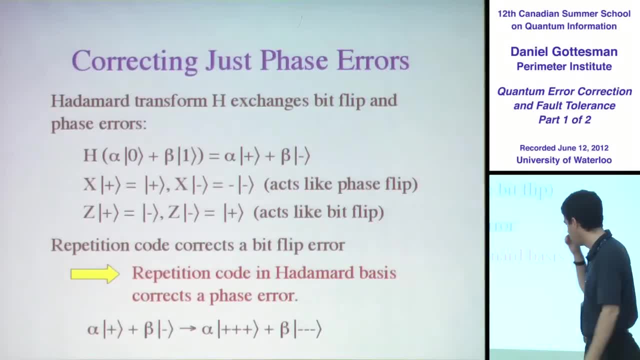 we can just do this repetition code again, but in the plus-minus basis We encode, say alpha plus plus, beta minus, as alpha 3 pluses plus beta 3 minuses. Okay, And then to measure whether one of these is the same or different. 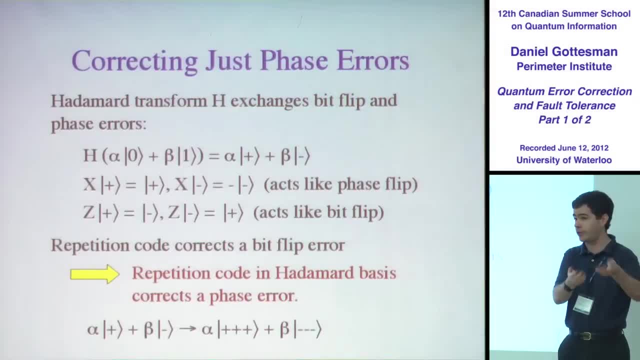 in the plus-minus basis. we do the same you know circuit with the c-naughts, but now we have to do some Hadamard rotations to make sure we're working in the right basis. So this is a code that corrects one phase error. 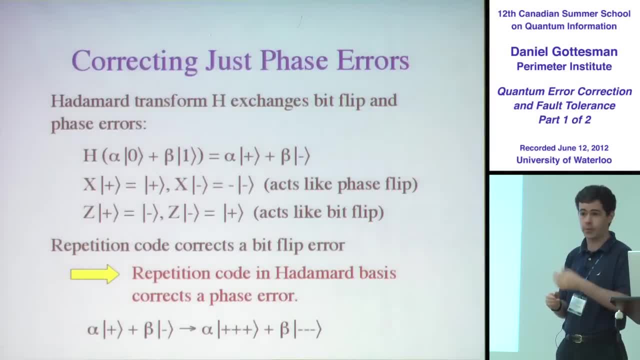 But of course the code that I showed you before to correct a bit flip error didn't correct a phase error, right. In fact it's more sensitive to phase errors Because if you have alpha 0,, 0, 0 plus beta 1,, 1,, 1,. 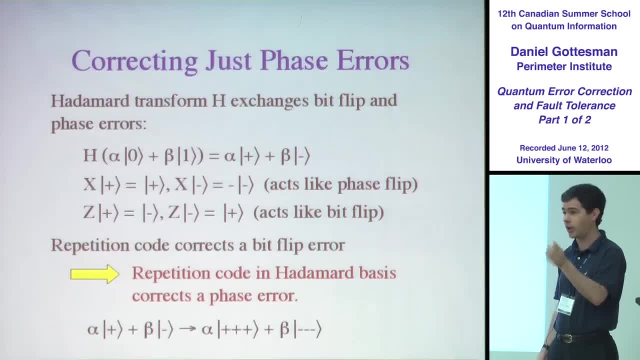 and there's a phase error on any of the three qubits, then you get alpha 0, 0, 0 minus beta 1, 1, 1.. And similarly, this code is very sensitive to bit flip errors. Okay. 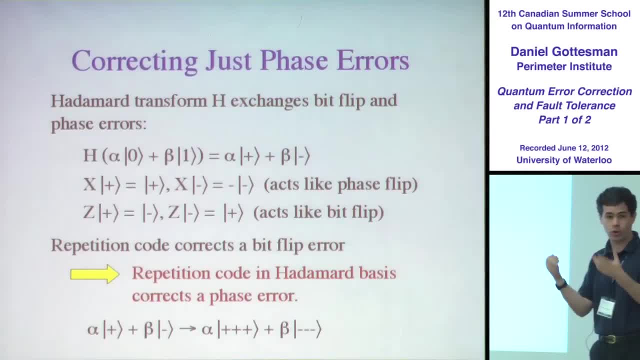 So that's not really very satisfying. We could have a code- a three-qubit code- that corrects a bit flip error but is bad for phase errors, or a code that corrects a phase error but is bad for bit flip errors. We really want something. 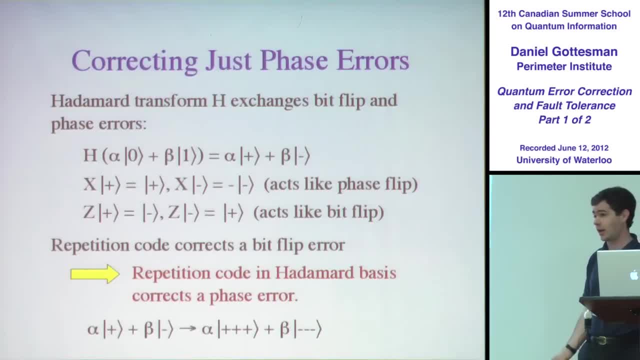 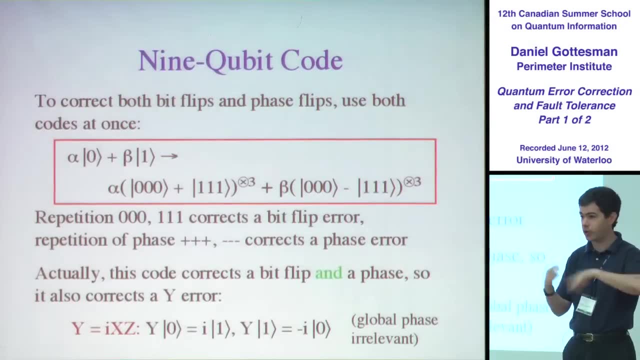 that does both at once, And so to do that we're going to have to add extra qubits. So one way of doing this is to go to nine qubits and kind of combine the bit flip code and the phase code. So in particular, 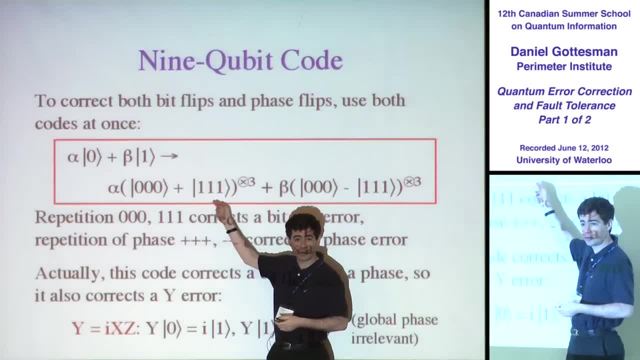 what we can do is we can encode a 0 as three copies of 0, 0, 0 plus 1, 1, 1, and a 1 as three copies of 0, 0, 0 minus 1, 1, 1.. 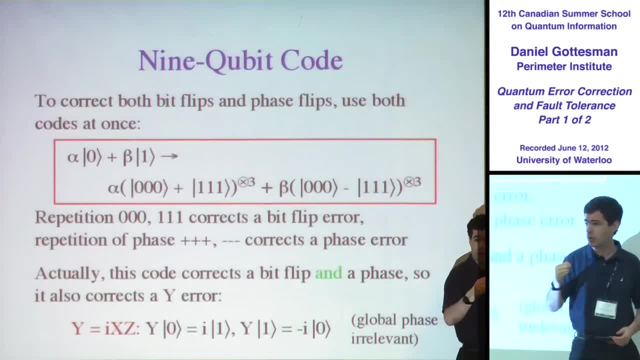 Okay, And then you see, within each block of three, all three qubits are supposed to be the same in the 0, 1 basis And so if there's a bit flip error, we can detect that by seeing that one of those three qubits. 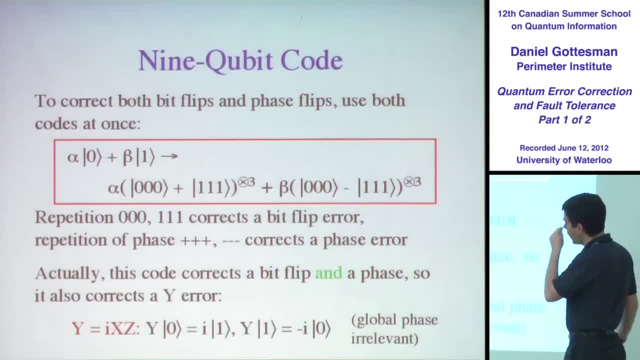 is different. And then, by looking at different blocks of three, all three of the phases are supposed to be the same. They're either supposed to be plus plus plus or minus plus plus, And so by comparing the phases we can see: 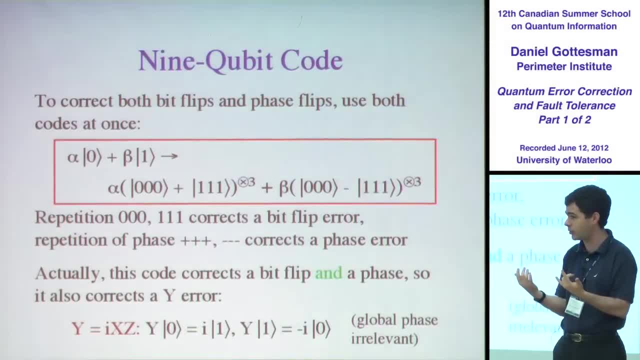 if there's been a phase error, one of those three phases will be different. Okay, And we can, by doing a somewhat more complicated circuit, we can detect that and in fact deduce which set of three had the wrong phase. Okay, 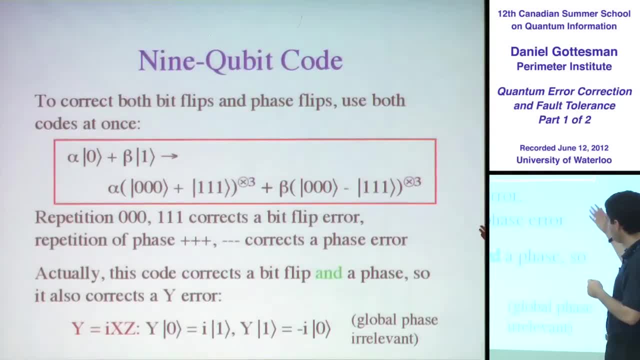 And then we can correct it. So this nine qubit code will correct either a bit flip error or a phase error, And in fact those two processes are totally independent, So we can correct it. So it's fine, It can correct both. 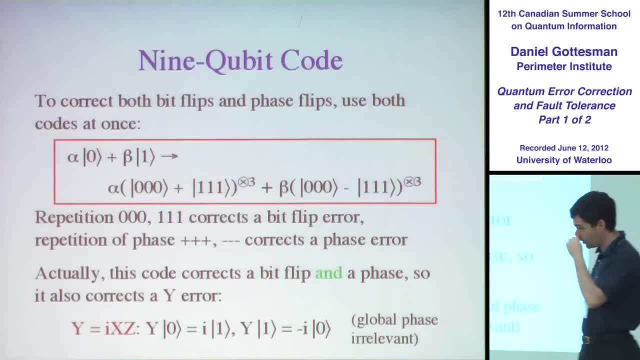 a bit flip error and a phase error And, in particular, that means it corrects one of these Y errors. Right, Because that's a combined bit flip and phase error on the same qubit. Okay, So that's great. So we wanted to make a code. 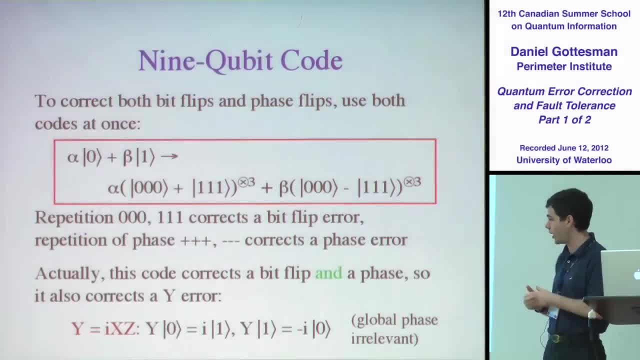 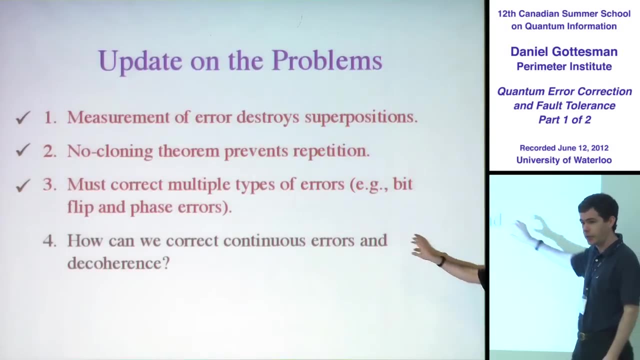 that corrected both bit flip and phase errors, and we were able to do that, And in the process we got an extra error for free. Okay, So we're definitely making progress. But so we've solved three of these problems, But this fourth one. 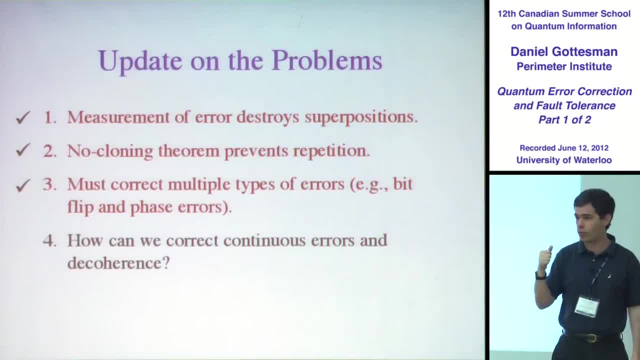 now the trend doesn't look very favorable. Right To go from correcting just bit flip errors to both bit flip and phase errors, we had to go from three qubits to nine qubits, And now this is an infinite set of errors that we want to correct. 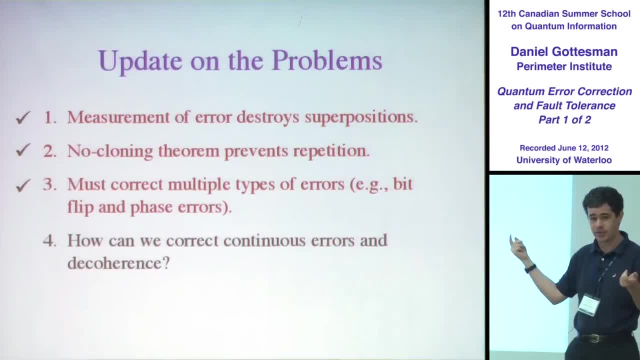 So does that mean we're going to have to go to infinitely many qubits? That would be bad Experiments. have enough trouble making you know five qubits, Let alone a million, Sorry, infinite Okay, But let's just. 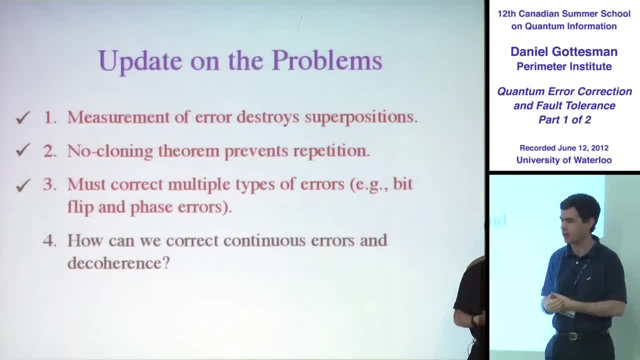 kind of proceed ahead with this nine qubit code and see what we can do with it. In fact, let's do something really very stupid. Let's take this nine qubit code and suppose that we have one of these continuous phase rotations and just pretend. 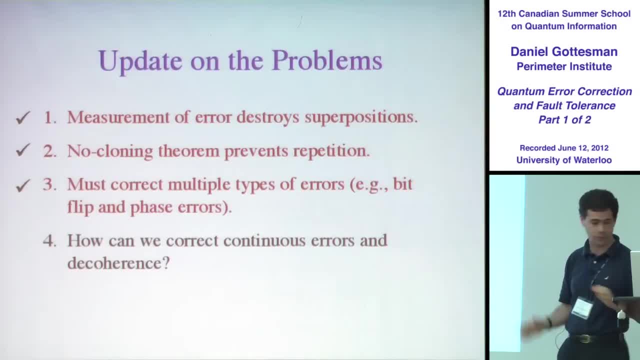 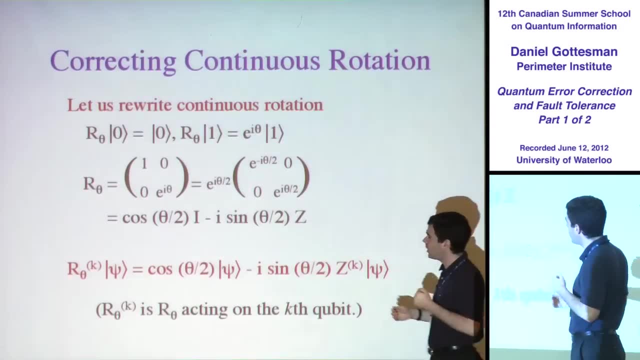 though that it was going to be an X, Y or Z error, And just correct it as if it were. So let's try to analyze what happens when we do this. Well, so this phase rotation, you can write it as a matrix. 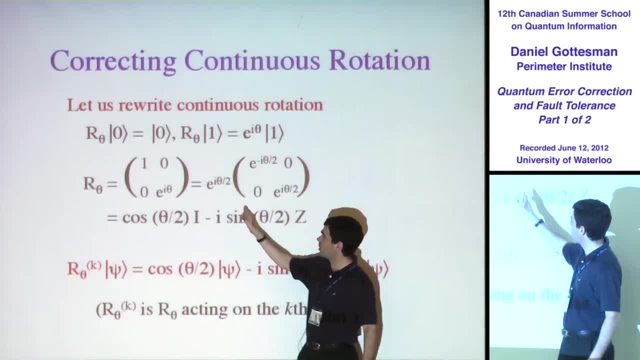 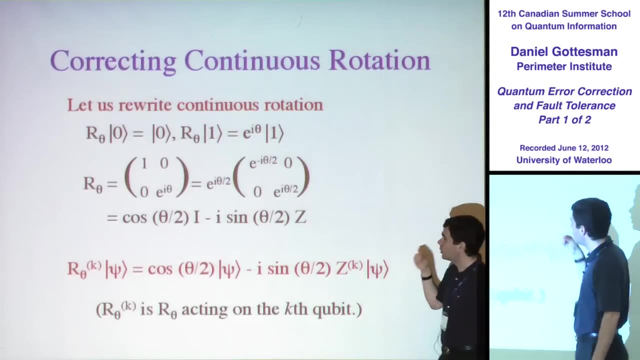 one E to the I theta And pulling out an overall global phase. it doesn't matter, It's this way, which can be written as cosine theta over two times identity minus I sine theta over two times Z. Okay, So, and what that means. 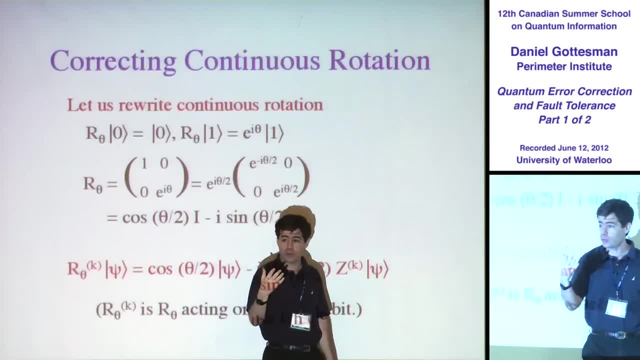 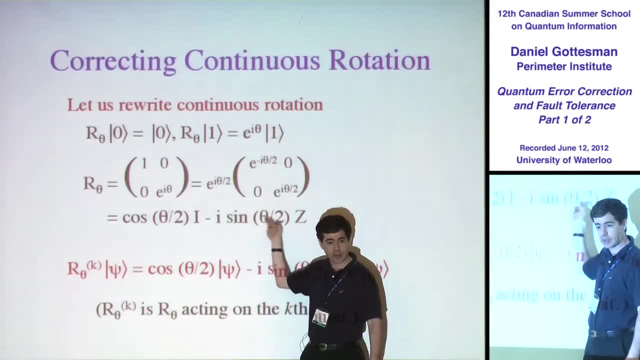 is that if we have this R theta applied to the Kth qubit of our nine qubit code, then we can figure out what happens by expanding this. So R theta K applied to psi is equal to cosine theta over two times identity. 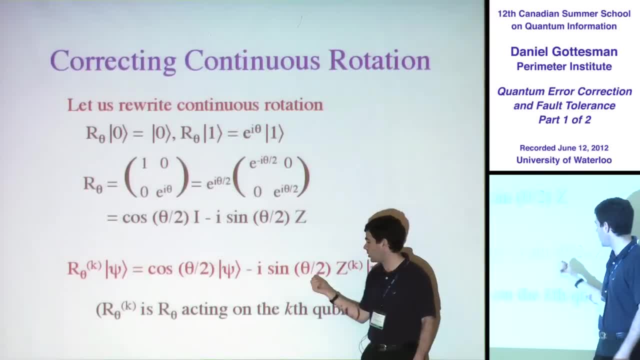 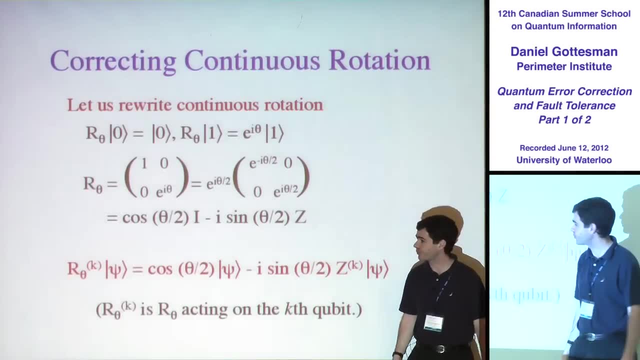 applied to psi minus I sine theta over two times ZK. applied to psi, Again with some global phase E to the I theta over two, which we don't care about. Okay, So far that makes sense, And so now let's. 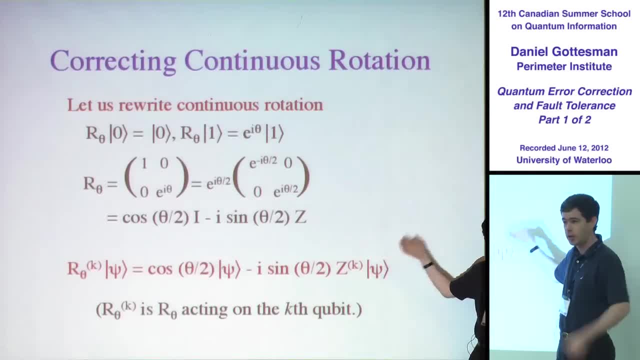 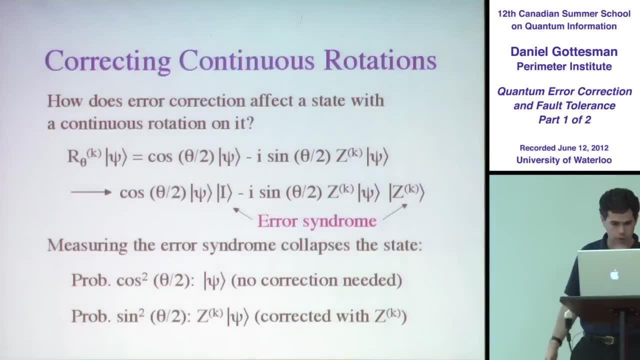 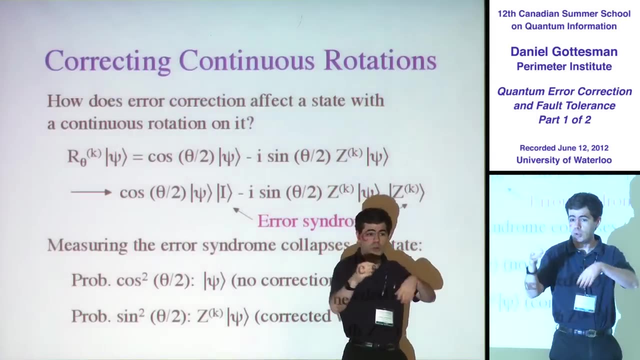 let's try to see what happens when we take this state and we try to error correct it, assuming that the error was actually an X, Y or Z error. Well, suppose we had just this state, psi. Well, when we 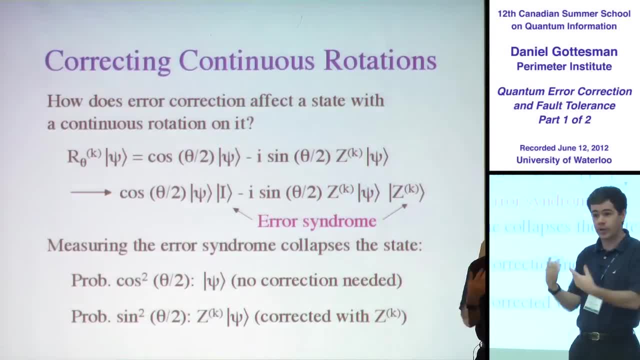 that psi is a correct code word. So when we measure the error synchrome for that we would interact the qubits, the data qubits, with some ancilla qubits And those ancilla qubits would be in a state that tells us: 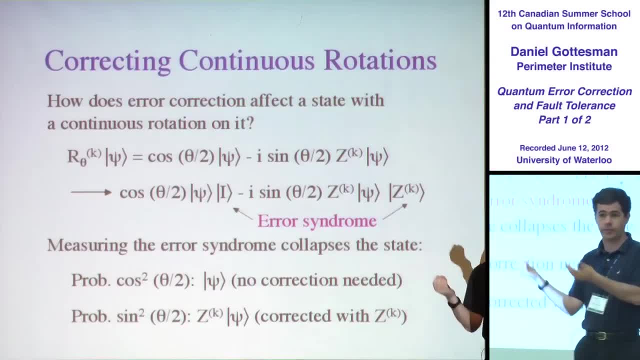 we have no errors, Right? All the qubits are the same in the Z basis and all the phases are the same. Okay, So so this ancilla, then, is supposed to to carry that, that error synchrome which says there's no error. 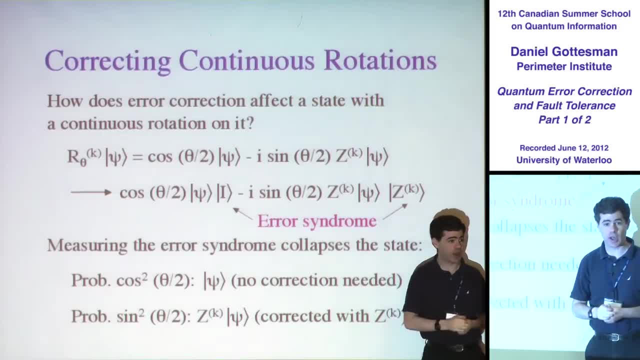 And suppose we had this state: Well, ZK acting on psi, we measure some error, synchrome and the, the ancilla then will, will have some value which tells us there's an error, a, Z error on qubit K. Okay, 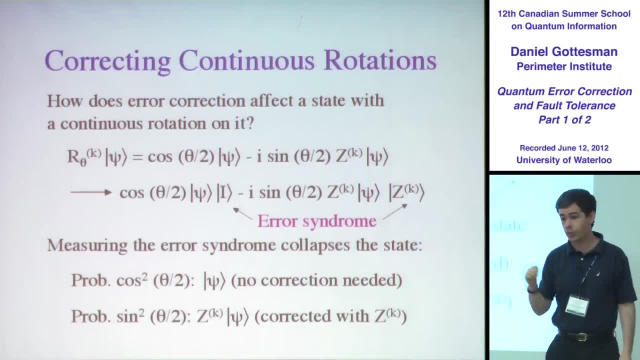 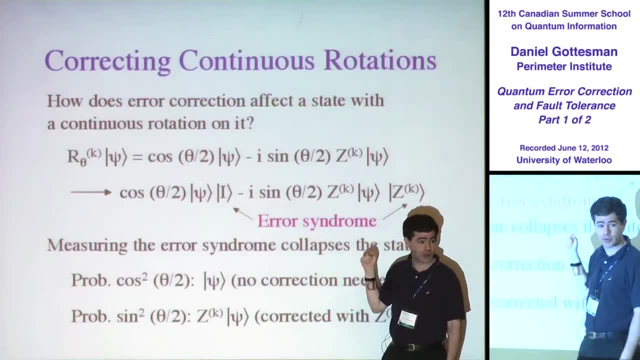 So this would be the, the error synchrome in that case. And of course quantum mechanics is linear. So if we have a superposition of this and this, it must go to the, the linear superposition of those two things. 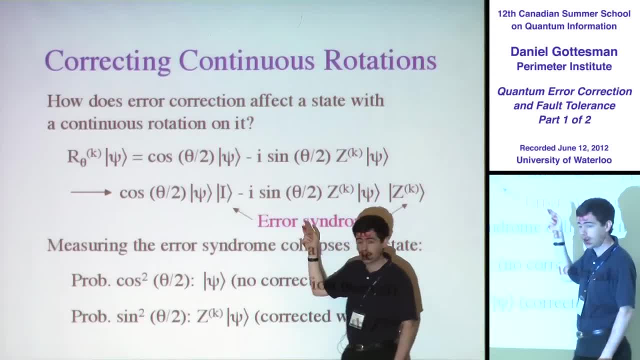 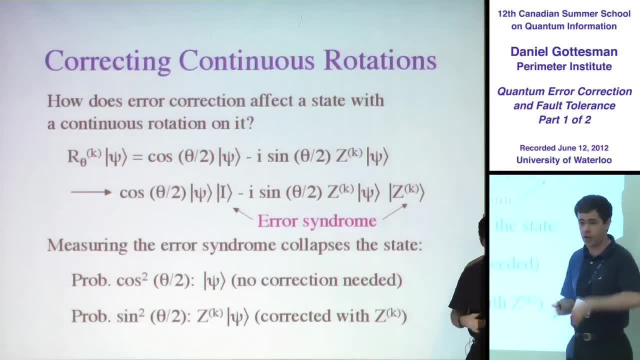 So that's what we have. We have cosine theta over two psi, I minus I sine theta over two ZK psi ZK. Okay. And so at this point I've just done, imagine doing the, the unitary, the. 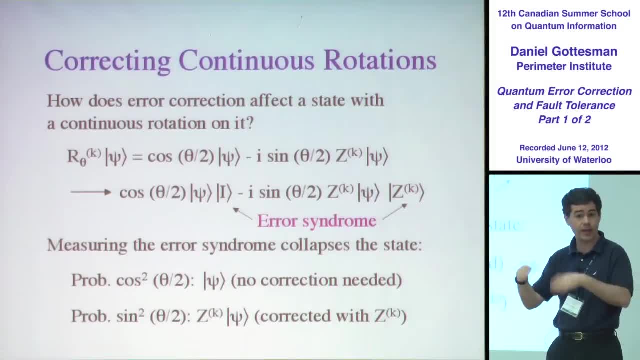 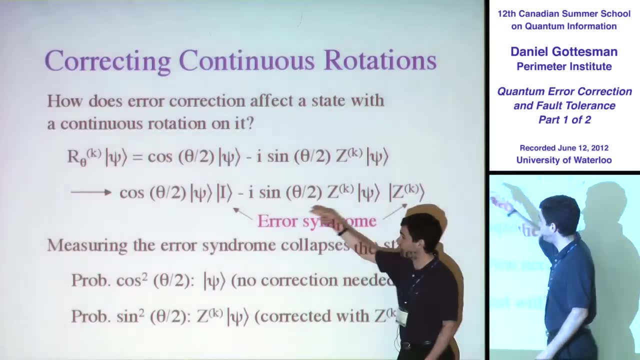 like the control, not gates that interact the qubits with the ancilla. So now let's see what happens when we measure the ancilla To see what the error synchrome is. Well, these are different error synchromes. So 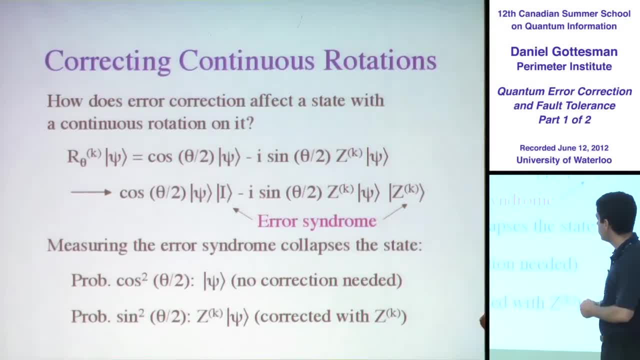 when we measure the error synchrome, there's a collapse And with probability cosine squared theta over two, we get this outcome. With probability sine squared theta over two, we get this outcome Okay. And in this case we measure that the error synchrome says: 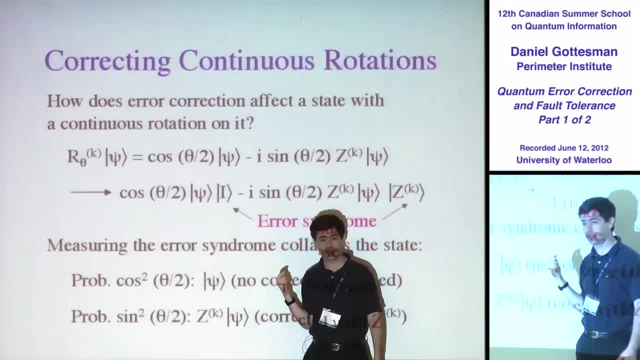 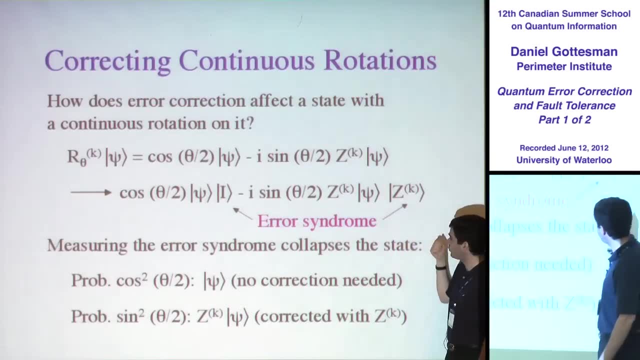 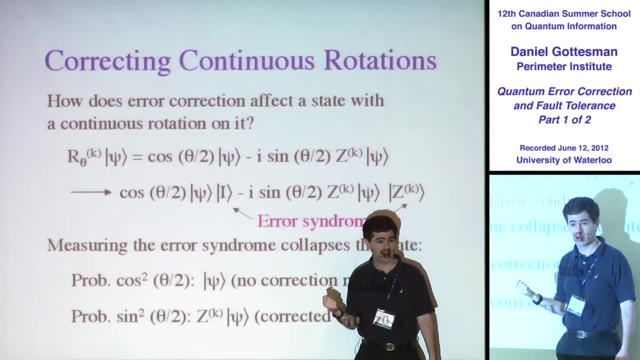 there's no error And the state collapses to psi. So actually it's true, There is no error And when the error synchrome says the error is zk, the state collapses to this zk psi, And the error synchrome tells us. 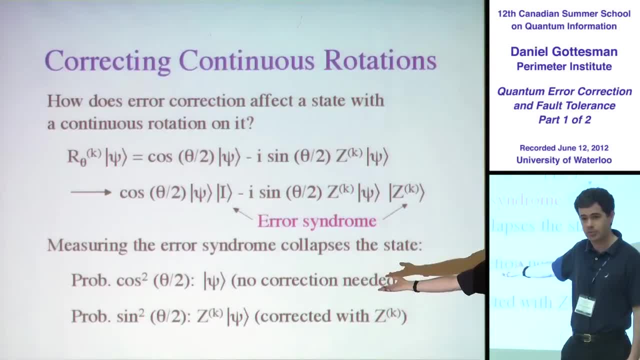 there's an error z on qubit k And actually that's what there is. Okay, So this is really a triumph of wishful thinking By pretending the error was i, x, y or z and making the appropriate measure. 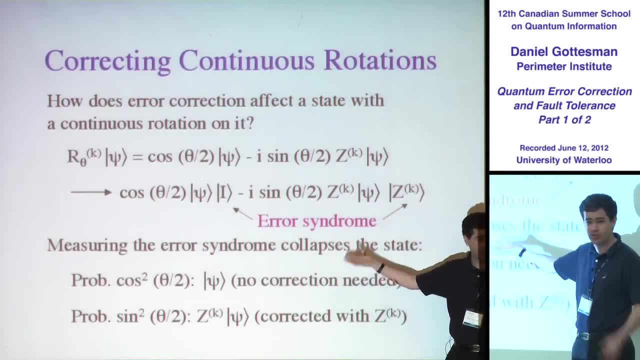 we can measure the error, So we can measure the error, And by making the appropriate measurement, we made that actually the case. It started out as something else, but now it really is the identity, or z. Okay, So this is the magic. 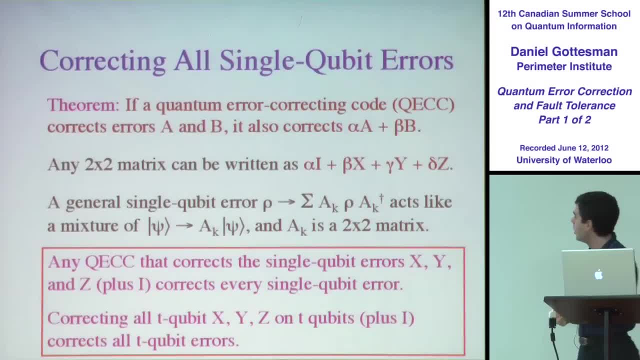 of quantum error correction And you can generalize this much further If you think about that argument. it holds really for any set of errors, not just the identity and z. So in general, if we have a code, a quantum error correcting code, 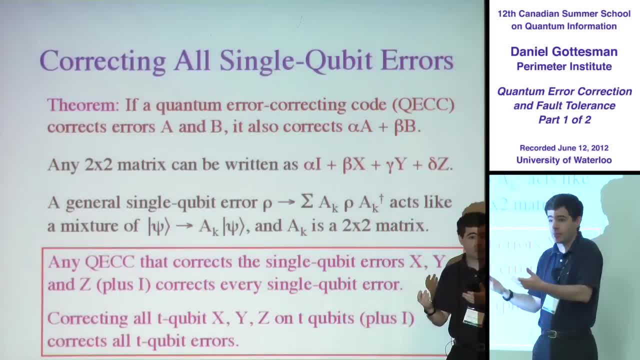 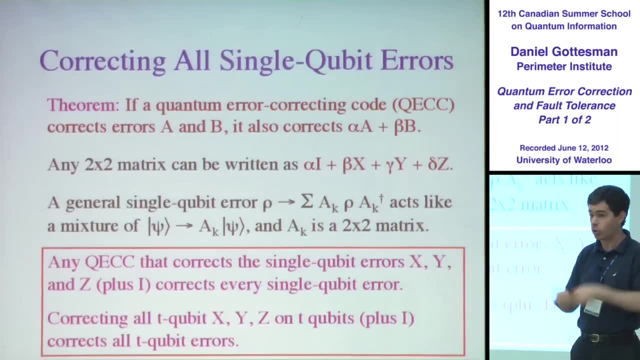 that corrects errors a and b and instead some error alpha a plus beta b occurs. well then, doing the regular correction, assuming a or b will collapse the error to either a or b, just as in the previous slide. Okay. 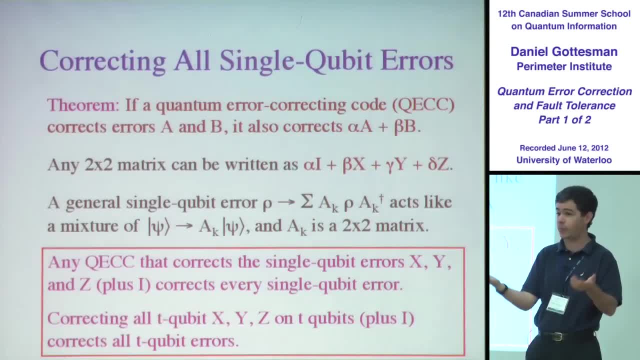 So if we can correct any set of errors, we can correct the linear span of those errors. Think of them as matrices say. Okay, And in particular, any two by two matrix can be written as a linear superposition of i. 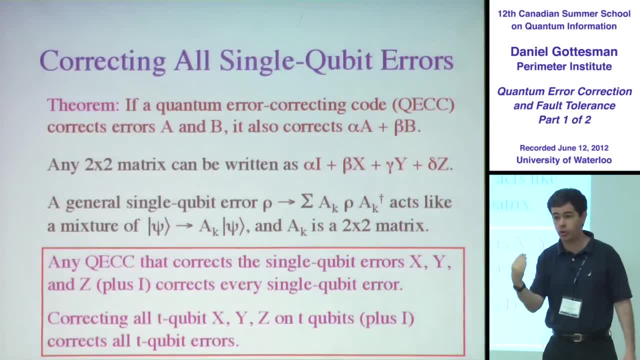 x, y and z, And so what that means is that the non-qubit code, for instance, can correct any two by two error, Any error on a single qubit. Okay, So so far I only told you about single specific matrices. 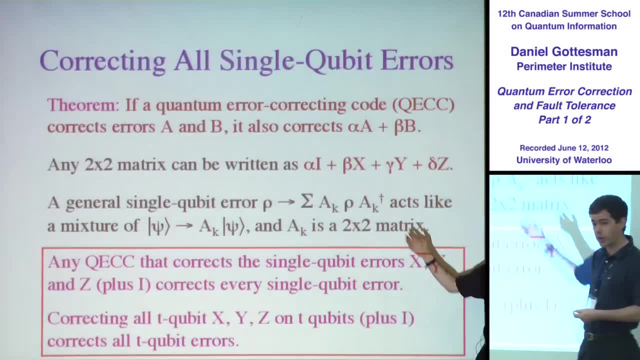 But if you have a general decoherent error, well then you have a mixture of different two by two matrices, And you know this. this property doesn't depend on it being unitary right, So it could be any two by two matrix. 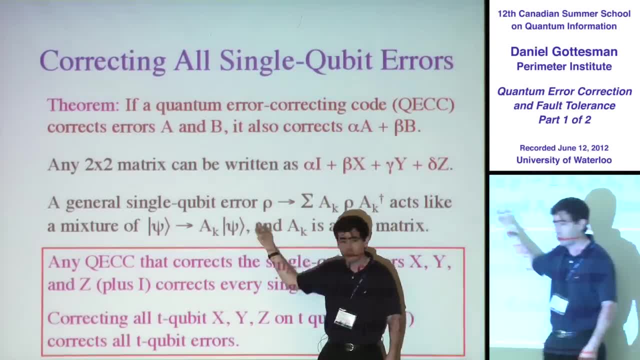 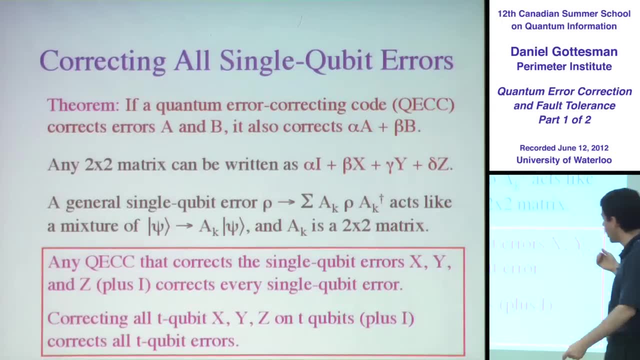 And so what happens is you get a mixture of different two by two matrices, but then the code can correct any two by two matrix. so you're okay. Okay, So the upshot is because this nine qubit code corrects the identity. 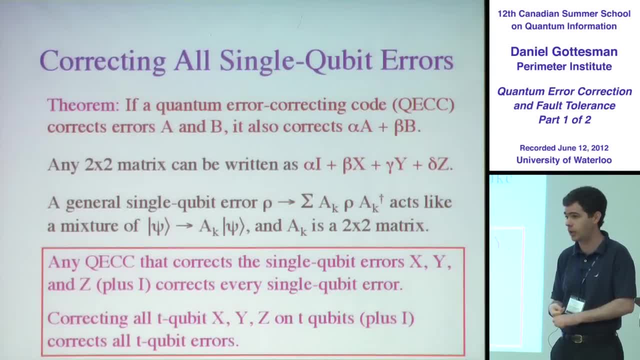 no error, corrects x on any single qubit, y on any single qubit and z on any single qubit. it can correct any single qubit error. And while this nine qubit code only corrects one error, only corrects errors on a single qubit. 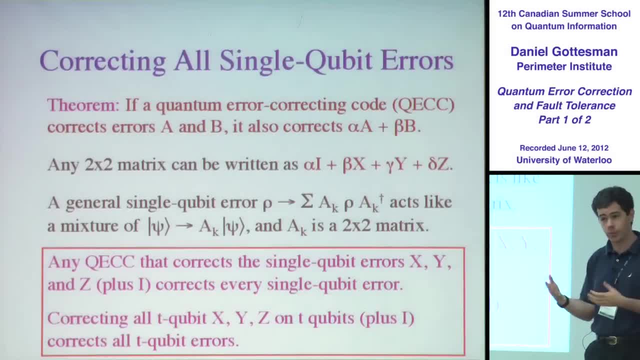 you can come up with other corrects that will correct many errors, and a similar property holds Certainly this: this theorem doesn't make any statement about how many errors you're correcting, And the upshot is that if you have a code that can correct x, 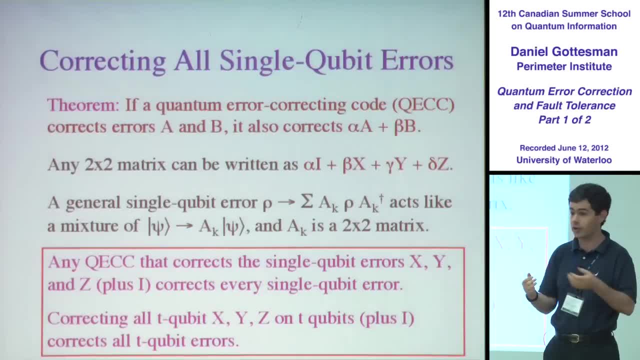 y or z errors that occur on t qubits at a time. you can correct any error that occurs on t qubits at a time, even if it is entangling those t qubits, Because you know. any two to the t by two to the t matrix can be written as: 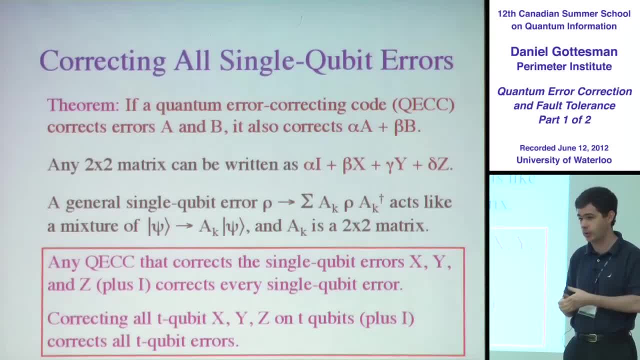 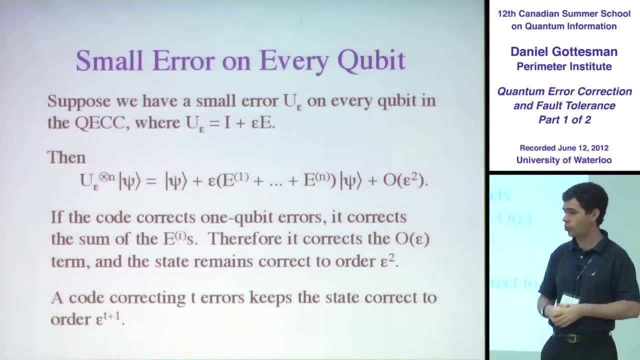 suppositions of tensors, tensor products of i, x, y and z on t qubits, So one other thing that people will frequently worry about. well, okay, so that's fine if you know you have errors on one qubit or t qubits. 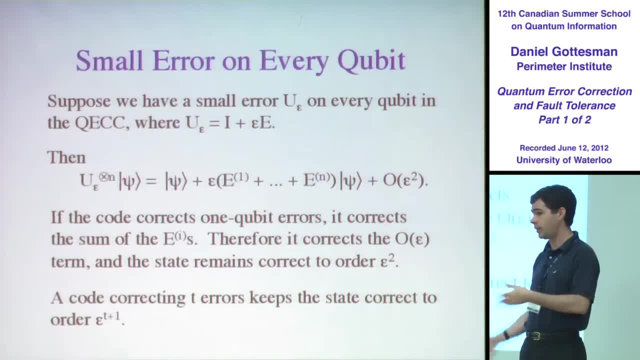 whatever, and that's all that happens. But something that happens very often is you'll have a system where every qubit gets changed by a small amount, So, for instance, there might be small rotation on every qubit, And so 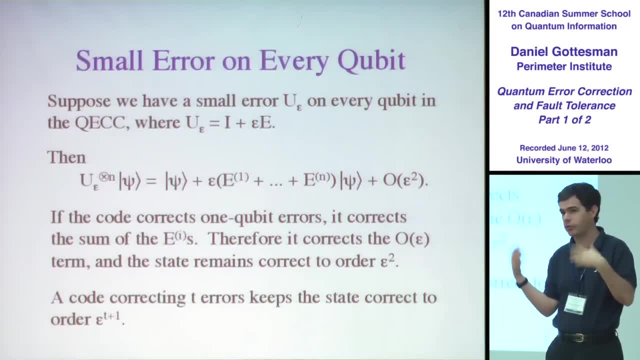 every qubit is under an error, but they're all small errors, so maybe we can still do something, And in fact we don't have to do anything new. We can just use the same codes again. And the reason is that if each qubit undergoes a small rotation, 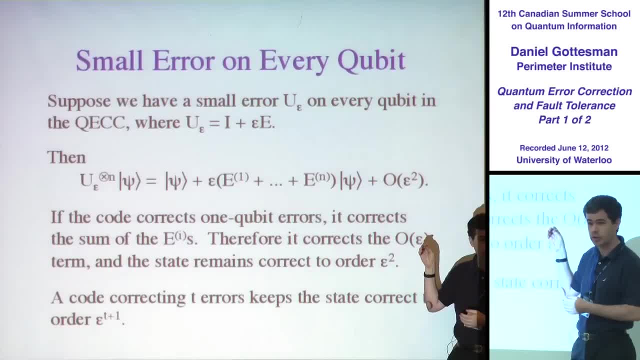 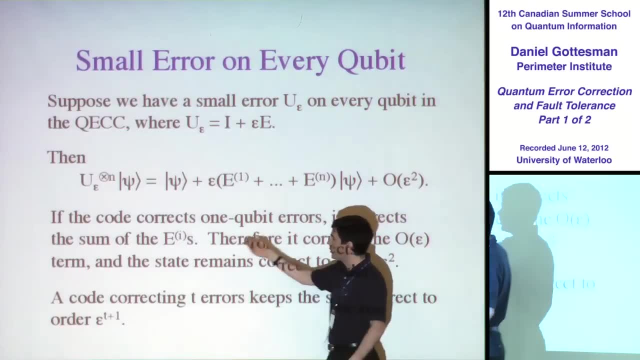 then we can expand the system to to so. so if each error is order epsilon, we can expand it in powers of epsilon and we get the state well to zeroth order. it's just psi again, but there is some. 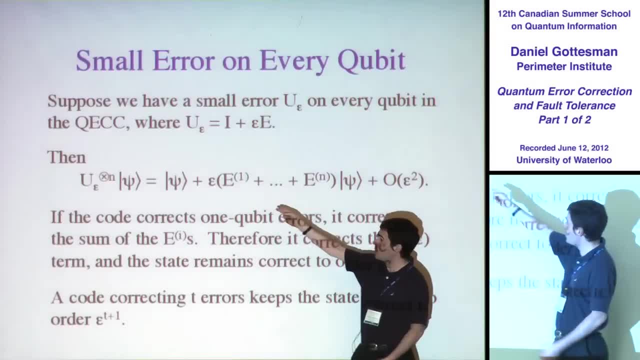 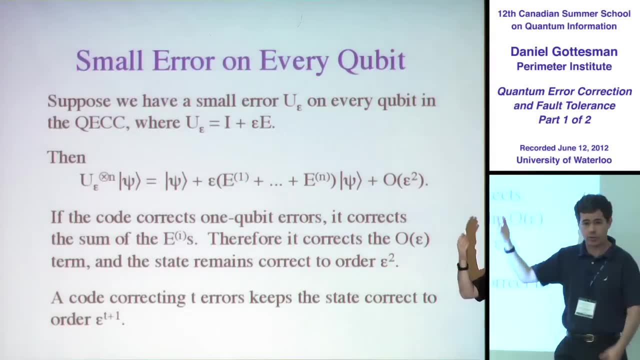 there is some first order error term, epsilon, which is the sum of errors on different qubits applied to psi, And then we have some order epsilon, squared term, that has two errors, and order epsilon, cubed term, that has three errors, and so on. 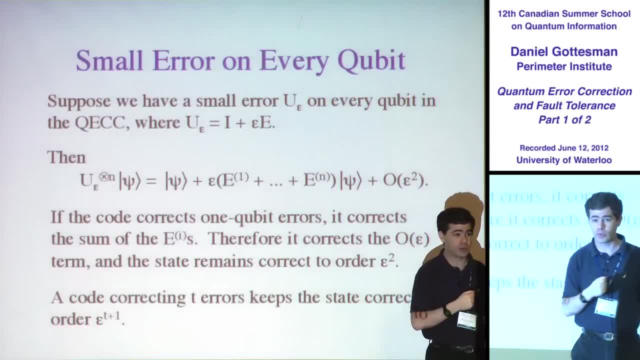 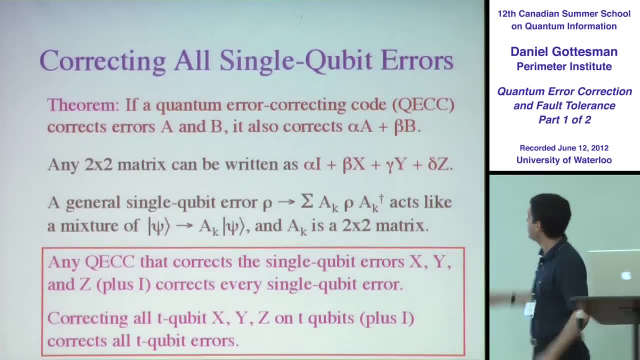 But if we have an error correcting code that corrects any single qubit error, then it corrects the sum of single qubit errors, right, Because you know this theorem also didn't make any restriction that those A and B had to be acting on the same qubits. 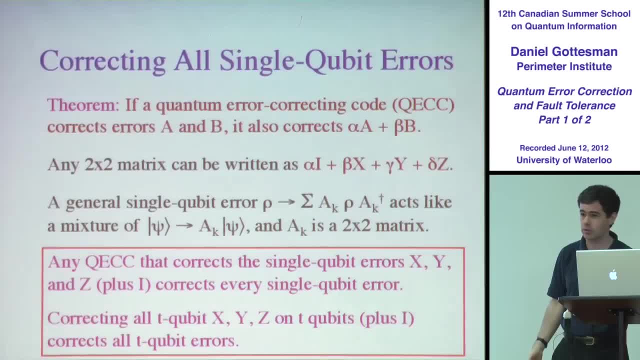 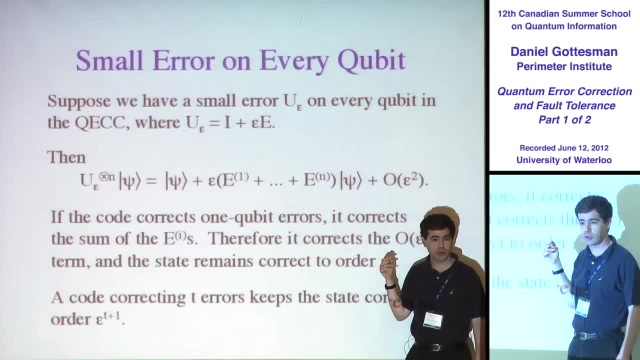 They're just matrices. They can act on any qubits you want and it still works. So the the the nine qubit code, say, or or any other of the error correcting codes I'll be showing you will correct this error. 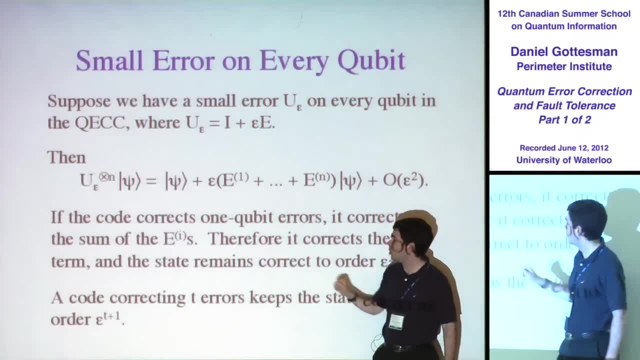 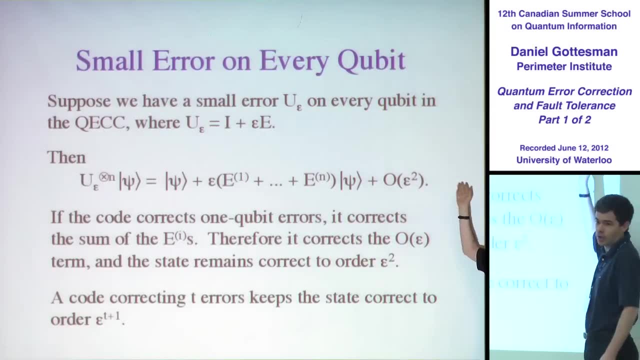 And so this term gets corrected back to psi. This first term, of course, stays psi, because it's the identity we. we want our code to correct that to And this term. well, okay, that my code is something different, But that means that the state that we get out at the end is correct. 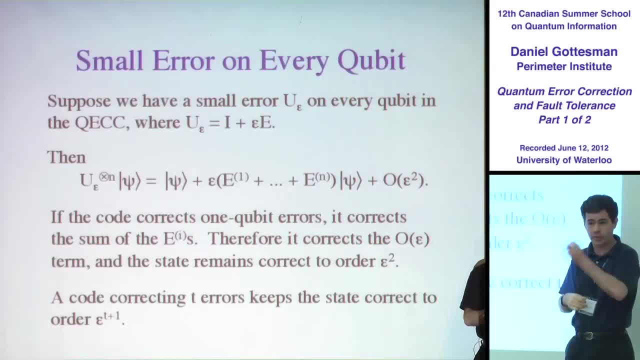 so at order zero, or epsilon to zero and epsilon to the one, and only has errors in order, epsilon squared Okay. So again, this is like the situation with the having a small probability of error per qubit If we didn't encode it. 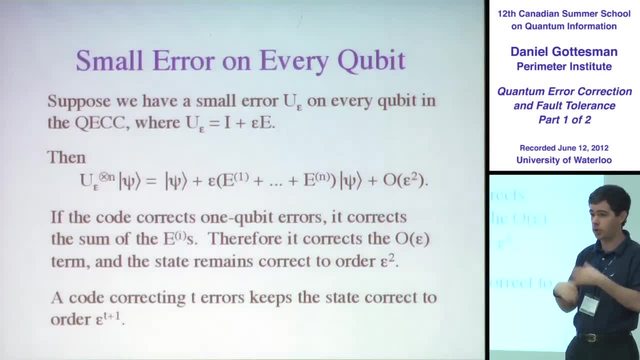 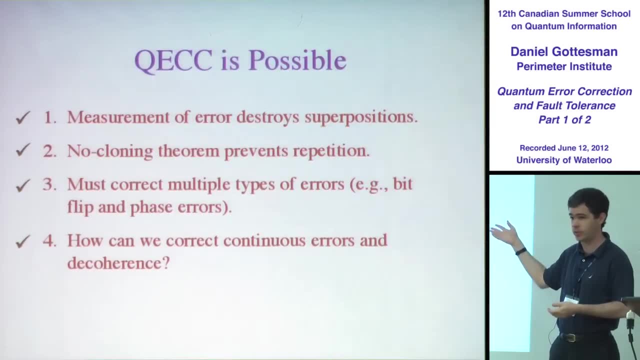 we'd have an error of order epsilon, But by encoding it we can reduce that to an error of order epsilon squared. That solves all this set of problems and it shows you that quantum error correction is possible. So the next thing I'd like to do is is kind of introduce you to 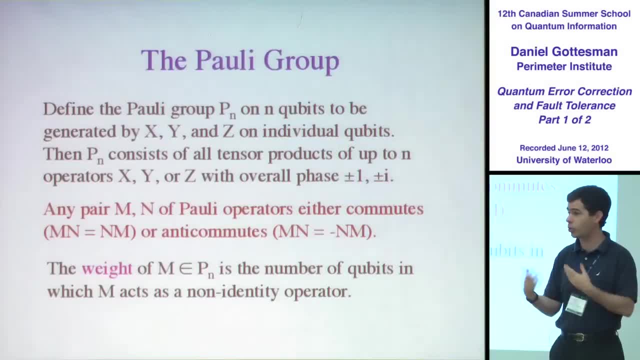 a formalism that that helps deal with quantum error correcting codes and makes finding them and talking about them easier. So to do that first, let's start with with the polygroup. So obviously the poly matrices have already played an important role here. We saw that the nine qubit code is correcting x. 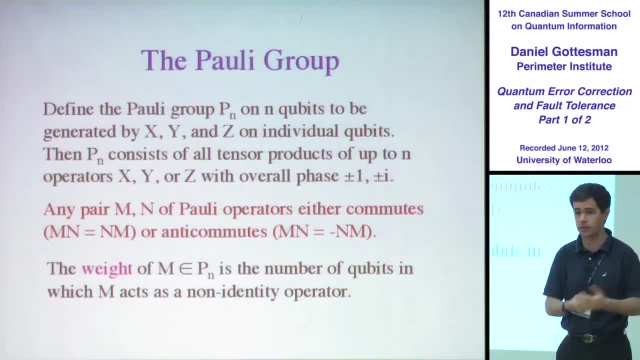 y and z errors and that by thinking about it that way, we can correct arbitrary errors. So what? the definition of the polygroup is then just going to be the group that's generated. It's generated by tensor products of i, x, y and z acting on n qubits. 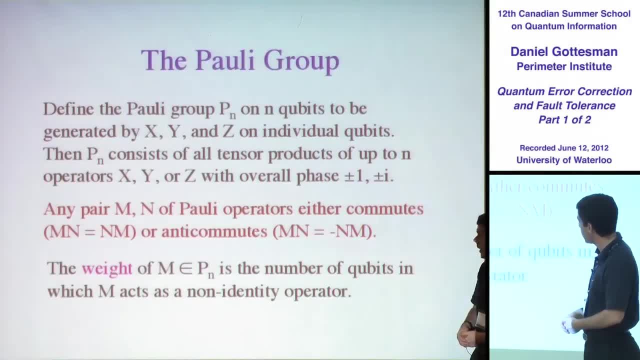 And well, first of all, x and y, y and z, x and z, they all anti-commute with each other. So it's not just enough to have tensor products of i, x, y and z. We'll also need an overall phase of plus one or minus one. 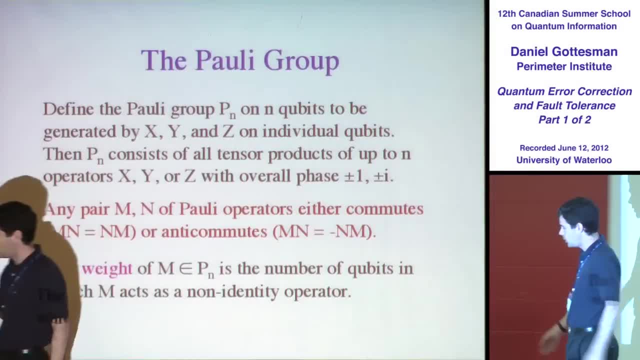 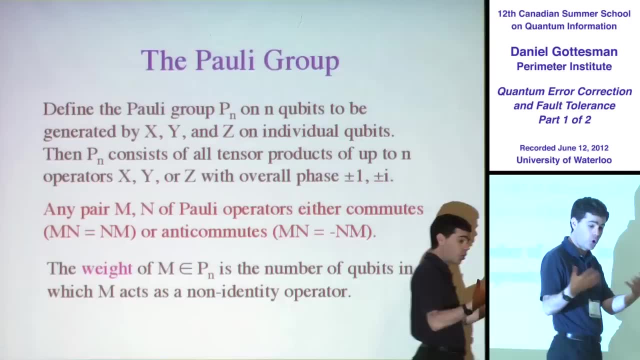 And in fact because we like to write y to make it Hermitian with these i's in it. we also need a phase factor of i. So the overall polygroup consists of tensor products of i, x, y and z on n qubits with an overall phase factor of plus or minus one or plus or minus i. 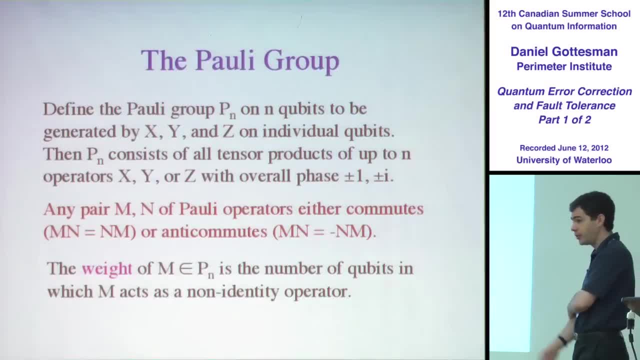 And this polygroup has a lot of very nice properties. So, for instance: well, if you have just one qubit, you know that x, y and z all anti-commute with each other. If you have two, three or more qubits. 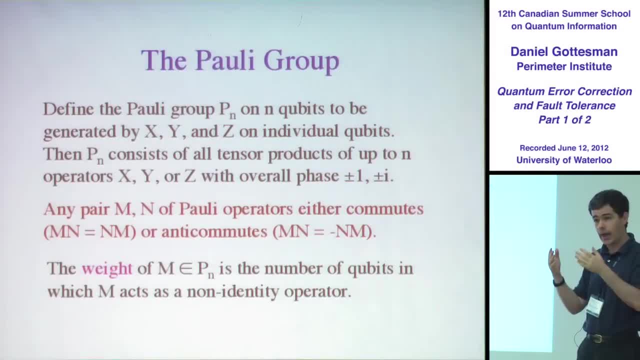 well, you can take any two elements of these polygroup and they either commute or they anti-commute. Now I could say that commutation is, I mean in the, in the, in the one qubit case commutation is kind of trivial right. 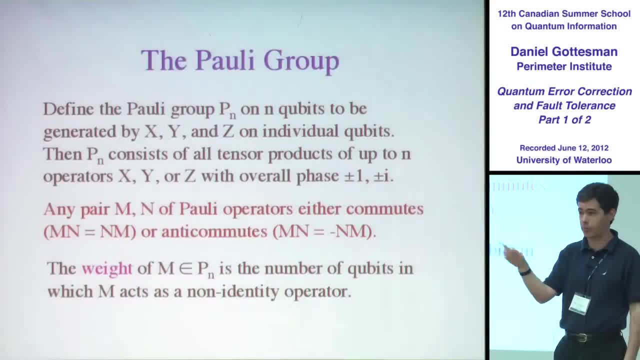 Because the identity commutes with anything. anything commutes with itself, but everything else anti-commutes With two or more qubits. that's not true anymore. You can have non-trivial commutations. So for instance, x tensor x commutes with z tensor z. 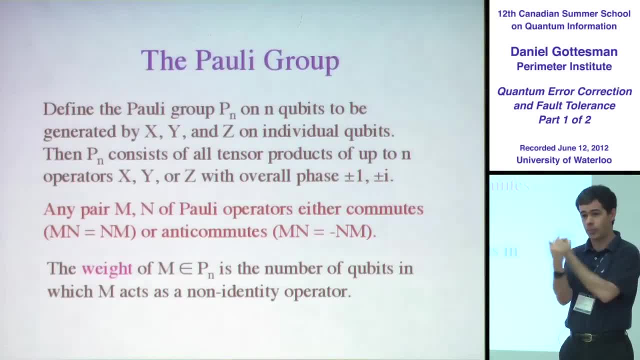 Because if you try to move them past each other, well, x moves past the first. on the first qubit, x moves past z gives you minus one. On the second qubit, x moves past z gives you another, minus one. So you get minus one squared plus one. 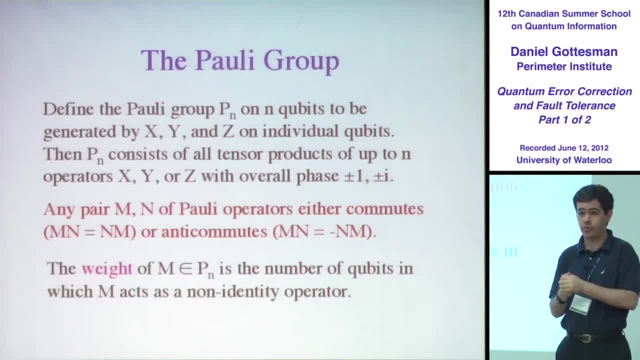 Okay, But but say x tensor z will anti-commute with z tensor z. So you can also have interesting anti-commutation And that's a very important property that we're going to use in a little bit. I guess it's also true that that anything in the polygroup 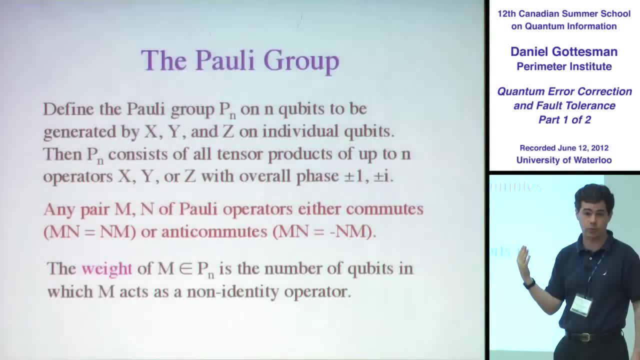 I didn't write it up, but anything in the polygroup squares. it's either plus one or minus one. The things that square to minus one are the things that have this phase factor of i out front. And then one piece of terminology that I'll need is is the weight of an operator. 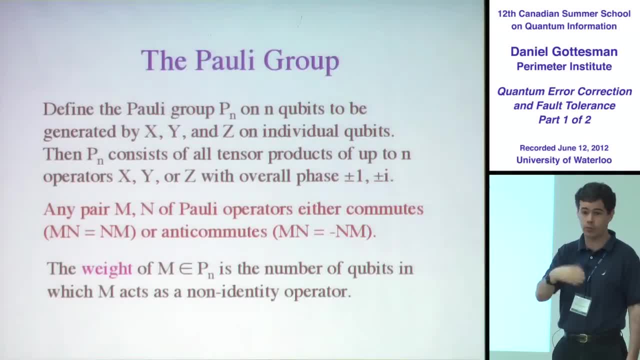 And so the weight of an element of the polygroup is simply the number of qubits on which it acts, not as the identity. So, for instance, if you have i, tensor x, tensor y, tensor z, it's a four qubit operator, but it has weight three because it was the identity on the first qubit. 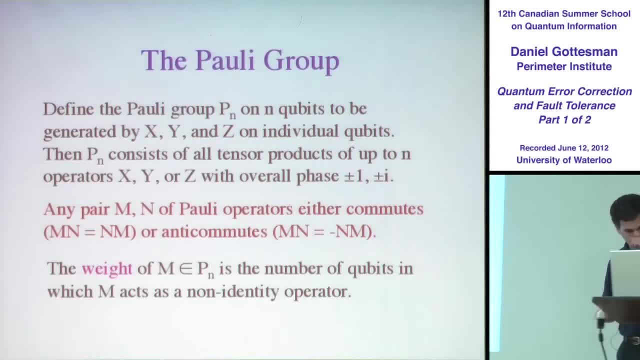 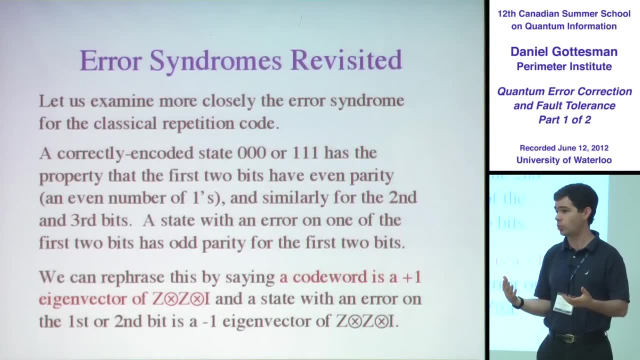 Okay, Okay, so now let's going back, go back to the nine qubit code and think more carefully about exactly why it worked and and how we corrected errors on it. Well, so actually we can go even further back to the repetition code. 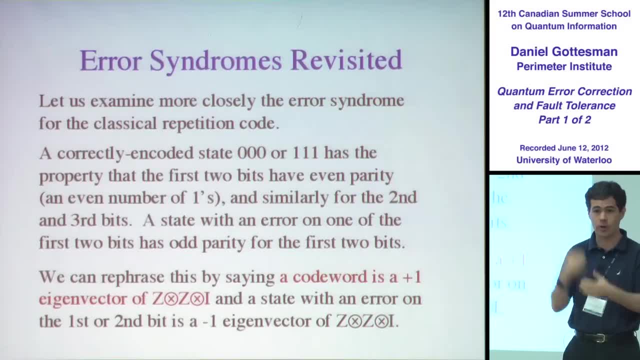 The, the nine qubit code is built out of kind of nested repetition codes, And so in the, in the in the repetition code we want to see whether the first two qubits are the same or different and whether the second and third qubits are the same or different. 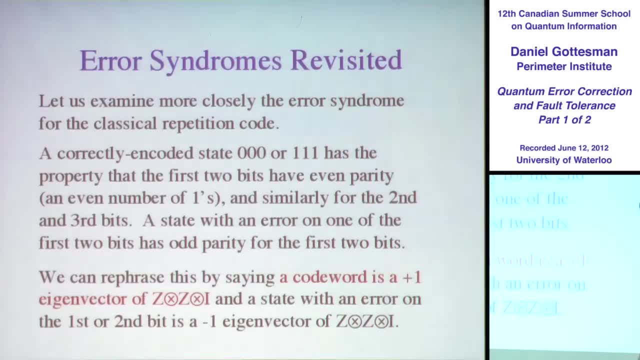 Right, And that'll tell us whether all three bits are the same or not. And one way of rephrasing that is: we want the parity Of the first two bits to be even And of the second and third bits to be even. 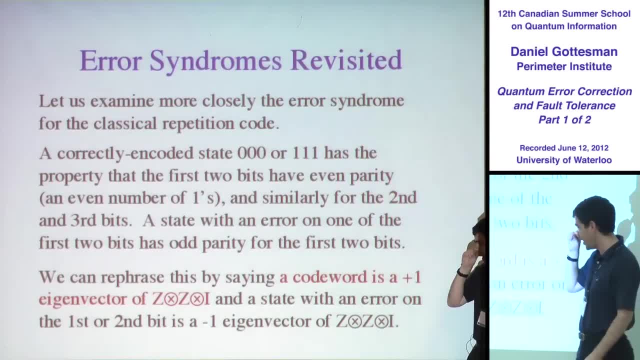 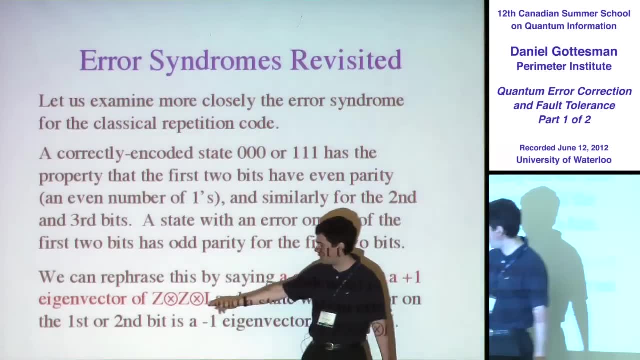 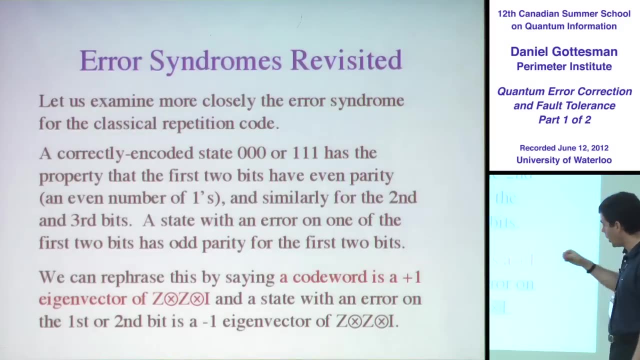 And another way of rephrasing that in more quantum language is to say that the, the- the correct code words are plus one eigenstates of the operator z tensor, z tensor, the identity. Why is that? Well, z has eigenvalues plus one and minus one, for zero and one. 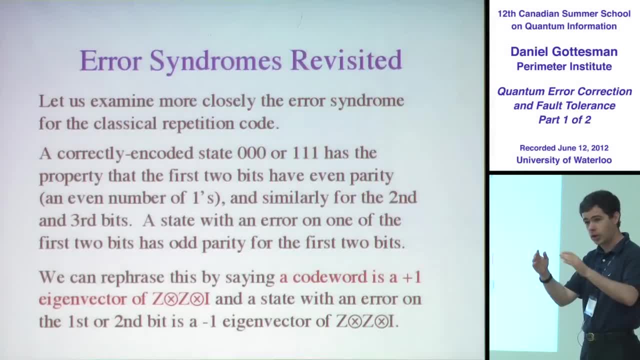 And so z tensor, z, acting on two qubits. well, if they're both zero, we'll get plus one squared as the eigenvalue. If they're both one, we'll get minus one squared as the eigenvalue. So if they're the same, you see, if they have even parity, 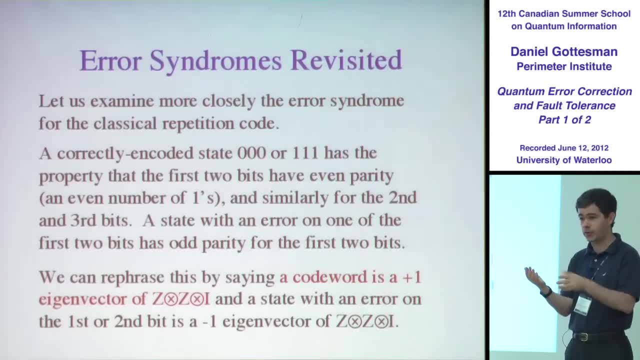 the eigenvalue is plus one, But if they're, they're different. if there's a zero and a one, if there's zero one or one zero, then we'll have eigenvalue minus one, because we'll have plus one for one of the z's and minus one for the other one. 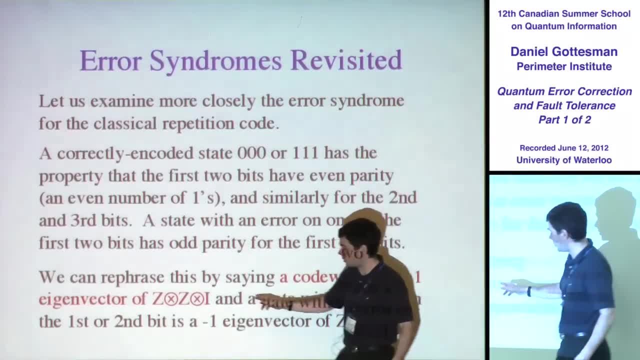 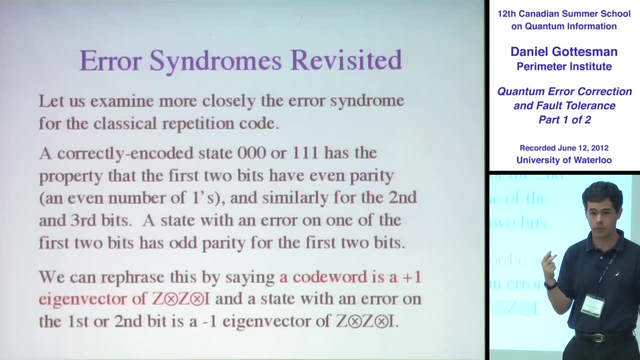 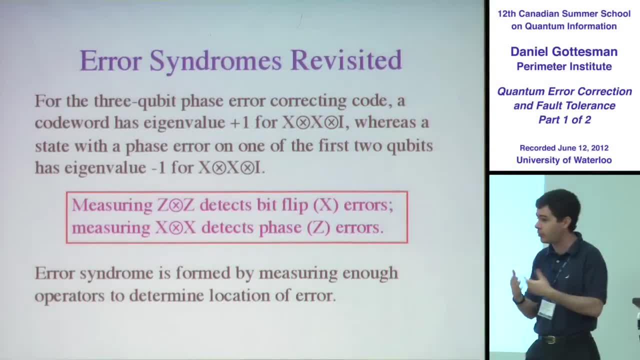 And similarly, if we think about the, the three qubit phase correcting code, well, we did that in the Hadamard basis That switches everything, switches x and z. So whereas the, the, the bit flip correcting code, the correct code words were plus one eigenstates. 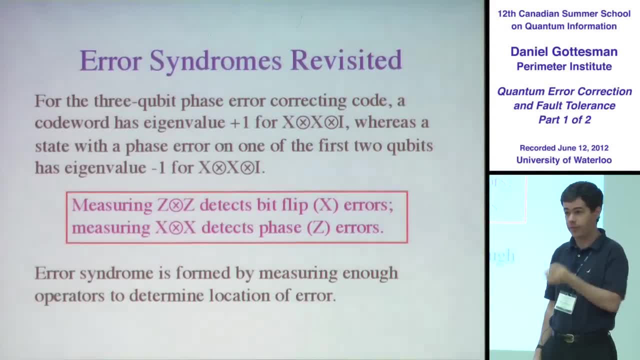 z- tensor z on pairs of qubits. the phase flip correcting code are plus one: eigenstates of x- tensor x on pairs of qubits. Okay so, in other words, to correct bit flip errors, we want a code where the correct code words are eigenstates of z, tensor z and. 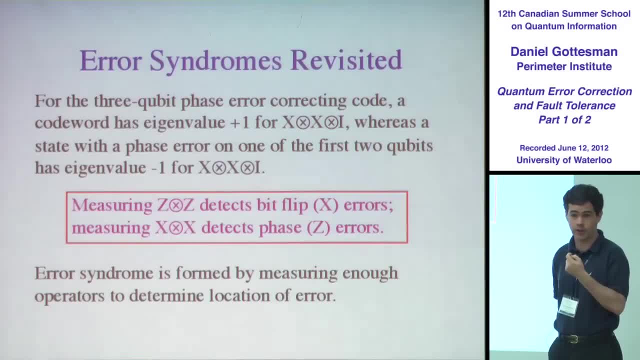 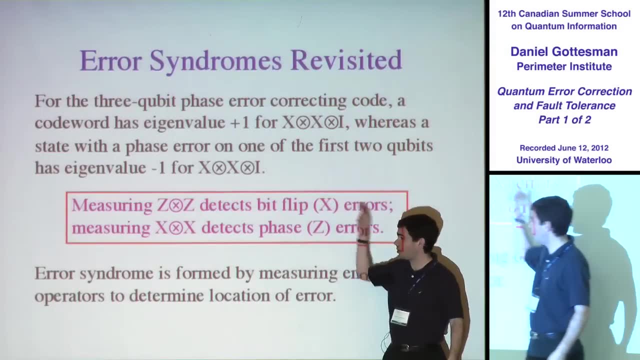 to correct z errors. we want a code where the correct code words are eigenstates of x, tensor x. Okay, there's a pattern here which is that you z's to find out about x errors and x's to find out about z errors. 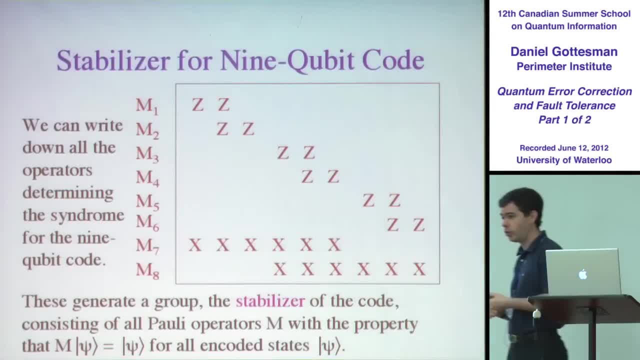 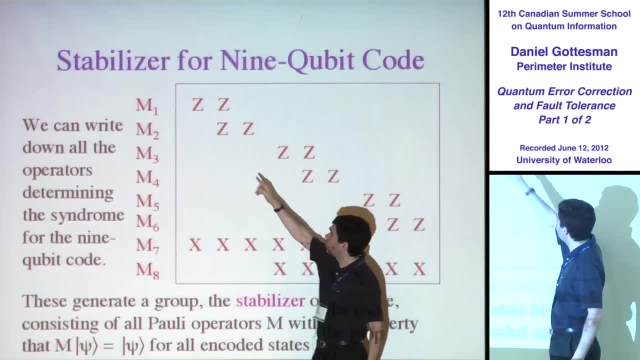 So putting this together for the nine qubit code there's, there's eight things that we want to measure to figure out where the errors are. So first, within each set of three, we measure z tensor z on the first two qubits in the set of three and z tensor z on the second and third qubits. 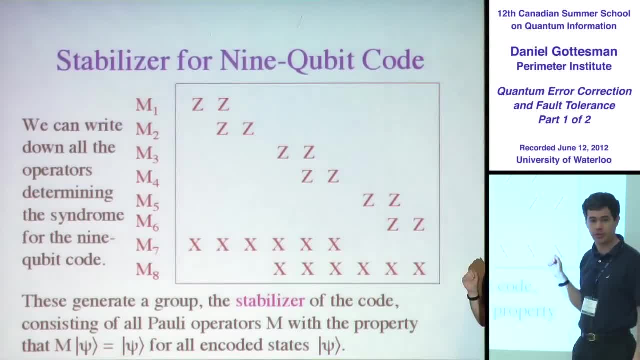 in the set of three, And so each of the rows here is supposed to to to say a thing: that we measure, that we want the eigenvalue to be plus one, and that if it's minus one, that tells us about an error. 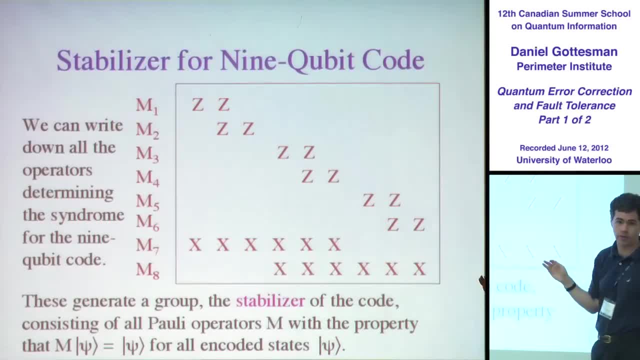 And I've omitted identities in tensor product signs to make it a bit easier to read. So the first operator is z tensor z on the first two qubits. second is z tensor z on qubits two and three, and then we go for the next set of three. 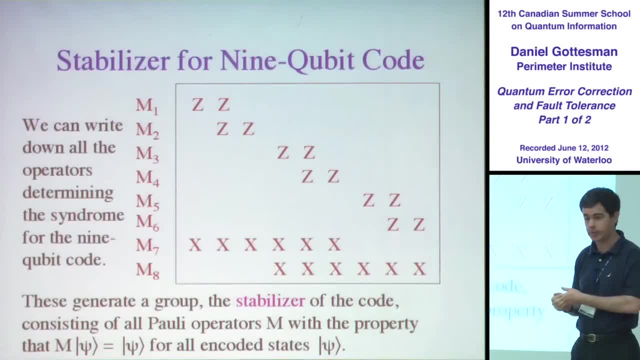 So we have z tensor z on qubits four and five, five and six and then seven and eight, eight and nine, So so these are the things that we measure to to correct bit flip errors on the nine qubit code. Now to 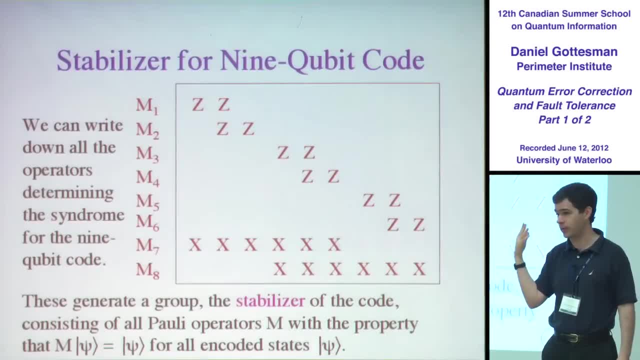 to measure phase errors. we want to do something with x's right The. it's not three qubit code anymore, so it's something a little more complicated. What we'd like to see is whether the, the phases in the first block of three and the second block of three are the same or different. 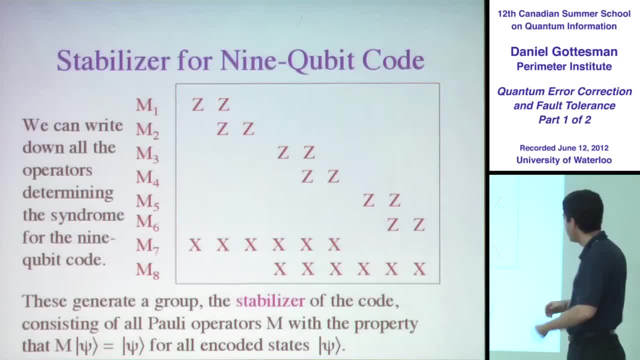 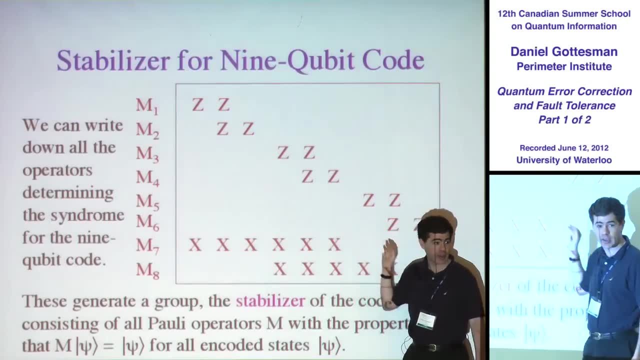 or the phases in the second and third blocks of three are the same or different. And so, to do that, we want to measure the eigenvalues of this operator. well, for the sec-, the first and second blocks involving six x's. Why is that? Well, if we just did a bit flip on, 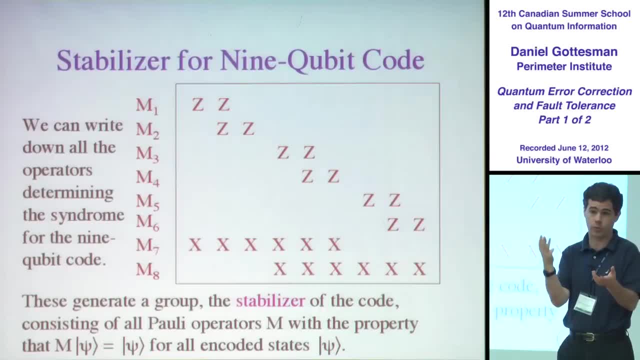 remember, the first block of three is supposed to be zero, zero, zero plus or minus one one one. and if we just flipped one qubit in that block of three you might get you know one zero, zero plus or minus zero one one. So it's not an eigenvalue of that, an eigenvector of that at all. 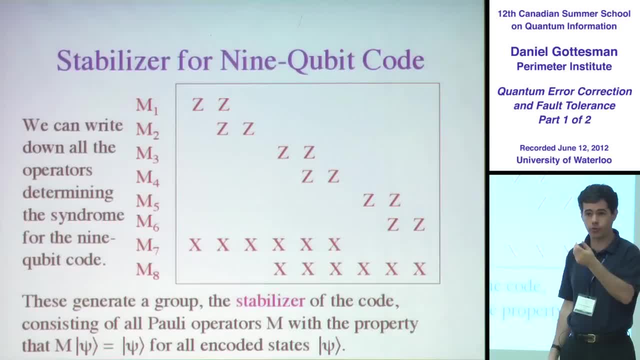 But if we flip all three qubits, then zero, zero, zero, plus or minus one, one one will go to one, one one plus or minus, zero, zero, zero, which is plus or minus the original state. okay. So zero, zero, zero, plus or minus one one one is a is a plus or minus. 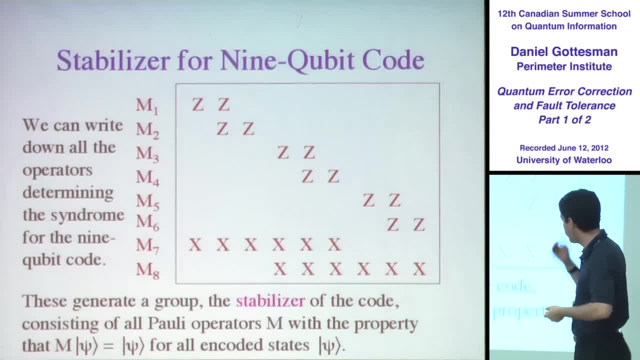 eigenvalue of xxx And therefore measuring x's on all six qubits. well, if the the we have two blocks of three with the same phase, we'll get the same phase twice and we'll have an overall eigenvalue of plus one. and if they have different phases, 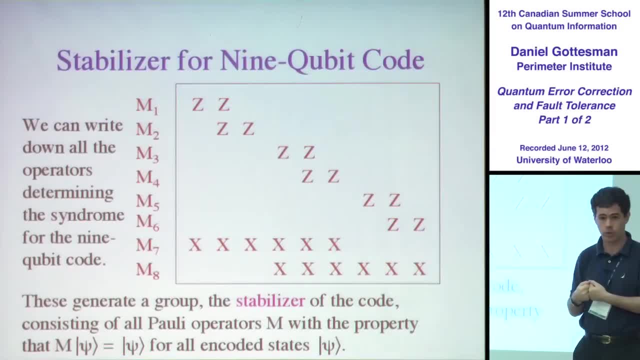 we'll get an overall eigenvalue of minus one. Okay, So measuring these two things will tell us whether all three phases are the same And therefore, measuring these eight things, that tells us the information we need to correct errors on the nine qubit code. 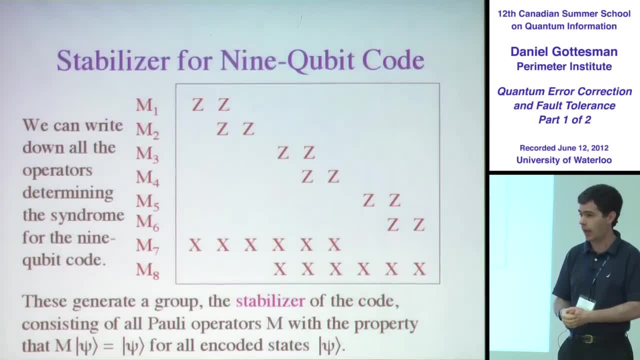 gives us the error syndrome for the nine qubit code, and we can go from there. So the the next step is to say, well, let's try to generalize this, Let's try to make up other quantum error correcting codes based on the same kinds of principles And 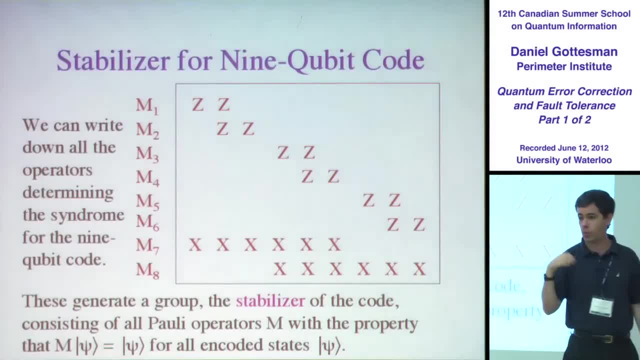 well, if you think about it, this is a list of eight things: that where the eight operators where the code has eigenvalue plus one, but there's other operators that also have eigenvalue plus one for this code. So, for instance, 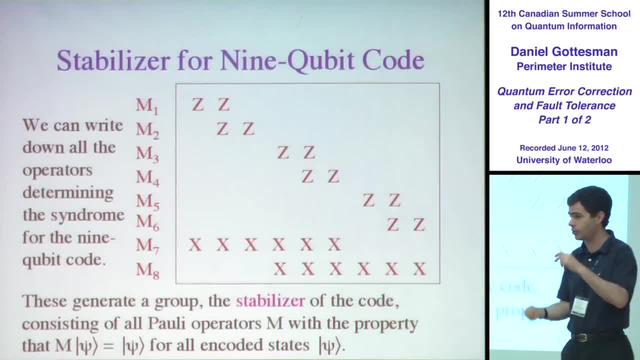 well, we said the first and second qubits could be the same, plus one eigenvector of ZZ, and the second and third qubits could be the same, but that also means the first and third qubits could be the same right. 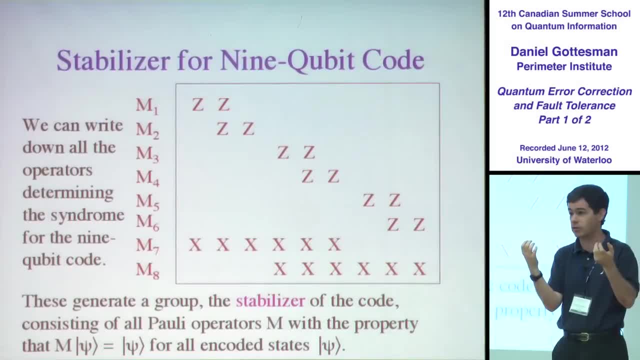 They could also be a plus one eigenvector of Z1, tensor Z3.. But of course that's not something new, because we already knew first, two qubits are the same, second and third qubits are the same. first and third must be the same. 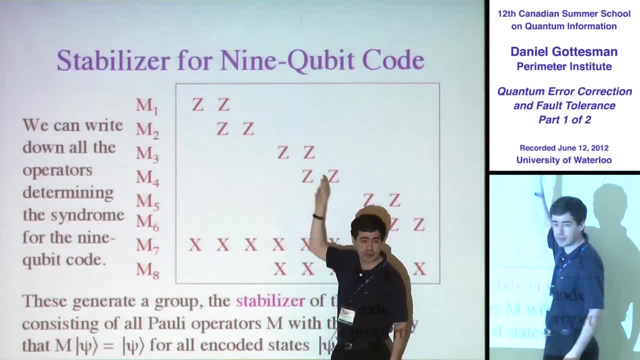 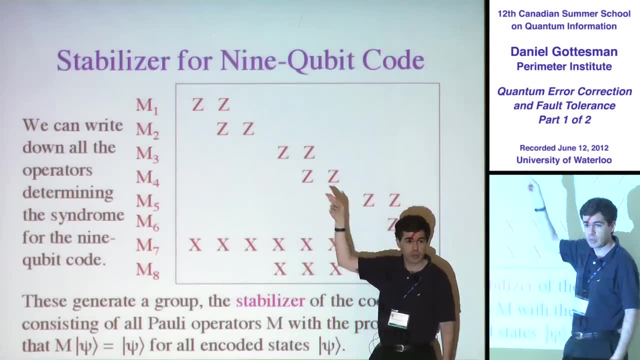 and that's encapsulated by noticing that ZIZ is a product of ZZI and IZZ- the first two lines here Okay, and in fact you can see that has to. in general be true that if you have the product of 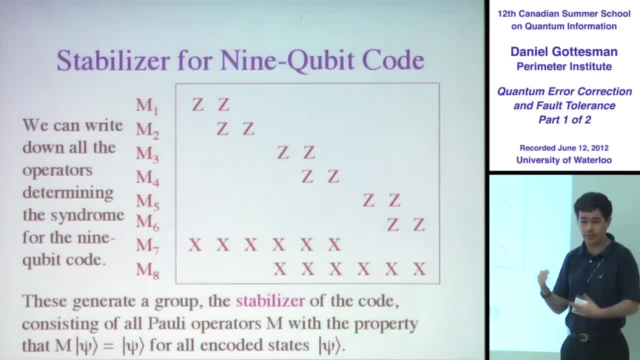 operators where the state has plus one eigenvalue. that's still going to be something with plus one eigenvalue And therefore what we can do is we can define the group called the stabilizer of all poly operators, M, with the property that M psi is equal to psi. 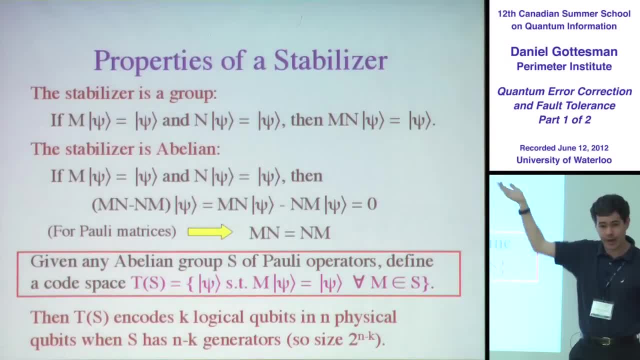 Okay, as I said, it's a group. if we have M psi is equal to psi and N psi is equal to psi, Then M N psi- well, that's going to be equal to M times psi, because N psi is equal to psi and M. 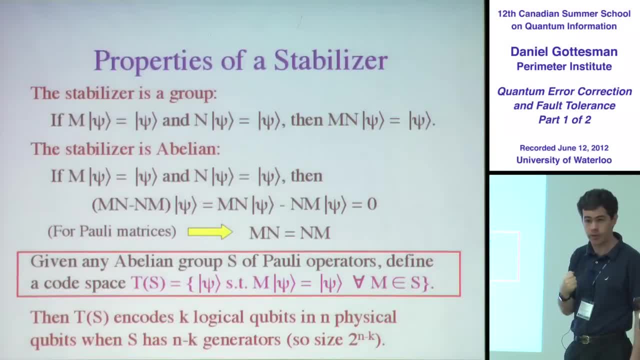 times psi is equal to psi again. So M times N is also in the stabilizer. And the more stringent property of this group is that it's actually an abelian group. Everything in this group commutes Poly operators. in general they can commute or anti-commute, but for stabilizer they have to commute. Why is that? 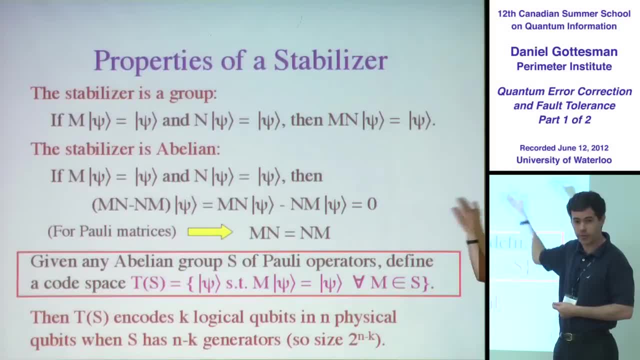 Well, suppose we have M and N in the stabilizer. So M psi is equal to psi and N psi is equal to psi. Then M N psi is equal to psi and M psi is also equal to psi, And so the difference M N psi minus N M psi is equal to zero. 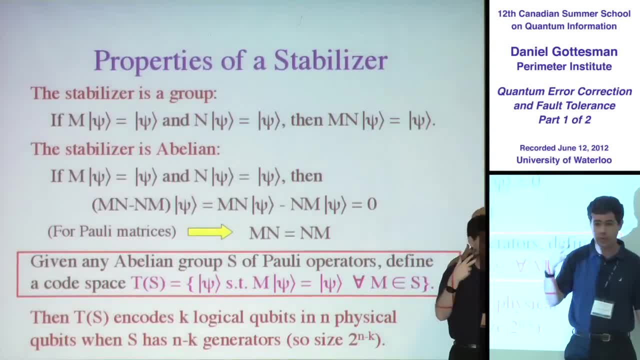 Okay, so the commutator M with N annihilates psi. Now, polymachines either commute or anti-commute. If they anti-commute, we're going to get something that has no zero eigenvalues, And so that means that M and N have to commute. 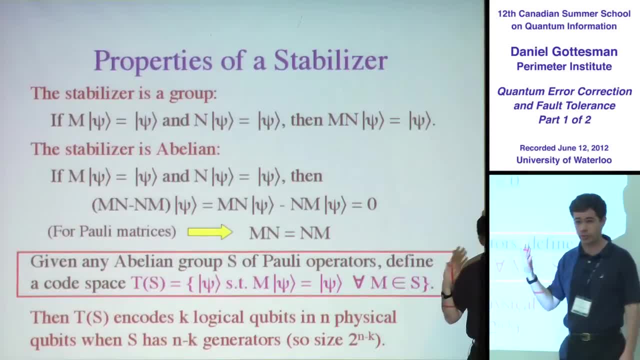 Okay, so the, the stabilizer, is always going to be an abelian group. This makes sense, right? You're used to thinking. if you're a physicist, you've taken undergraduate quantum mechanics and they? they pointed out that you know commuting operators have simultaneous 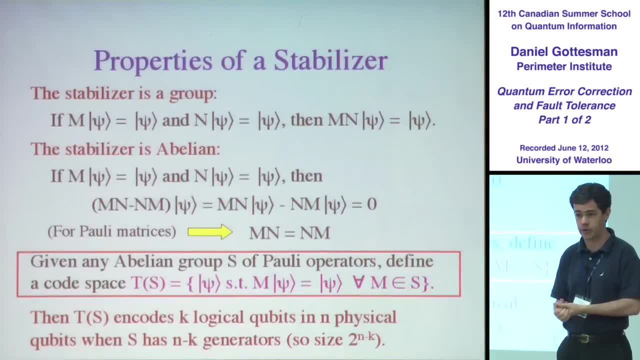 eigenvectors, Non-commuting operators don't necessarily. Okay, and that's just what's going on here. You want a set of operators that all have plus one eigenvalue for all the components. So you want a set of operators that all have plus one eigenvalue for all the components. 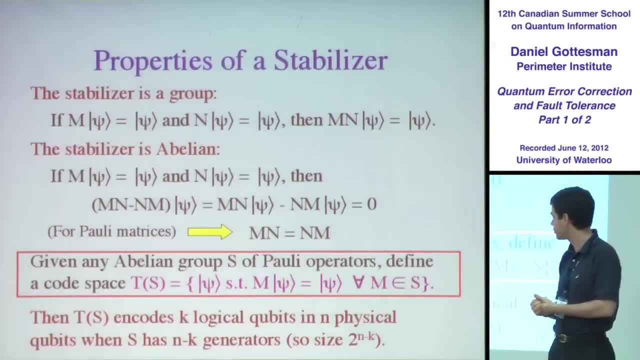 So you want a set of operators that all have plus one eigenvalue for all the components. So you want a set of operators that all have plus one eigenvalue for all the components. Okay, so for the non-qubit code, I wrote down vectors and based on that I deduced a stabilizer. 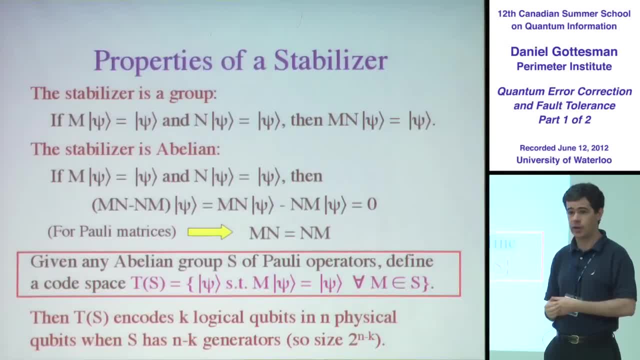 And you can do that in general. but actually it turns out it's more convenient in a lot of cases to go the other way, To come up with a stabilizer group and from that deduce a code. So suppose we have an abelian group of polys. 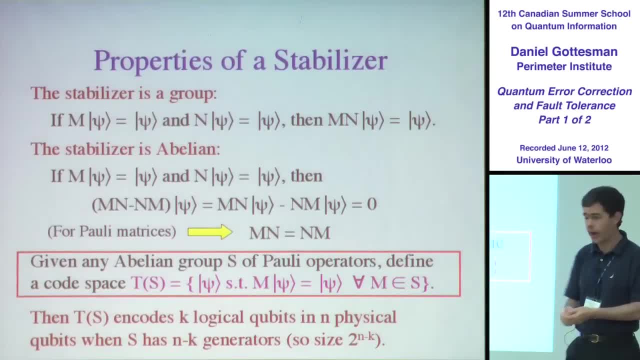 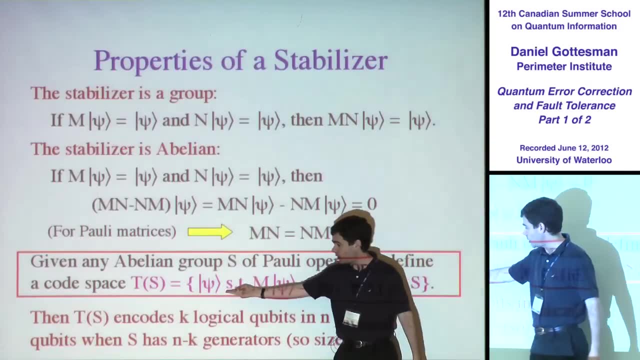 so some subgroup of the polygraph, So some subgroup of the polygraph, And let's insist that it doesn't have minus one in it, because I wanted to find the code space to be the set of vectors, psi, such that m psi is equal to psi for all m in the stabilizer. 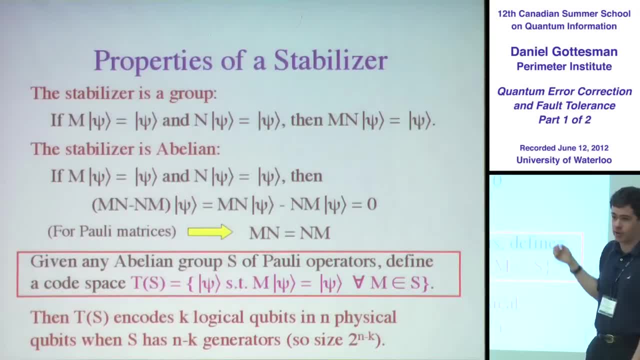 Obviously, if minus one were in this code then there would be no plus one eigenvectors. But in general that's how we wanted to find the code to be the simultaneous eigenspace plus one eigenspace of everything in the stabilizer. 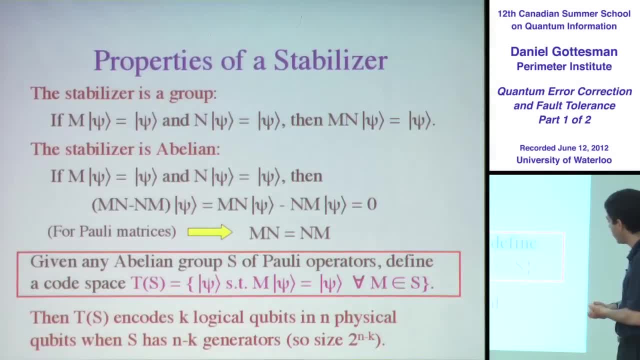 But in general, that's how we wanted to find the code to be the simultaneous eigenspace plus one eigenspace of everything in the stabilizer. OK, And it turns out that if you do this, the- So remember- a poly is a square to the identity. 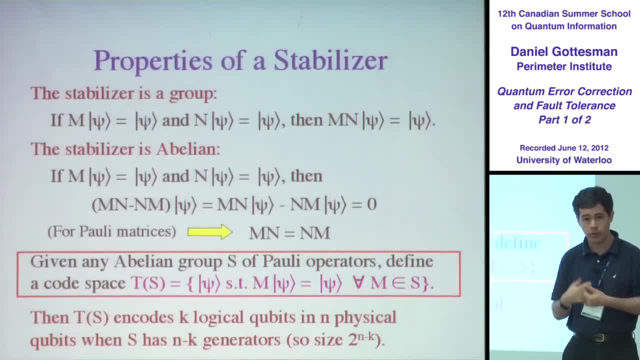 and in the stabilizer everything commutes with each other. so suppose you have a list of operators, of independent operators that are in the stabilizer. well then, the product of those things would be the stabilizer, but squares would just be the identity again. 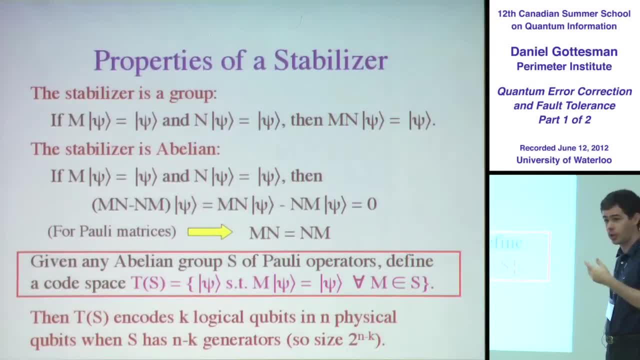 So to get an arbitrary element of thecios for each of the properties Stabilizer, you should take products of any subset of the Generators, not Repeating Generators. okay, so if you have our generators, you have two to the r elements in the stabilizer and 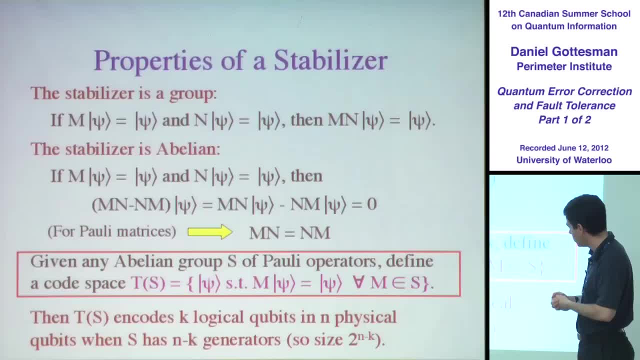 in general. if You're, you have a stabilizer code that has Our generators and n physical qubits. it turns out that it will have K equal n minus r logical qubits. Okay, I guess what I've written here is the other way around: you have k logical qubits and physical qubits. the stabilizer has n minus. 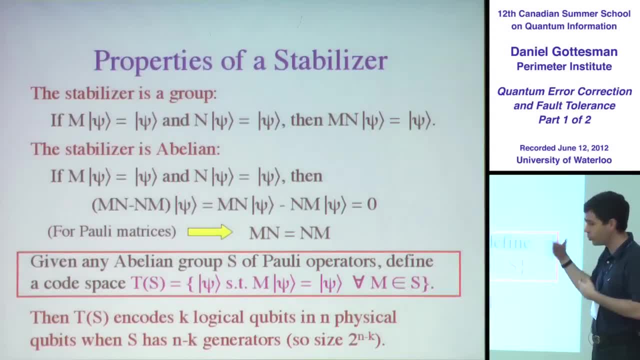 K Generators. Okay, so intuitively you can. you can understand this in the following way: each generator splits the Hilbert space into plus one eigenspace. in a minus one eigenspace, each of each subspace is half the size of the whole Hilbert space. 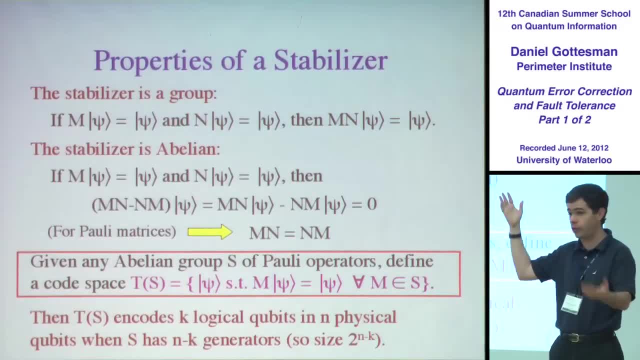 So if you started with n physical qubits, That's a two to the n dimensional Hilbert space. you put one generator and say I want the plus one eigenspace of that generator. Well, that's a two to the n minus one dimensional Hilbert space. 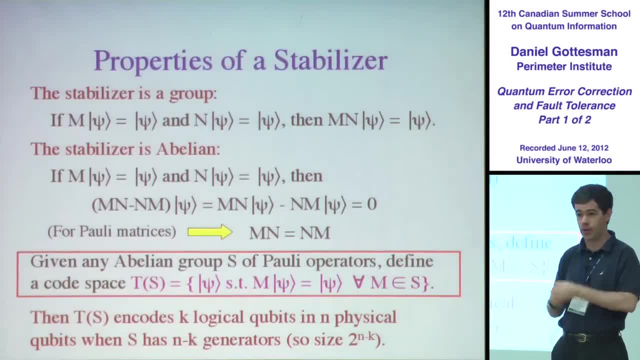 Then you take a second generator, it splits the the subspace in half again, And so the simultaneous plus one eigenspace is two to the n minus two dimensional. and each generator you adds puts it in half again, And so if you add Our generators then you're down to two to the n minus r. 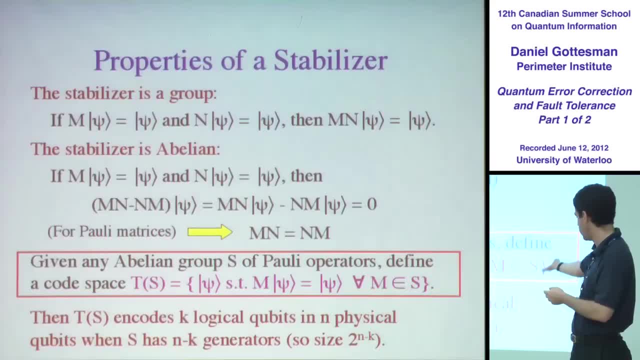 dimensional subspace, Which you know is, is compatible with it. Now, I could say that that is a lot of proof, because you need to show that each generator, your add, is Splitting not just the whole Hilbert space in half, but also the, the, the current. 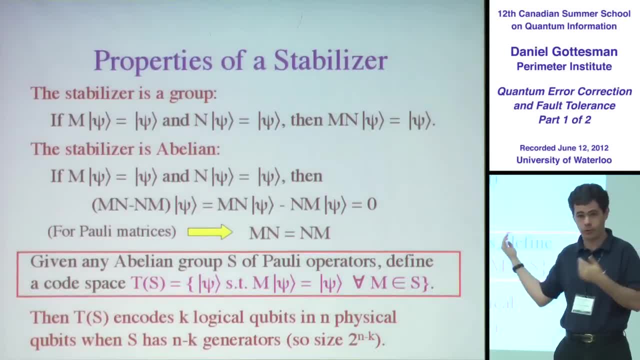 eigenspace in half. That for polys. that happens to be true. So this is right, but that does require some additional proof. Okay so? So this is kind of the basic properties of stabilizer. given a stabilizer, We can come up with a subspace. You know how big that Hilbert space is? 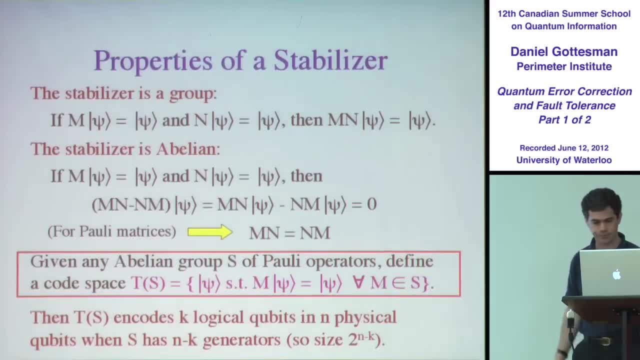 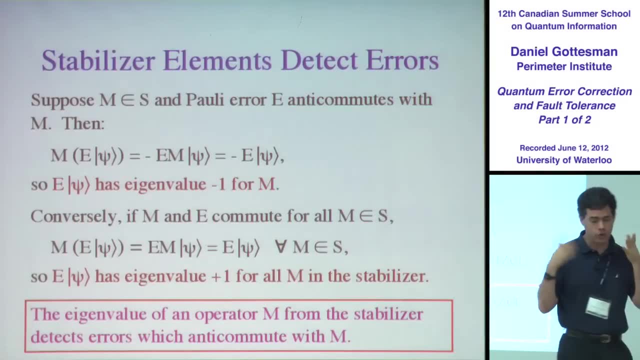 But what we really like to know is: is it good at correcting errors? Okay so. so how does the stabilizer tell us about errors? Well, it should tell us something right in the nine qubit code. we came up with the stabilizer by thinking about what operators we had to measure it to find the error syndrome and 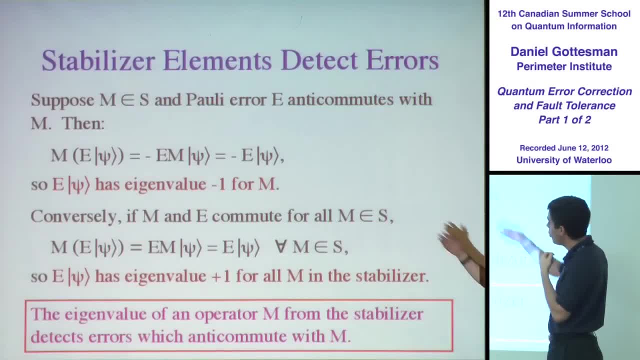 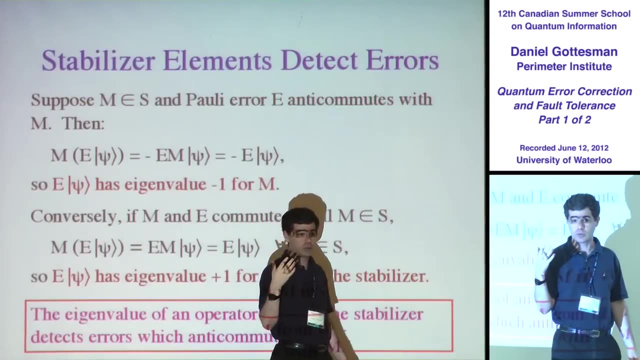 That's something that that's true very generally. So suppose we have some some M in the stabilizer and We have some error e that anti commutes with M. Well, Let's see how the I get with the I. what happens to the eigenvalue of e psi for M? 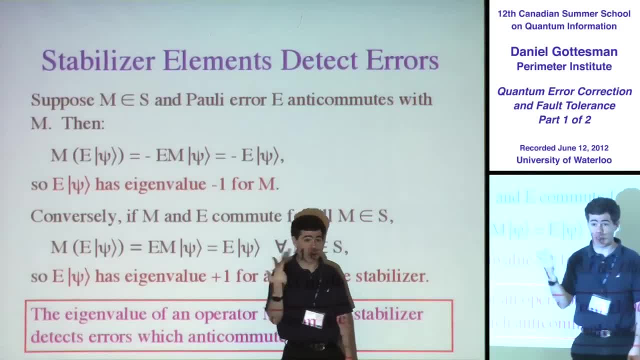 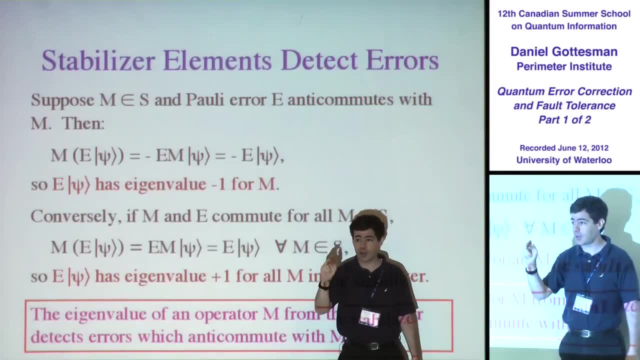 So M e psi? Well, that's equal to minus e M size, since e and M anti commute and M size equal to size. So this is equal to minus e psi. So e psi is now a minus one eigenvector of M, Whereas psi was a plus one eigenvector. 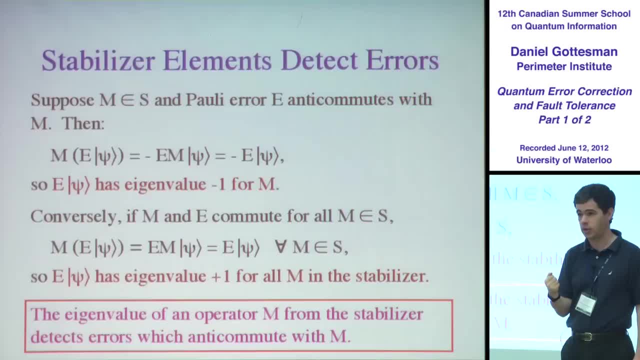 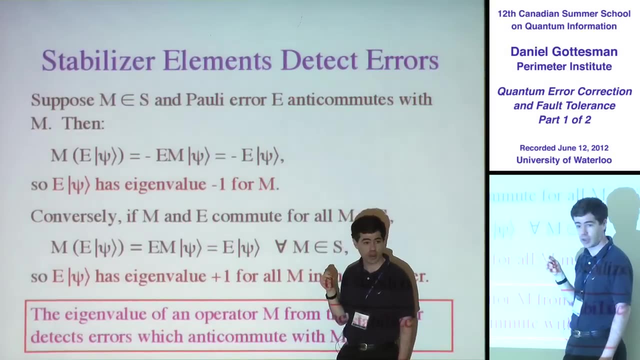 So having the error e, which anti commutes with M, Changes us from plus one eigenvector of M to a minus one eigenvector of M. Firstly, if M and e commute, Then M e psi is equal to plus e M psi, which is equal to e psi. So e psi remains a plus one eigenvector. 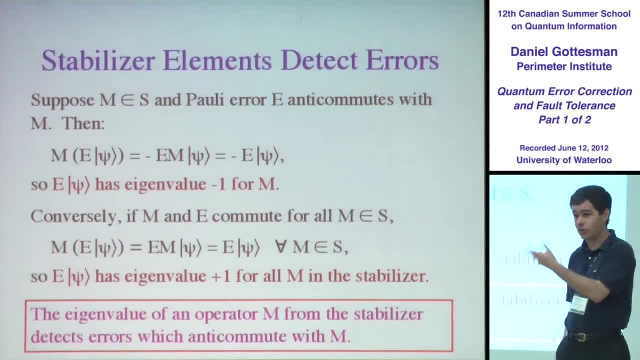 Okay, So what this means is that if we have an error e, Then you look at. you look at each element of the stabilizer M and if e commutes with M, Then the eigenvalue of M stays plus one. if e anti commutes with M and the eigenvalue changes to minus one. 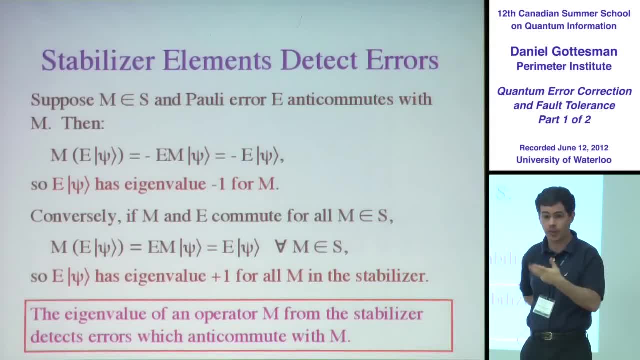 Okay, so this tells us. this is telling us something about what errors are occurring if we look at the eigenvalues of the Generators of the stabilizer, and that'll tell us a lot of information about the errors if we pick the generator as well. um, okay so. 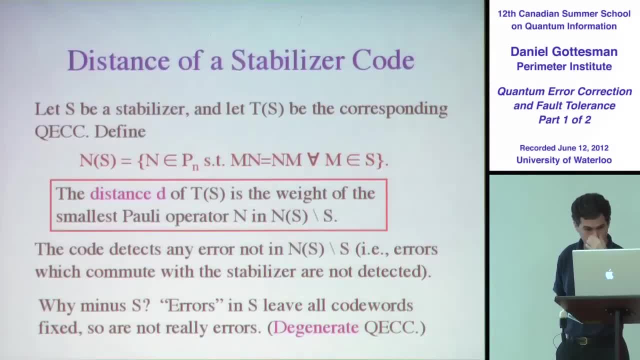 in particular, Let's define a set n of s, which is a set of all poly operators which commute with everything in the stabilizer. So if one of these errors occurs, our stabilizer code will not be able to detect it at all. Right, because if we measure the eigenvalues of all, all the generators of stabilizer, 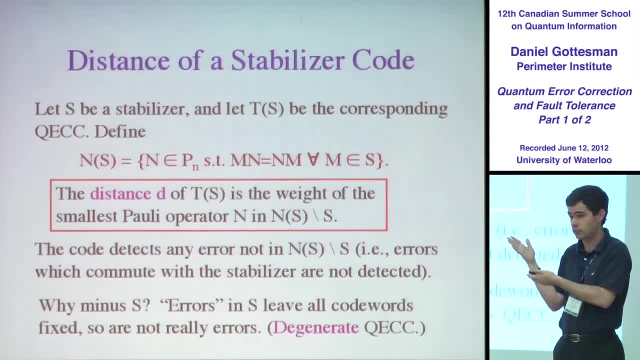 They're all still plus one because the error commuted with it Okay, and the correct code words had eigenvalues plus one. so you know, there's no way we can tell that anything has happened and In fact, elements of stabilizer will map code words to code words. 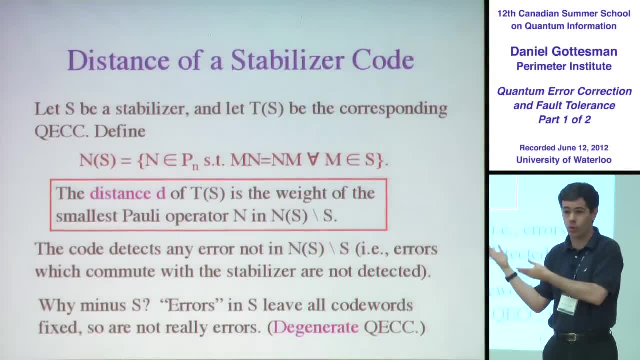 So it's not just that we're not measuring the right things, It's actually there's no way to tell, because the states that we get at the end are valid code words. They just might not be the ones we started. Okay, so things in n of s are bad. Those are undetectable errors. 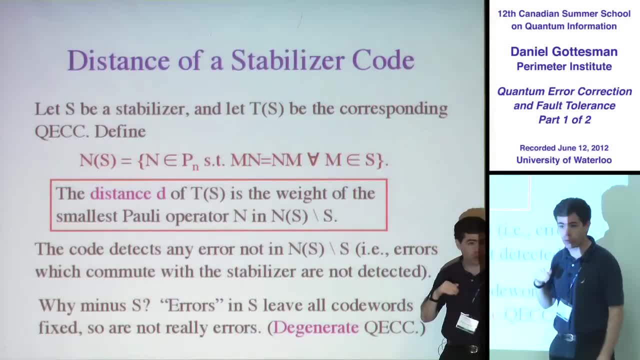 and so, in general, we can Say that the code detects any error that's outside of n of s minus s. So why is that? well, if it's outside n of s, that means that it anti commutes with some element of the stabilizer. And if it anti commutes with some elements of stabilizer, then we'll see that when we measure the eigenvalues. 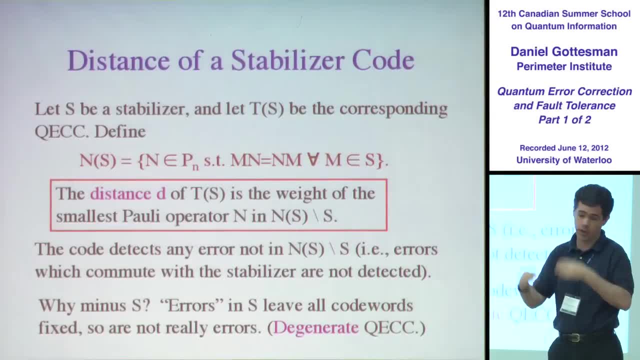 Okay, we'll see that an error has occurred because the- if it anti- commutes with M, the eigenvalue of M will have become minus one. So that tells us there's an error, but Y minus s. so what happens if we have an error? that's in s. 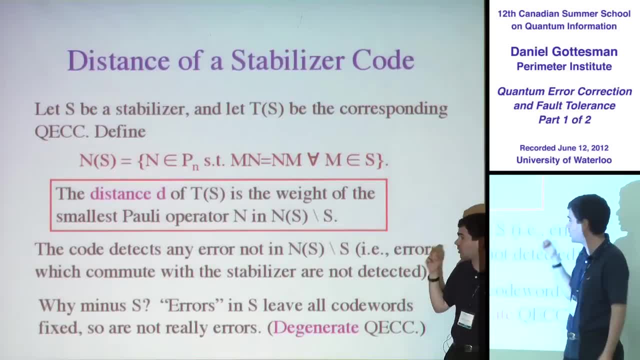 Well, we can't detect that in the in one sense, because the all the eigenvalues will still be plus one. But if it's in s, remember the defining property of s is that it leaves the code words unchanged. So if you have an error in s, that occurs on the state. 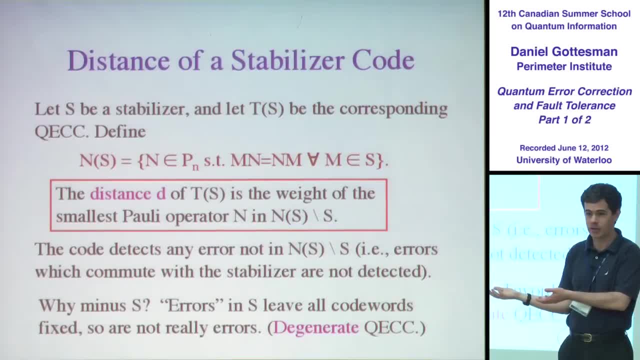 Well, the state psi is still psi. It's not really an error at all. It's just acting like the identity on the code words. So things outside n of s can be easily detected by seeing that they're there. They're no longer plus one. eigenvectors and things in s are not errors. 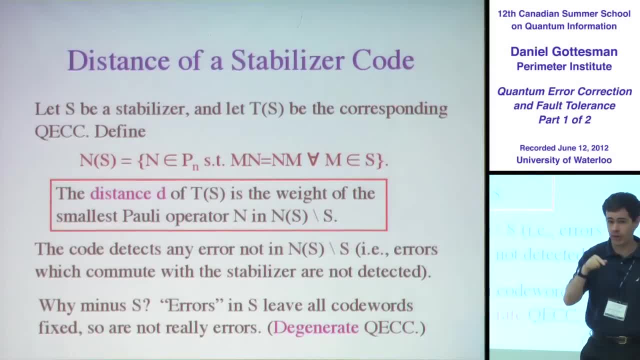 But things in n of s minus s, those are bad. those are things that we can't detect, because they map code words to code words, but they map some code word to a different code word, and That would be a large problem. That's an empirical error. Anything outside n of s minus s, though, is fine. those are the errors we can correct. 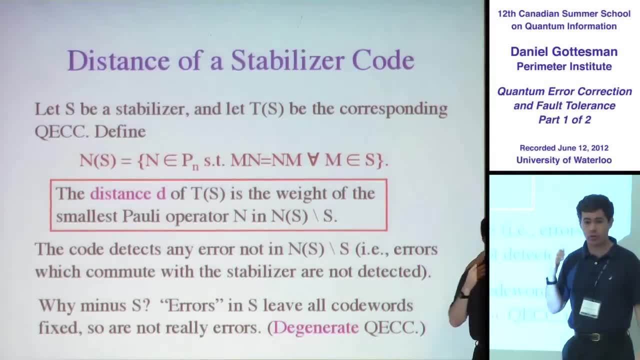 okay, so based on that, we define the distance of a code of This form anyway to be the weight of the smallest poly operator, That's in n of s minus s. so the distance is the, the, the the size of the smallest undetectable error. okay, and intuitively that means that it's the number of qubits you have to. 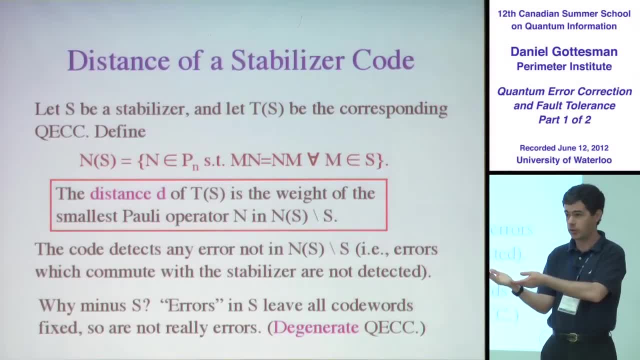 talk to map one code word to a different code word. it's a distance between those two code words. okay, so this, this property of having to deal with the minus s and the possibility of errors that act like the identity, that's something that's unique to quantum codes. there's no real analog in theory of 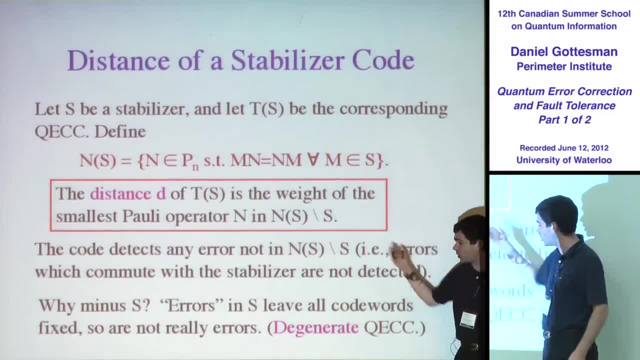 classical error correcting codes, and so code where you're invoking this property is called the degenerate code, and actually you already saw an example of that. the nine qubit code is an example of a degenerate code because z tensor Z, acting on the first two qubits is, as I invite, a plus one, and that means: 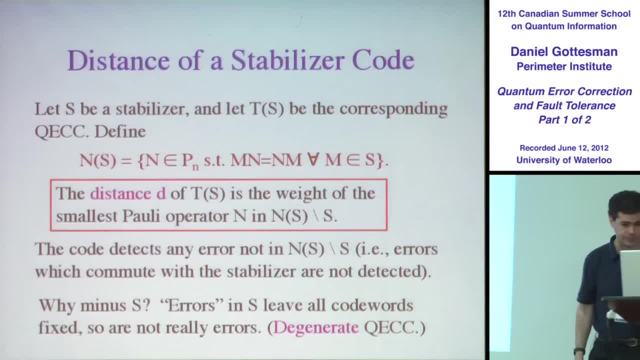 that so well, okay, let me let me get back to that in a minute, actually, okay, so just to finish. so so far I only talked about the technique and I don't want to go into too much detail about it. but I want to talk about the technique and I don't want to go into too much detail about it, but I 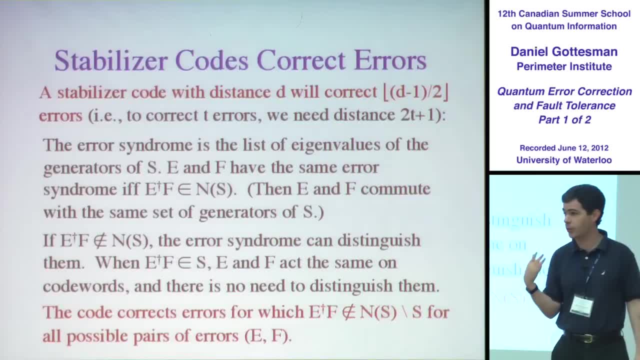 but of course, what we really want to do is correct errors. so how does the stabilizer code correct errors? well, we have to detect errors. we just have to see that one of the eigenvalues of the generators has changed from plus one to minus one. to correct errors, we actually want to identify what error occurred. 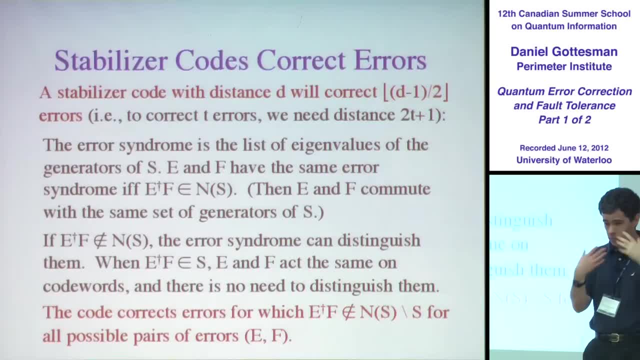 okay, and the way we can do that is by looking at all the eigenvalues and noticing that they can be. they can be different for different errors. so, for instance, an error that commutes with the first operator, first generator, but not the second one, would have eigenvalues plus. 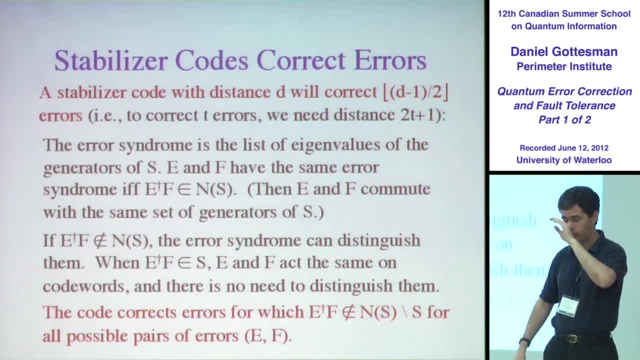 one and minus one for those two. where's one that commuted with the second one and not the first one, would have eigenvalues: minus one plus one. okay, so those two would have different error syndromes and the error syndrome would therefore allow us to distinguish those two errors and, in general, if you think, 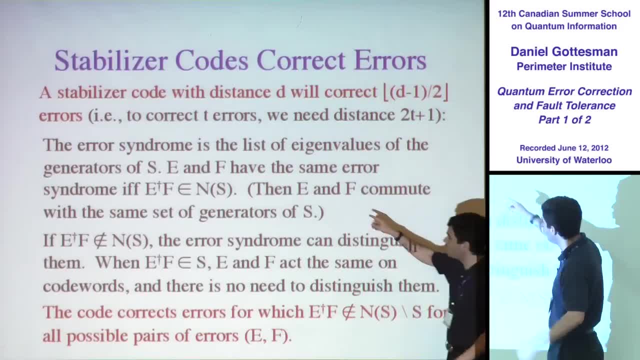 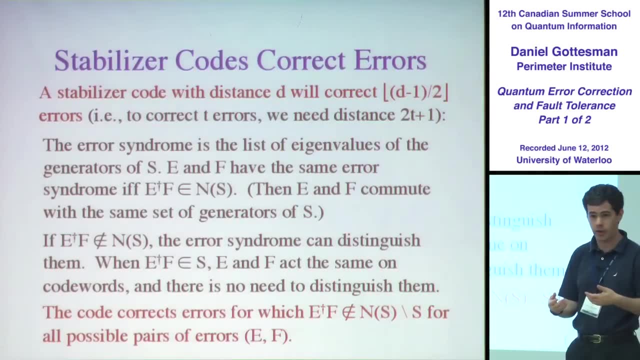 about it. you can see that two poly operators, E and F, are the errors that are the same error syndrome if, and only if, they commute with the same set of generators. and they, if they commute with the same set of generators, then E dagger F is in the N of S. it commutes with everything in the stabilizer. okay, so 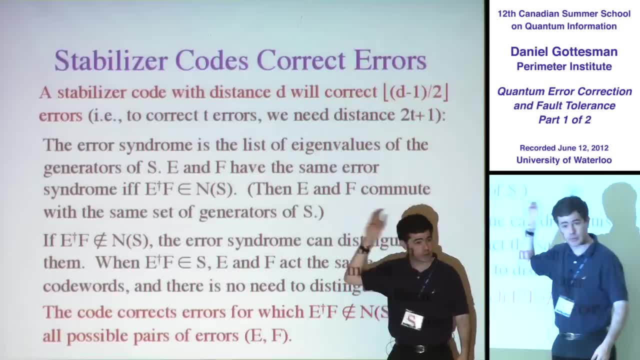 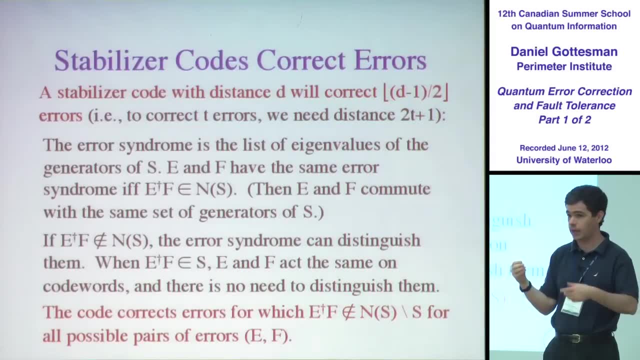 having the same error syndrome is equivalent to saying E dagger F is in N of S. so if E dagger F is not in N of S, that means there's. we can distinguish these two errors by error syndrome and, if that's true, of all pairs of errors. 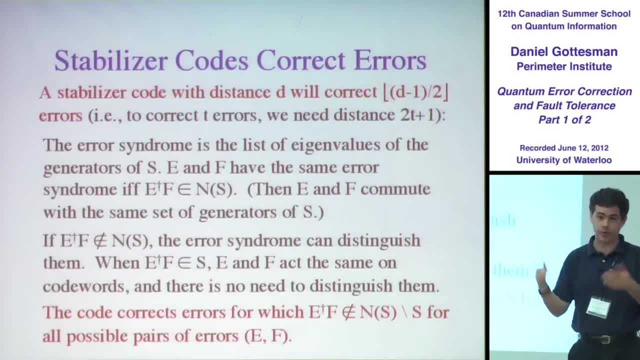 then we can correct errors. if they commute with the same set of generators, then we can correct this set of errors. so, for instance, if the set of errors, set of possible errors, is all errors, all single qubit errors, then this allows us. then then we look at all products of single qubit errors, which will be all. 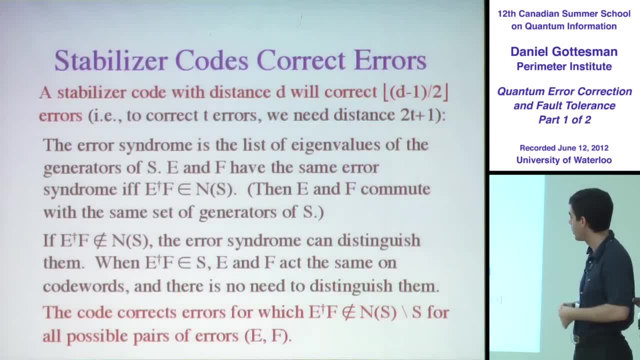 two qubit errors and we can correct those. but there is another possibility, remember, for detecting, for being able to detect the error. we should consider the possibility, the, the- I'm sorry, the undetectable errors, or N of S minus S. so what happens if E dagger F is in in N of S but it's actually in S. so if E? 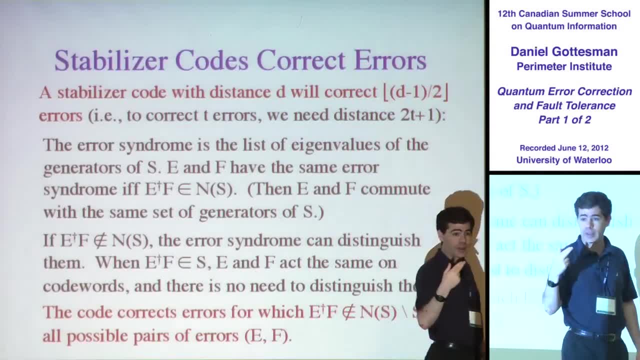 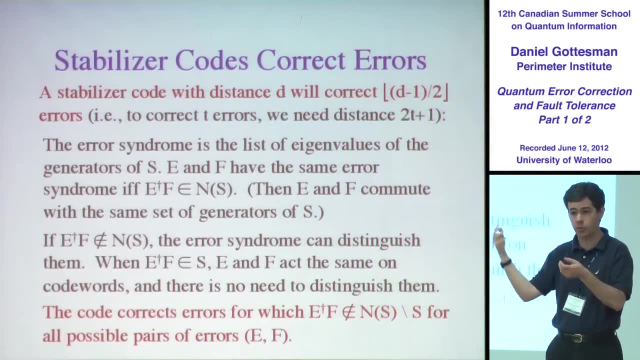 dagger F is in S. well, what does that mean? that means that E dagger F leaves every code word fixed. E dagger F psi is equal to psi, and what that means is that E psi is equal to F psi. so E dagger F in this case is inside N of S. S is always. 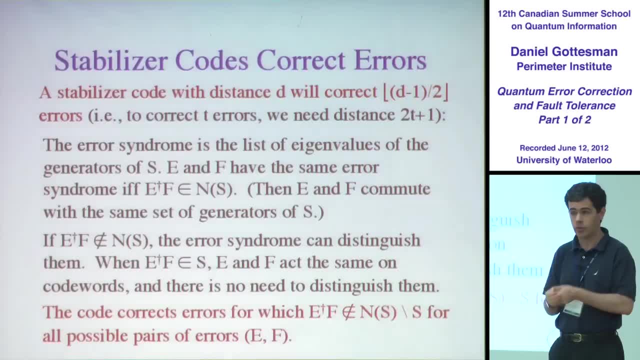 inside N of S. So that means that we can't detect that the error E dagger F occurred. We can't distinguish E and F by their error-synchrony. they have the same error-synchrony, But there's a good reason for that. 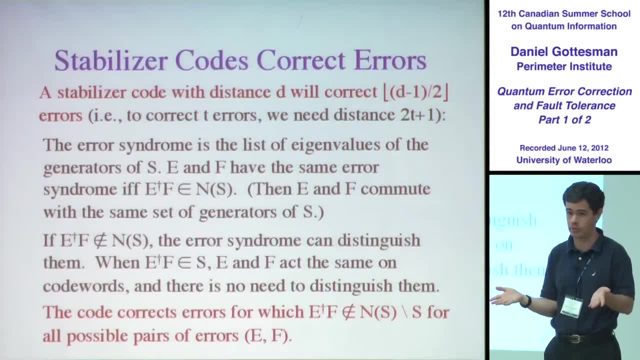 They have the same error-synchrony because they do the same thing to the code words And therefore we don't need to distinguish them. We can just guess which one actually occurred and correct it. And you know they both do the same thing, so correcting one of them corrects the other. 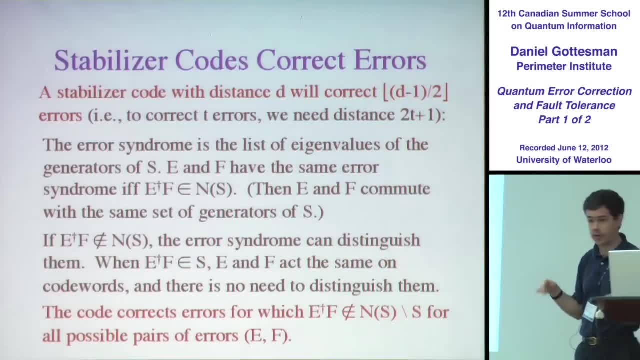 one too, And so that's the sense in which you can see that the nine-qubit code was degenerate, Because if you think of, say, the first set of three, 0, 0, 0,, plus or minus 1, 1, 1,- well, 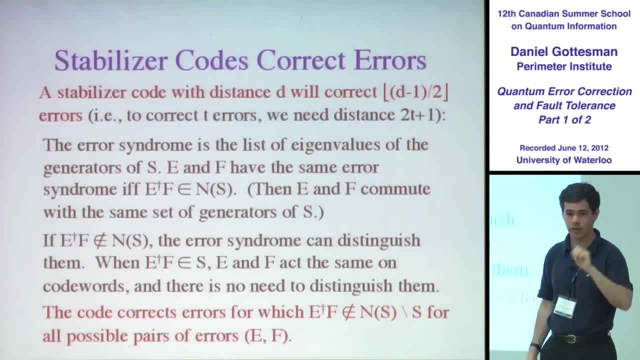 if we have a phase flip on the first qubit, that takes us to 0, 0, 0, plus 1, 1, 1, to 0, 0, 0, minus 1, 1, 1,. if we have a phase flip on the second qubit, it does the same. 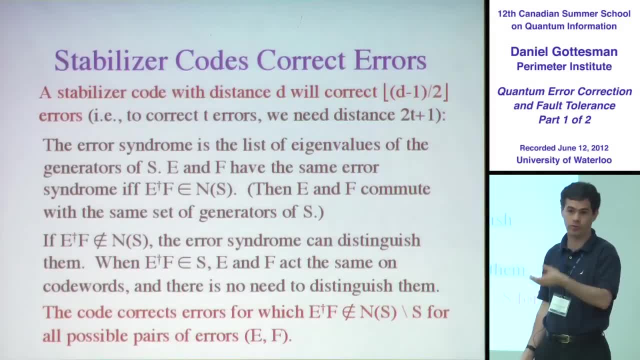 thing. It takes 0, 0, 0, plus 1, 1, 1, 1, 1, to 0, 0, 0, minus 1, 1, 1,. OK. 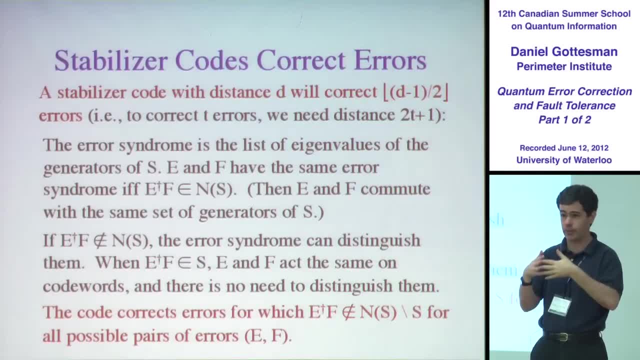 And so that's why it's degenerate, because two different errors do the same thing. So if E dagger F is in S, we don't need to distinguish E and F, and we're also OK. So that's the real condition. 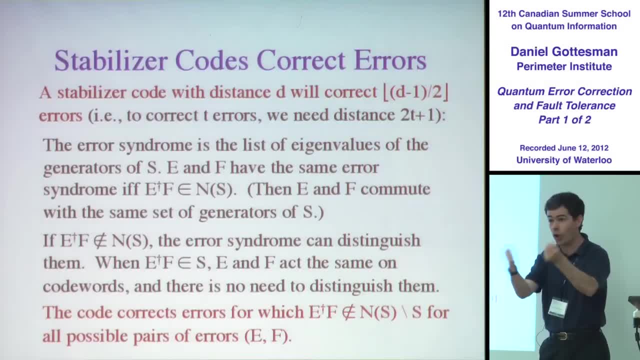 We say a code corrects some set of errors if for all pairs of errors in the set of possible errors, E dagger F is either outside N of S or it's inside S. So that's the condition for a stabilizer code to correct errors. 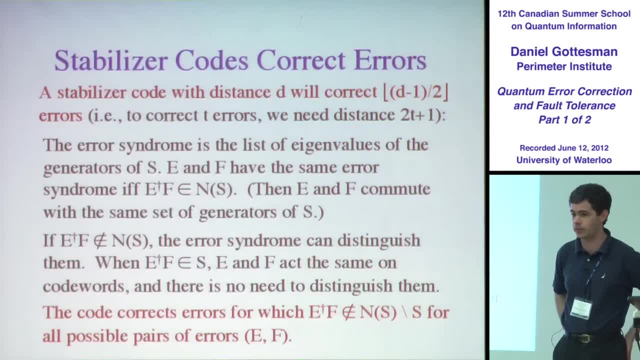 OK, I'll stop there And we'll continue from that point after. That's the last, I guess. 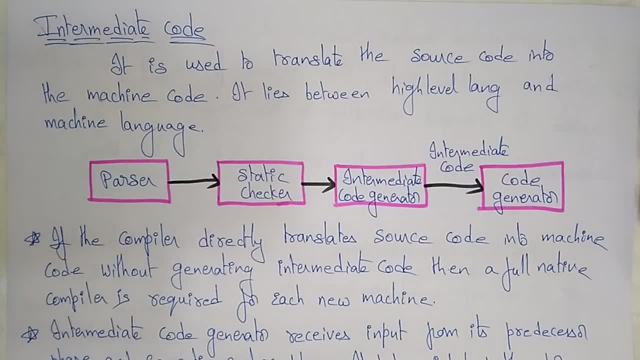 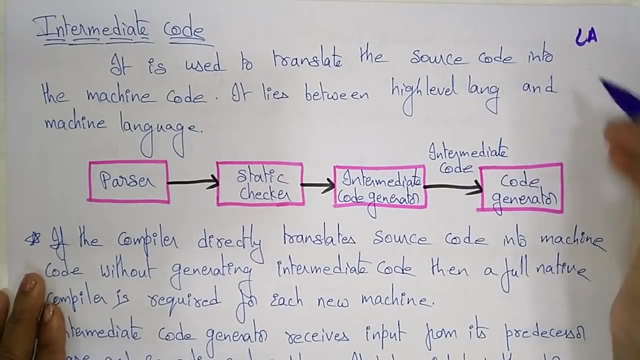 Hi students, welcome back. Coming to the next topic, that is, the intermediate code, Let's see what is this intermediate code. You already know at what stage this intermediate code will be there In the compiler. first you are having the lexical analyzer, next is the syntax analyzer and the semantic analyzer, next is the intermediate code generation.